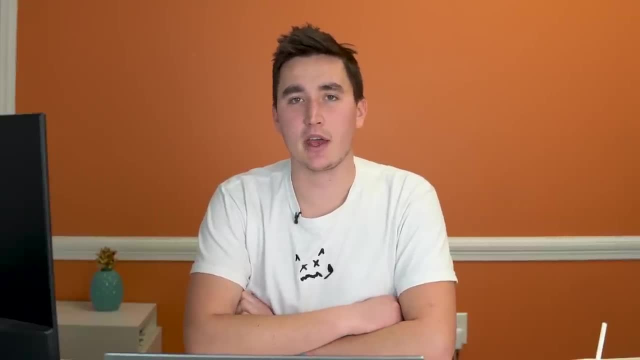 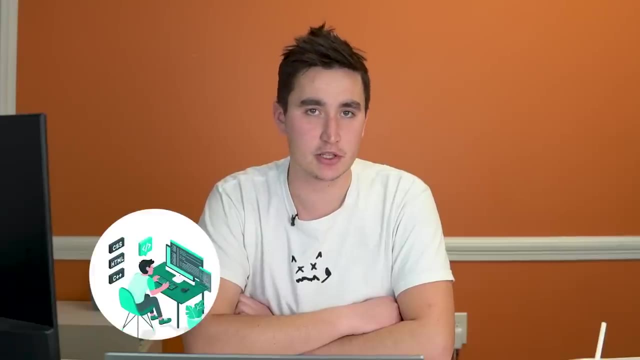 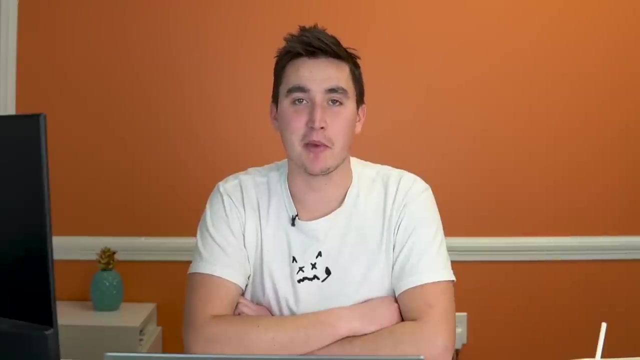 machine learning models. In this video, I will be interviewing Kylie Ying. Kylie is a fellow tech YouTuber who makes content on topics that include programming projects, Python tutorials and lifestyle vlogging. Kylie has both her bachelor's and master's degrees from MIT. 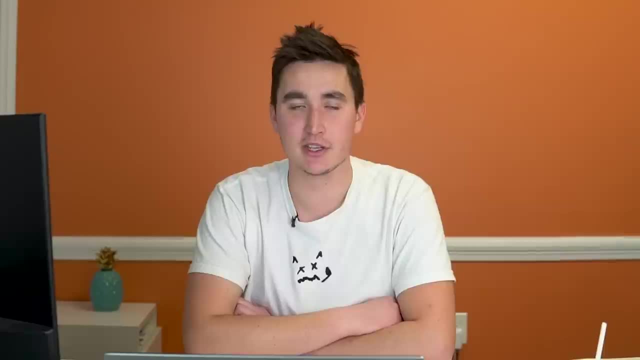 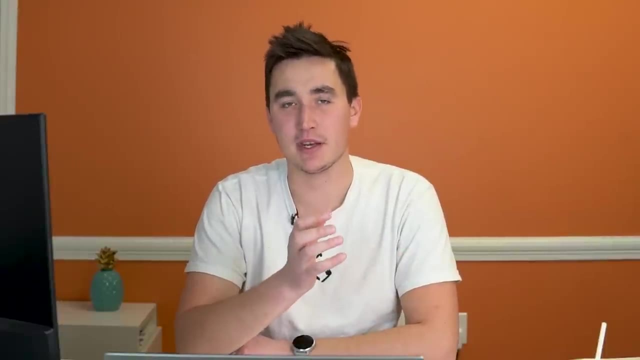 and she has a track record of success in the interview process, receiving offers from top-tier companies such as Meta. The format of the video will be roughly a 45 to 60 minute technical interview, followed by a breakdown of how that interview went. 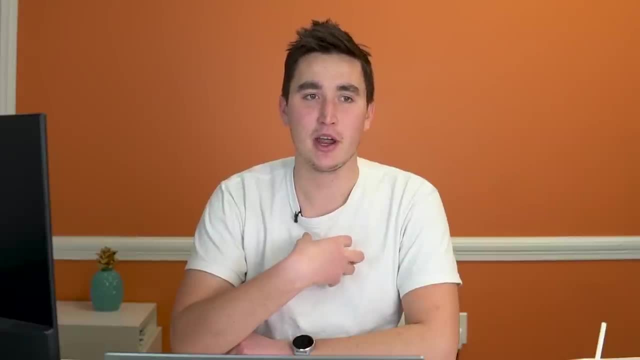 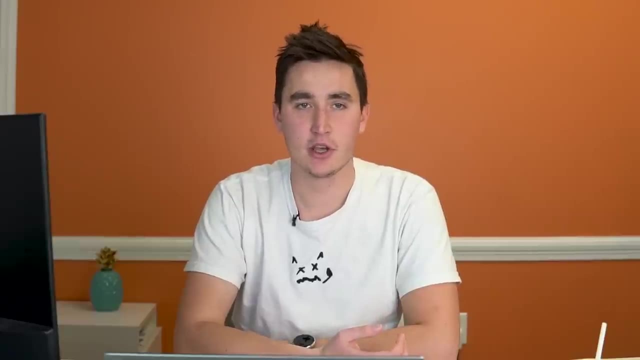 where both Kylie will be giving me feedback as the interviewer, as well as I'll be giving her feedback as their interviewee. Some important context: I have conducted dozens of interviews when I was a part of the founding team of Posh Technologies, From roughly the size of 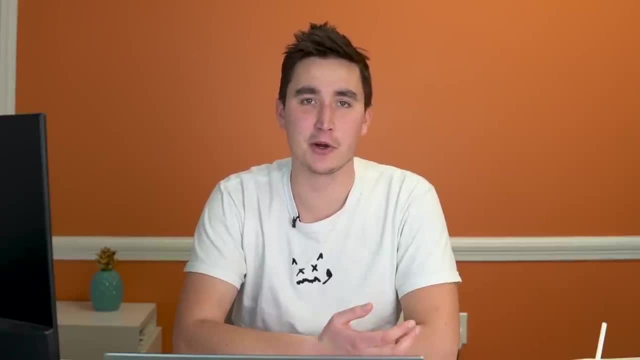 just five people to all the way till we were just under 40 people. I participated in most interviews, so I've seen the good. I've also seen the bad. The questions that we walk through in this video are an adaptation of the style that we used in one of our interviews for data science candidates. 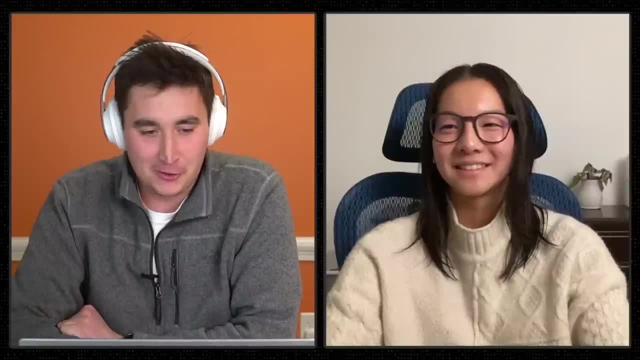 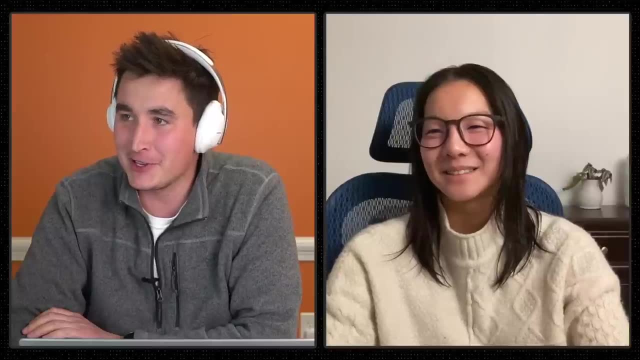 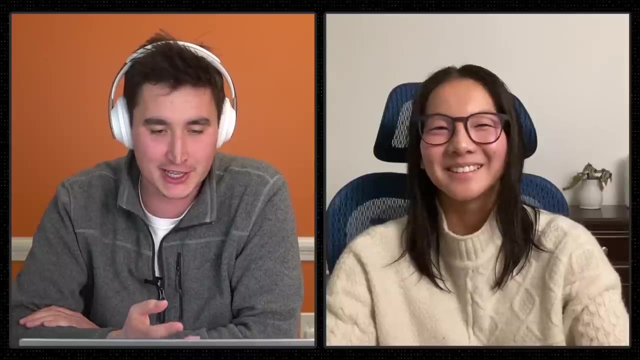 at Posh, so I try to make it as real world as possible. Welcome. how's it going today? It's good. how are you? I'm doing pretty well. Weather's not been too bad, so I can't really tell. Exciting to meet you, exciting that you're interviewing for this team. Great to meet you too. 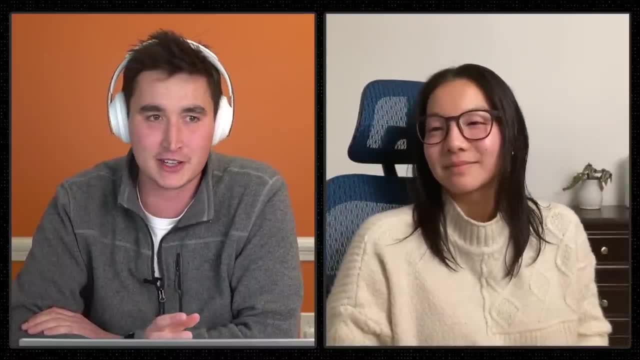 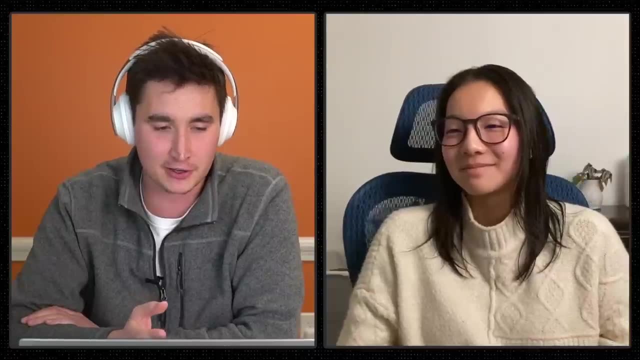 We've been looking for, you know, someone to fill this role for the past, you know, couple weeks and, I know, excited by your resume and just excited to learn more about you and, kind of, you know, walk you through the task that we'll be solving today. So, I guess, to start off, 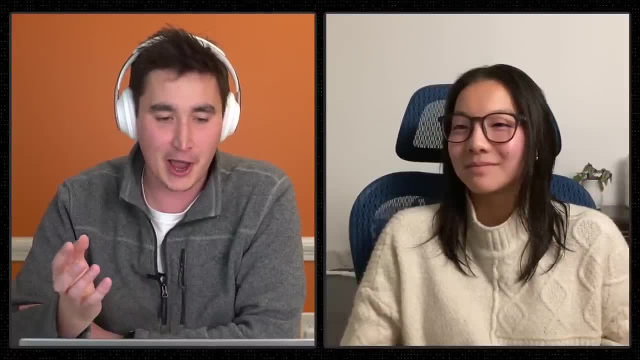 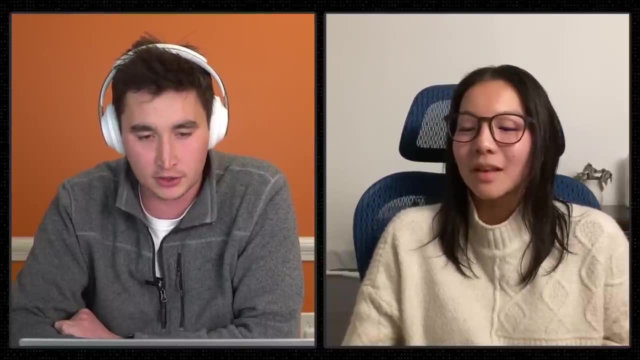 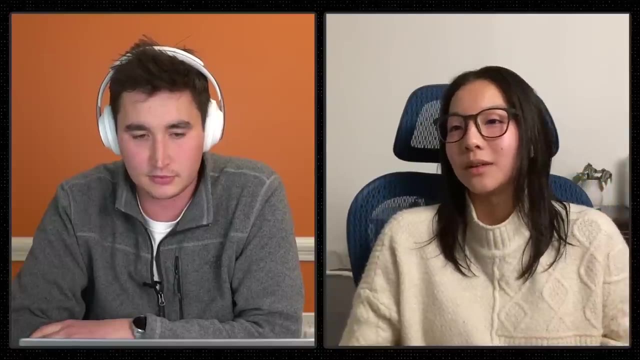 I'm curious. you know I read your resume, but just tell me a little bit more about yourself and, I guess, what you're looking for in your next opportunity, Your next role? Yeah, so I finished my master's and undergrad from MIT. I was doing a lot of. 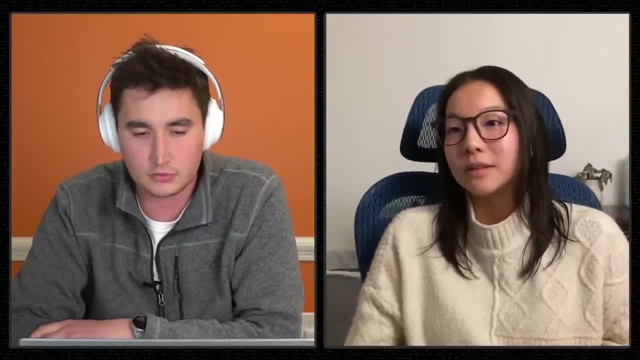 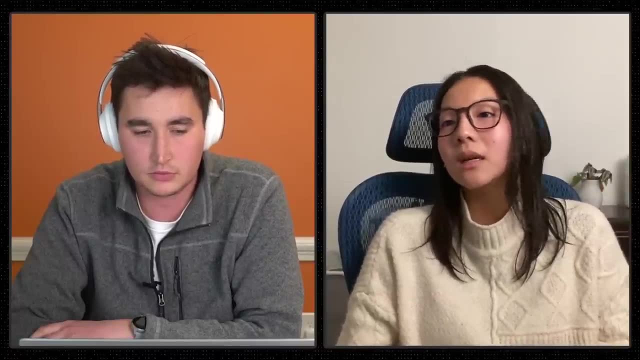 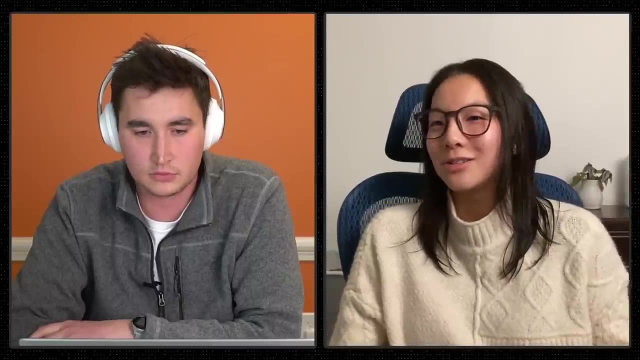 electrical engineering, computer science, along with physics, and in my next role I'm just looking for something more quantitative, something intellectually stimulating and you know, just somewhere I can learn a lot. So I saw this job and I thought I'd apply, because 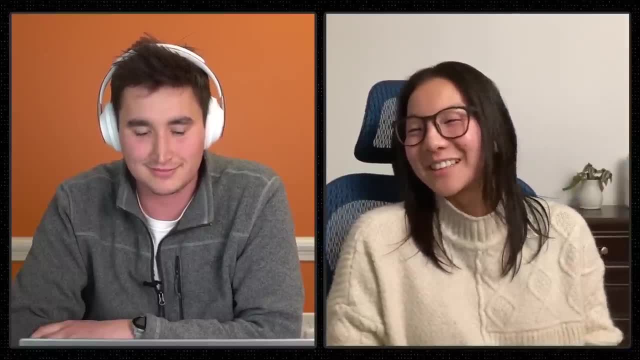 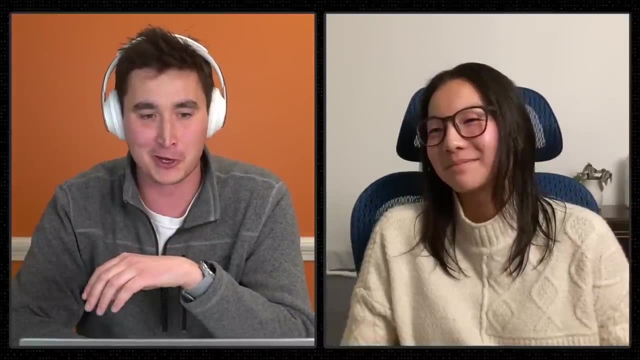 based on the job description, it just sounded like everything that I wanted. you know? Yeah, definitely And honestly, from my experience, like we have a really hard working team. We're working on hard problems, exciting problems, So definitely like. 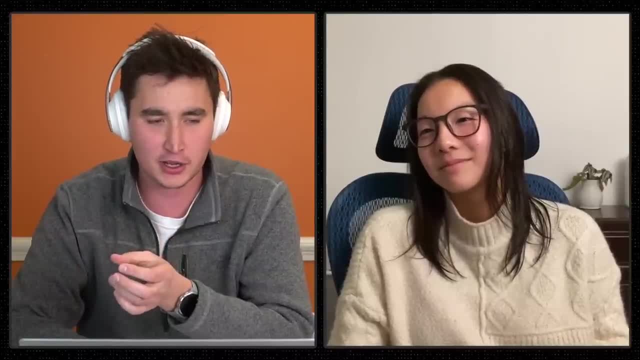 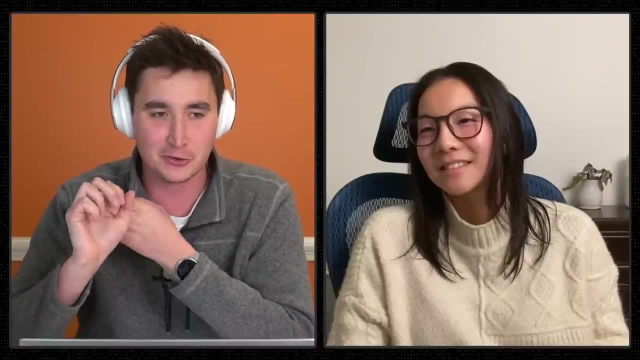 fits that category. I guess, just to break into that a little bit more, like what you just said, a lot of things, computer science, you know, electrical engineering and physics. I guess what made you kind of study all of these things, I guess what excited you about just that? 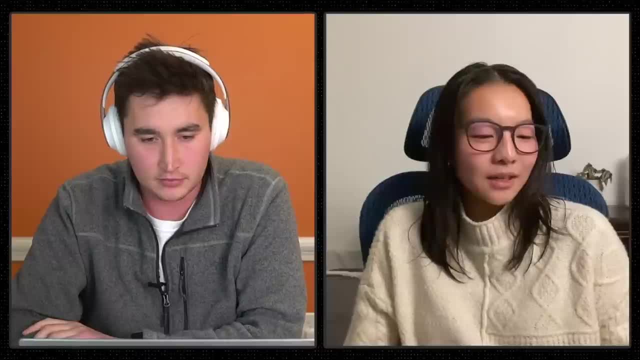 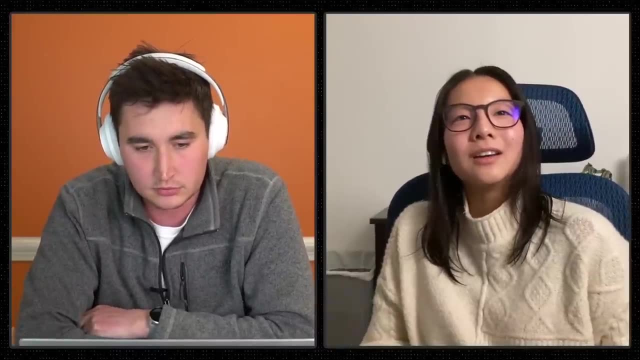 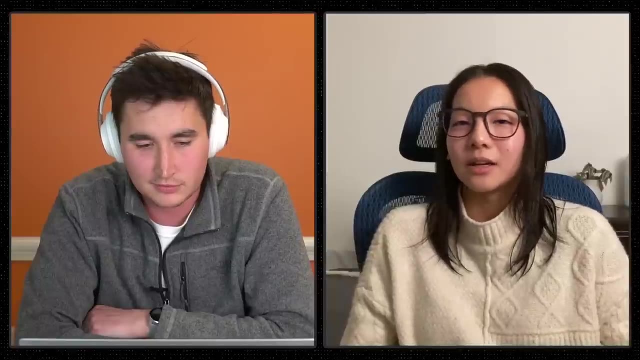 you know, spread, I think with like well, okay. so I really think that with EE and CS it was because I wanted to. I was I had the super like, I was very interested in AI and robotics and I just really wanted to be able to just someday create Jarvis. 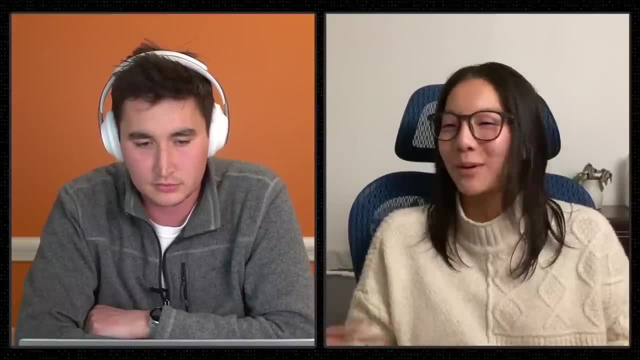 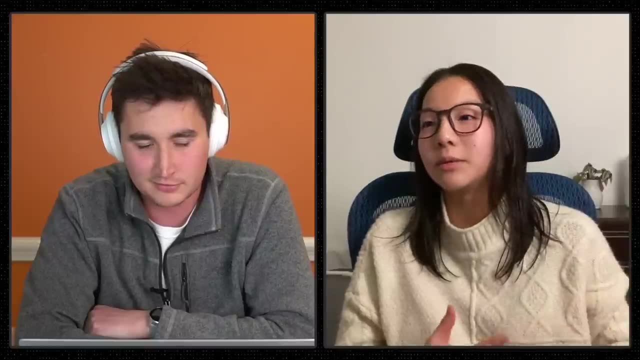 like to have the tools to create Jarvis- And which, by the way, is Tony Stark's superhuman AI. And so I thought, you know, with computer science I would be able to have the programming, the AI part of that, but then, also with EE, I'd be able to literally build the Iron Man suit. 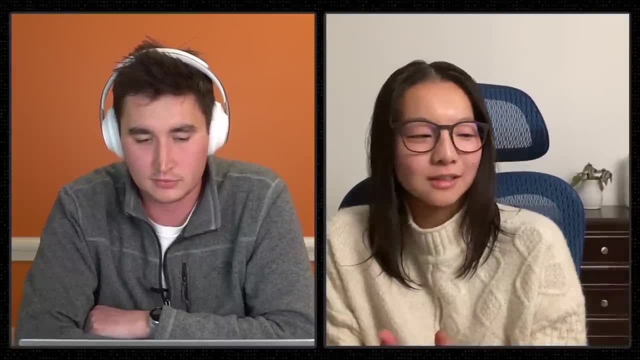 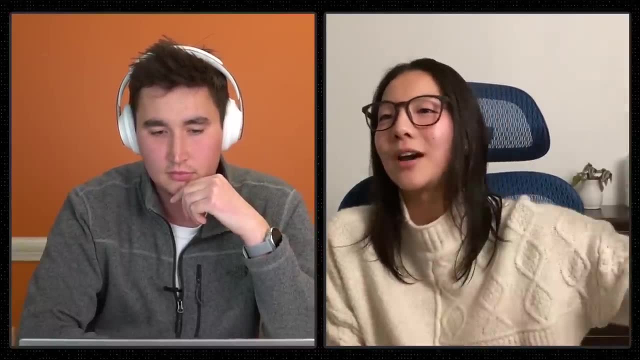 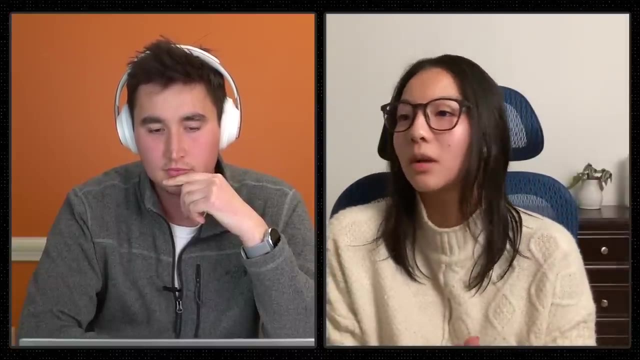 which would be pretty cool. And then with physics, I think it's just. I've always been really curious about the evolution of the universe, like what's out there- black holes, the galaxies, stars, all of that good stuff, And so when I took a relativity course, it just really 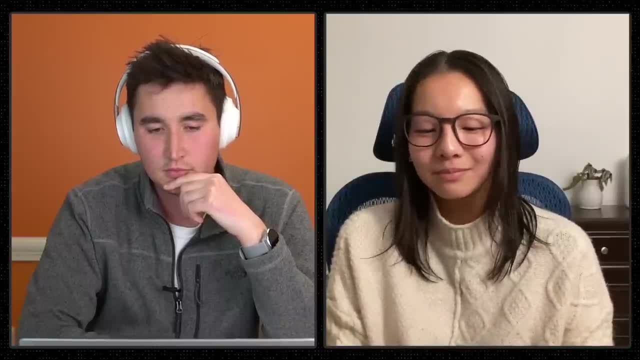 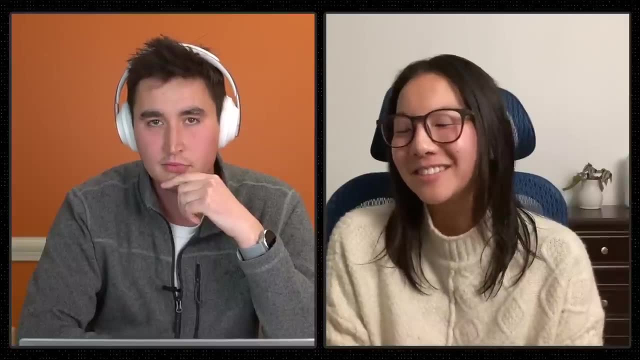 blew my mind that there are all these things that I could do. I think it's really cool, I think it's. there are all these things that I don't- I just you don't even know- that are out there right, Like light bends around stars because of gravity, Like that's so cool. Yeah, no, definitely It's. 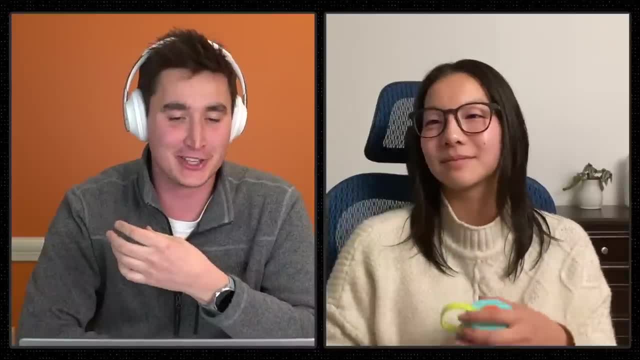 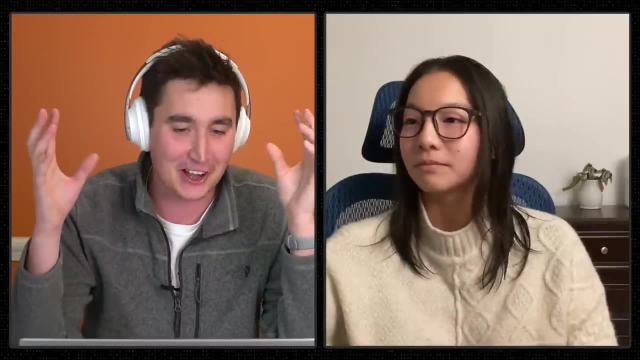 fascinating, Like especially exploring outside of my realm. I don't have that physics experience, I don't have that kind of, you know, space exploration, all of that fun stuff experience, but I am fascinated by it as well. And also fun fact: I'm sure you're aware, but Tony Stark was. 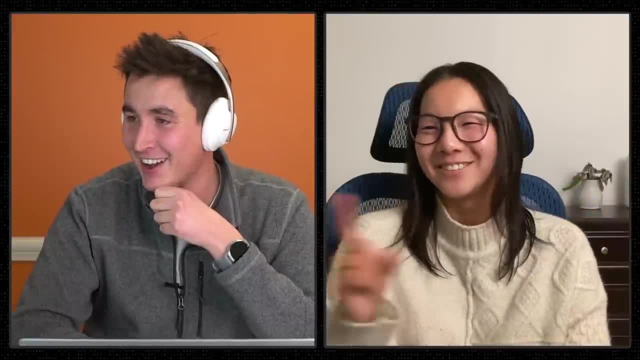 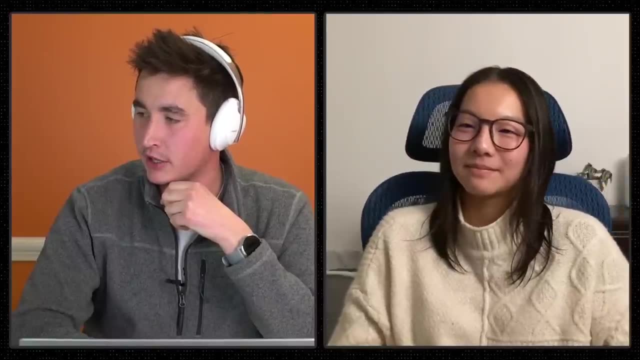 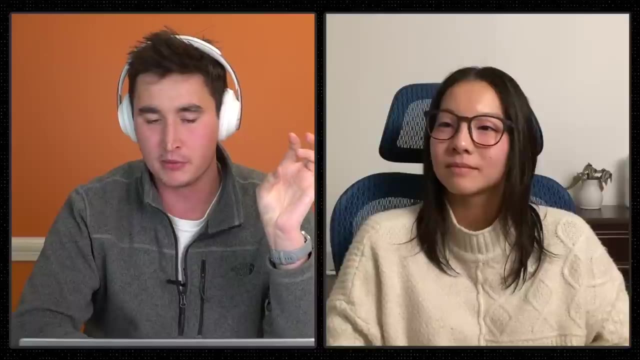 also an MIT grad, so you're in good company there. Why I wanted to go to MIT Smart, Okay. So I guess, before we get into like kind of the real bulk of this interview- I mean I think you kind of hit on it a bit with that, but I'm curious to just dig into this a bit more. So I mean, 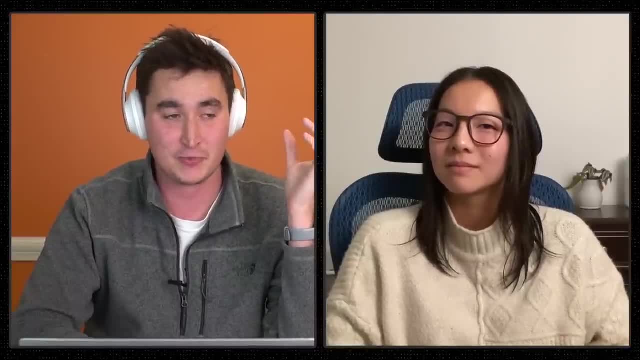 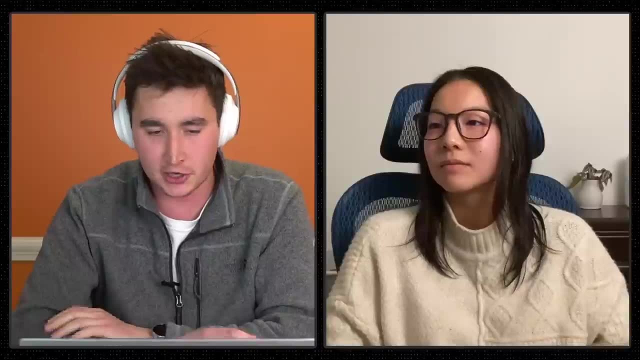 in the past year or two, even just really like past like six months, there's been a ton of developments in the artificial intelligence, machine learning space. I'm just curious if there's anything you want to say about that. Yeah, I mean, I think it's, I think it's, I think. 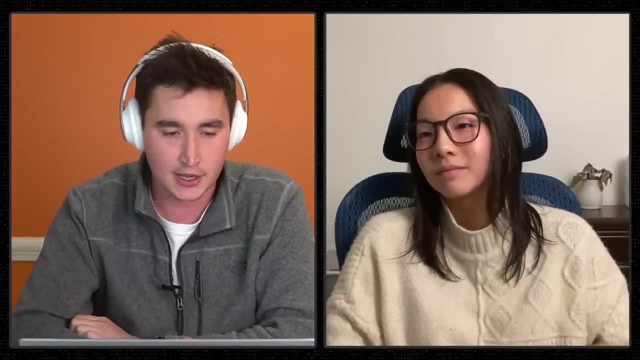 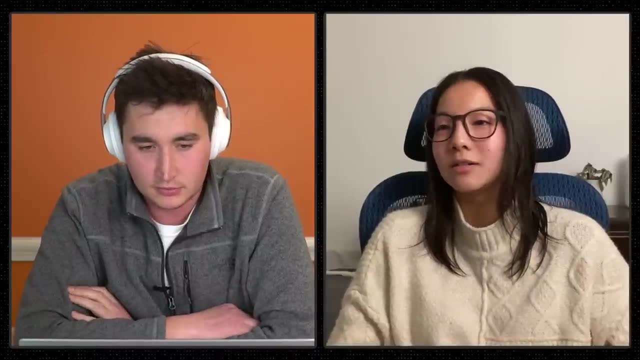 anything that kind of sticks out to you that you're particularly excited about and, if so, like what that is and what excites you about that. Yeah, So I definitely think that what everyone's talking about right now is like chat, GPT- right, Because it's super disruptive. Everybody's like. 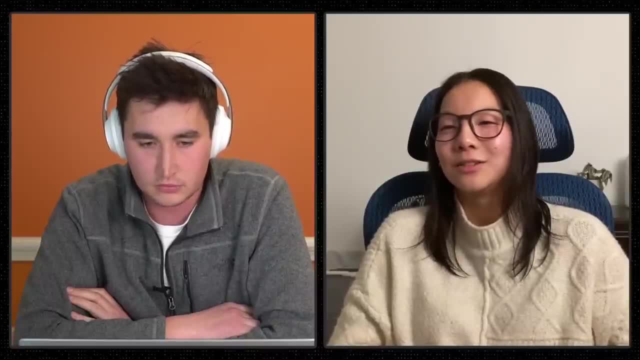 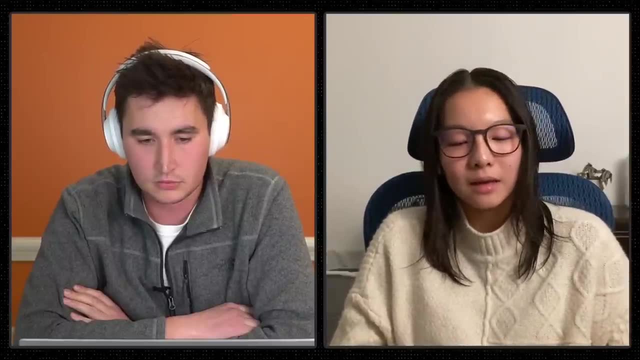 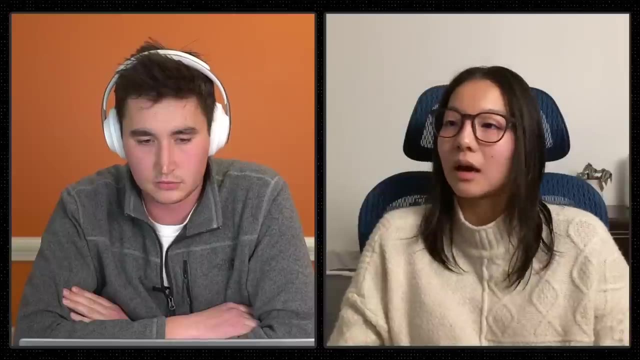 Googling how to write their essays or how to code up this. you know something- script, which is awesome, But I would say that you know this. this AI stuff. I mean I'm super interested. specifically, I think I'm really interested in reinforcement learning and and just getting 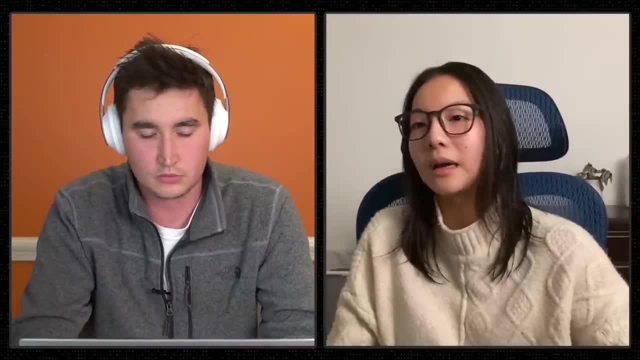 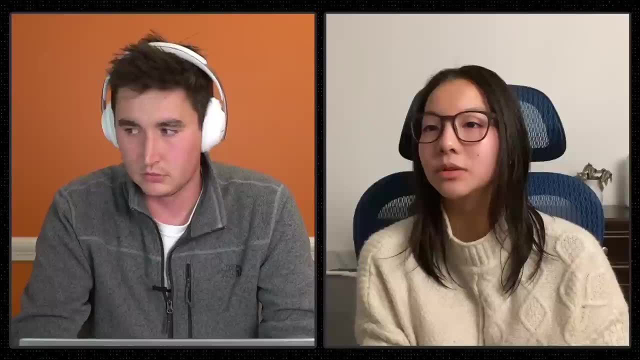 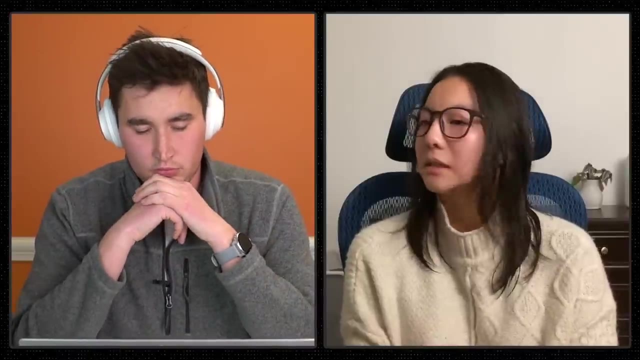 a computer to beat humans at certain things, or robotics in the sense of like self-driving cars. I think that's really interesting: being able to teach a robot how to interact and basically do what a human would do. Also, things like superhuman chess AIs or superhuman poker AIs. I think that's. 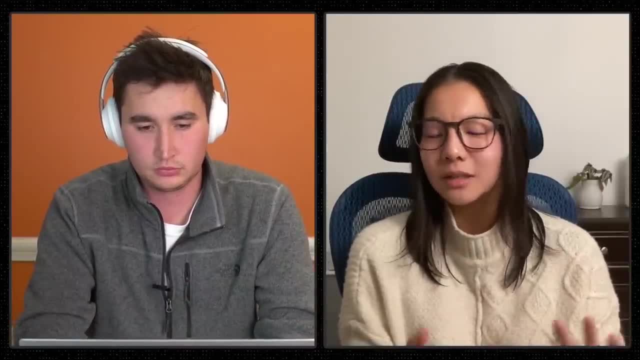 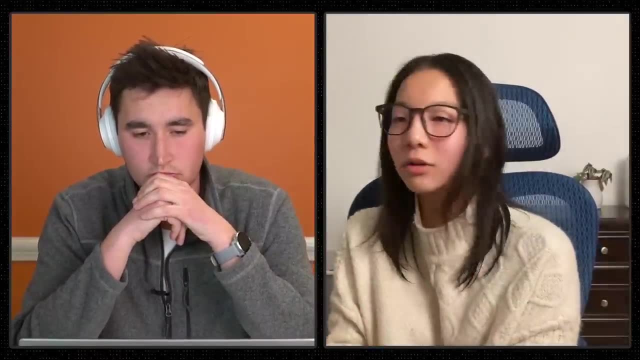 all really cool. I think that's really cool. I think that's really cool. I think that's really cool because it's it's beating humans at a game that you would think you know is only for humans, like chat, like a poker is built on psychology, math and randomness. You would never expect there. 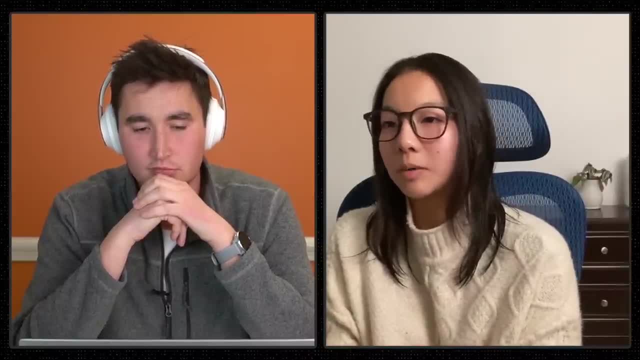 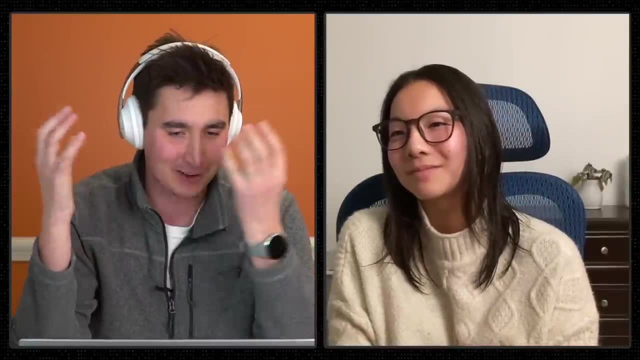 to be this like Nash equilibrium, like optimum solution, Right, But there is which is really cool. Yeah, It gets really, really interesting when you combine the psychology element of the human experience with machines, with AI, And I think that, from my experience, I think that 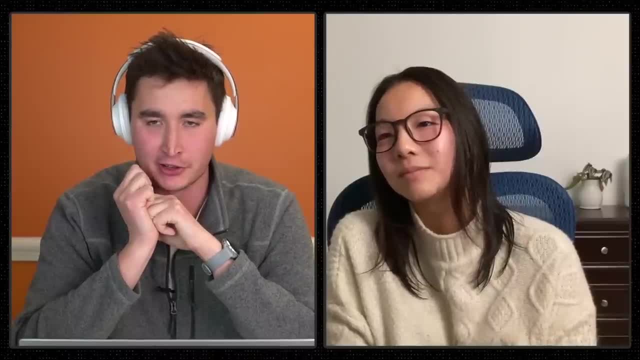 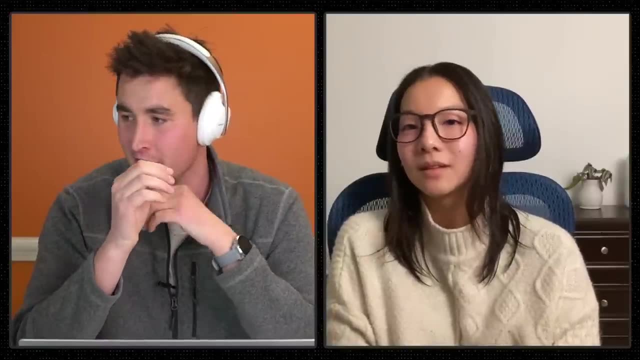 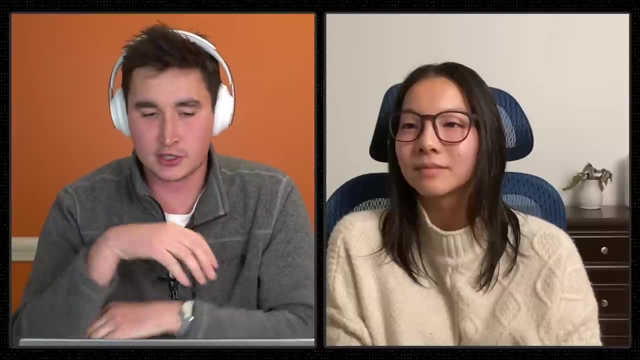 that's something that's often overlooked, and it kind of bothers me that it's overlooked because it's so important to the concept of artificial intelligence, if it's going to be that intelligent. So yeah, definitely. I think those things are super exciting, Awesome. Let's switch. 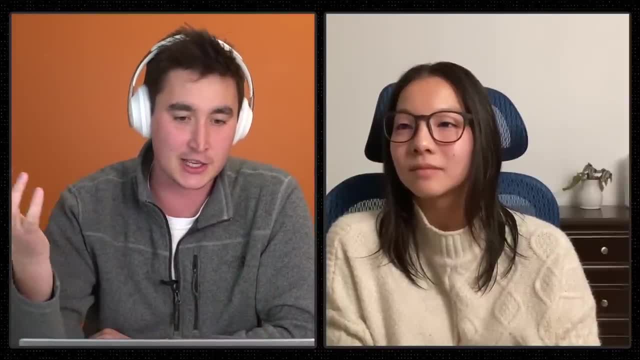 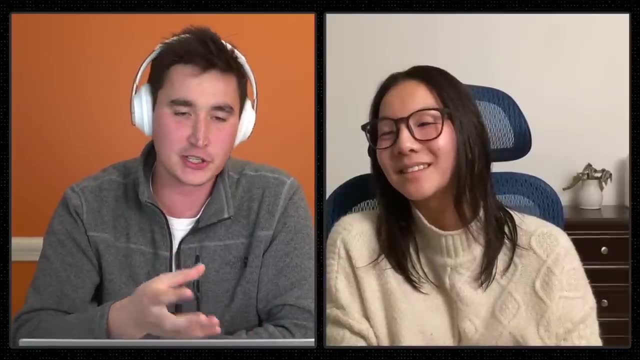 gears And I guess, to give you a little bit of context, my name is Geeth Kali. I'm a senior data scientist here on the team. So you know, the question that we're going to kind of present is something that we're asking a lot of people, And I think that's really cool. I think that's. 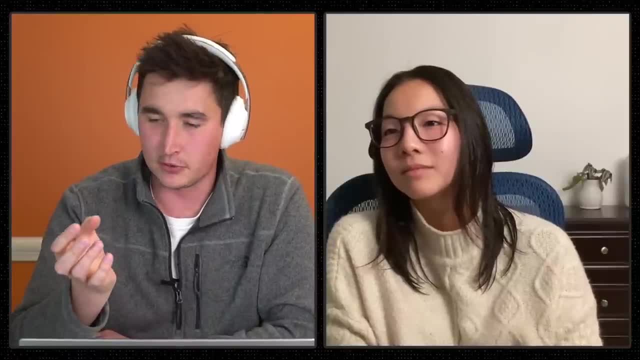 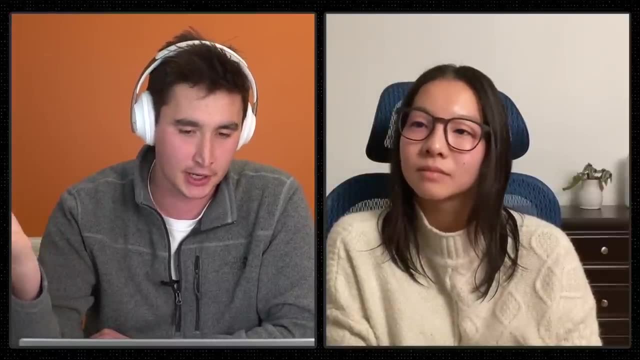 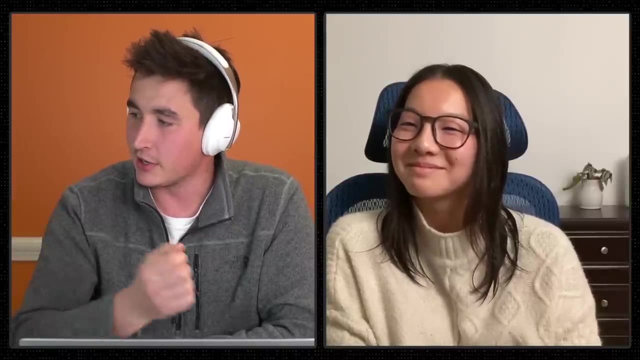 something that we're actively looking at here. So this is kind of the task right now. So you're working on as a data scientist on the team here at Gwitter. You know our CEO, Mr Elon Tusk, has been complaining a lot recently, And we're a social media site. 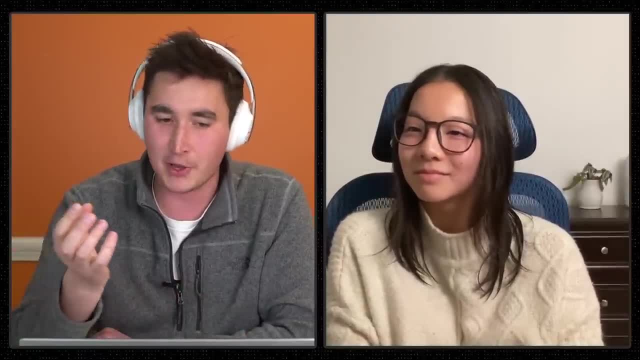 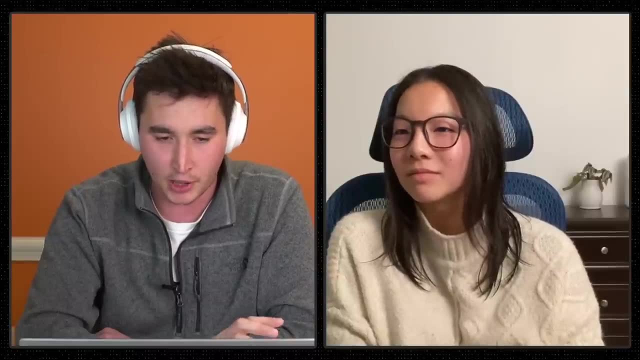 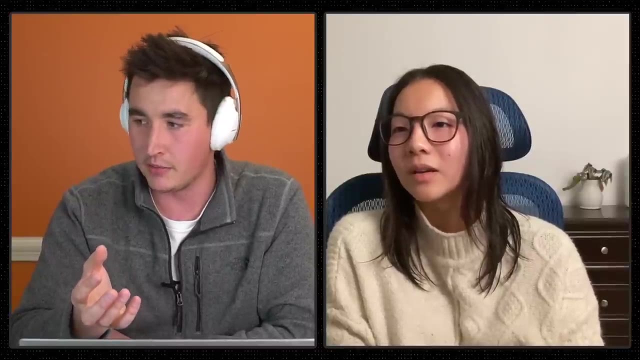 maybe similar to something that you might be aware of, But our CEO has been complaining a lot recently about the serious bot issue that's kind of infiltrated our site, or you know he kind of has mentioned has infiltrated our site and become a serious issue that we want to look at. We want 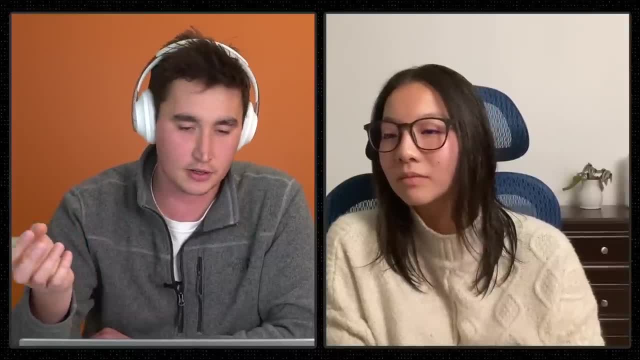 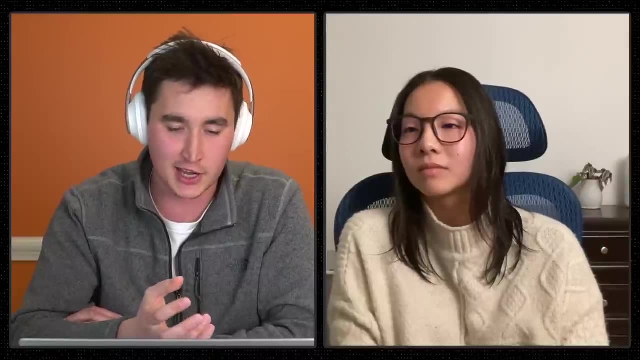 to. you know, mitigate and solve. So you know some things that these bots are causing some issues are. you know they're quickly responding. you know when our CEO posts and you know within a minute there's, you know, hundreds of replies promoting some sort of you know. 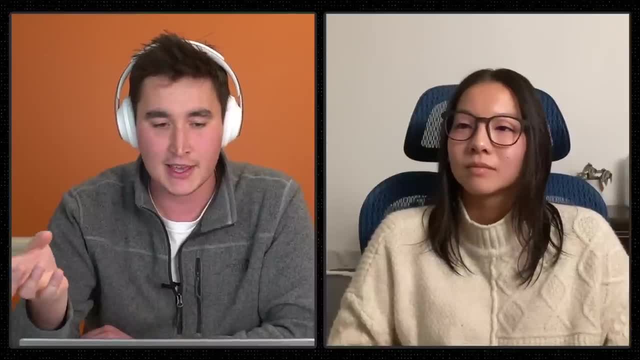 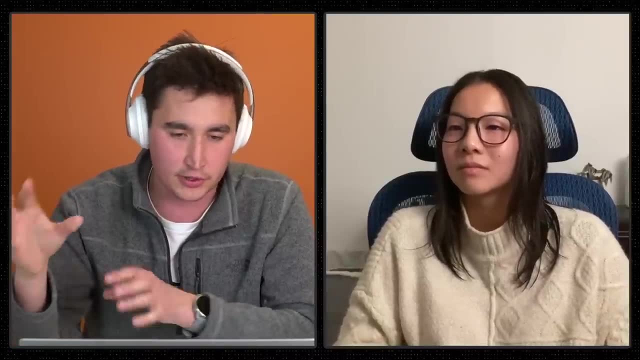 site, Some sort of program, some sort of- you know- money scheme. So there's bots that are doing these. you know quick postings. There's, you know, coordinated bots that are all over the you know the ecosystem, that are sharing propagandist messages and sharing fake news. 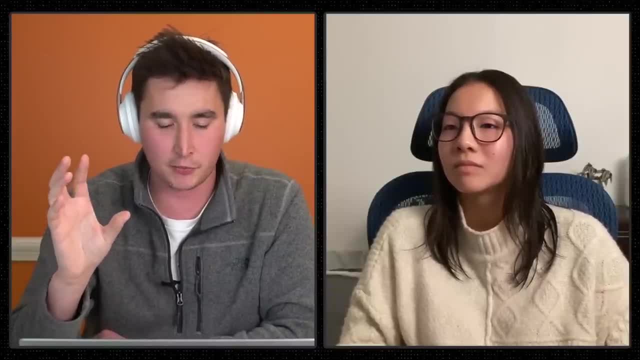 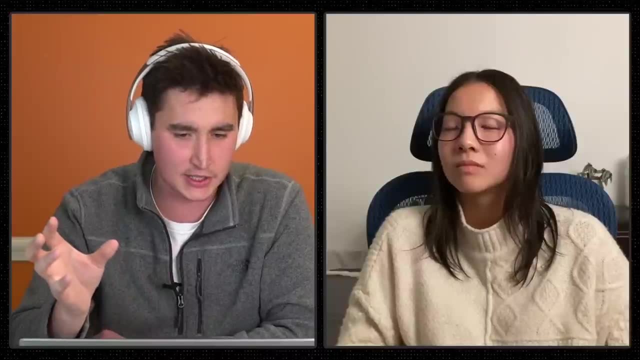 messages. So that's a little bit of context, I guess, before I dive into, like you know, some of the specific kind of guided questions. does that make sense? what I kind of presented, And I guess first off a question to you, just kind of this, is not really a data science question, but 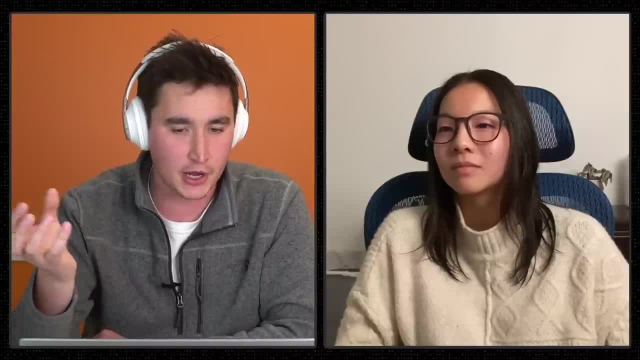 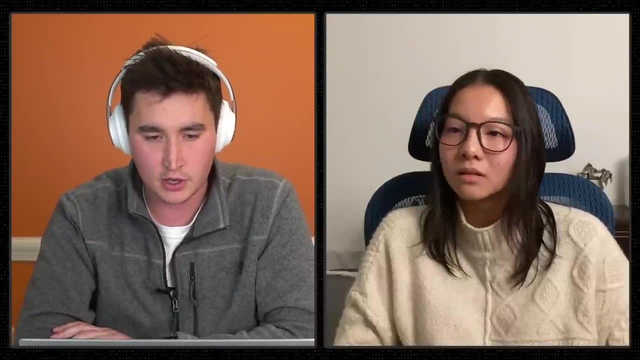 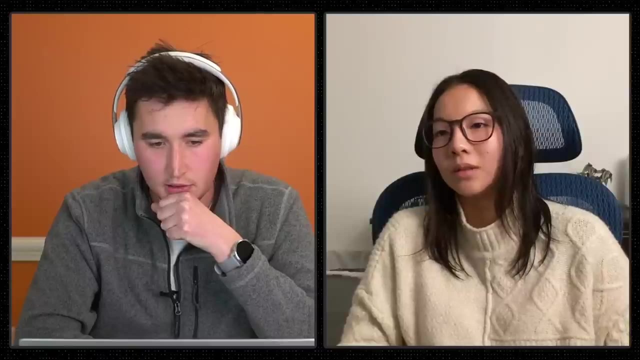 do you have any thoughts on, like other issues you know bots on this social media site might cause, and things that we should be thinking about, you know, when we're investigating this issue. Yeah, So I definitely think that obviously bots are annoying, right Like nobody wants to. 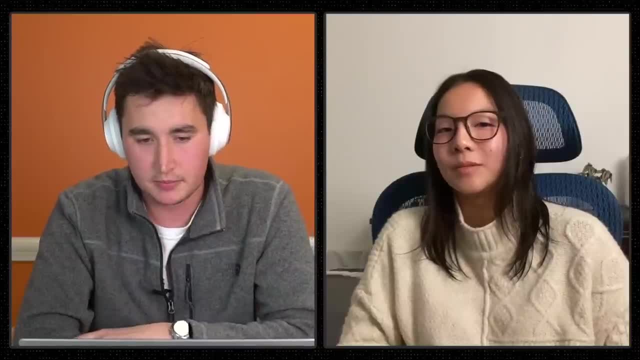 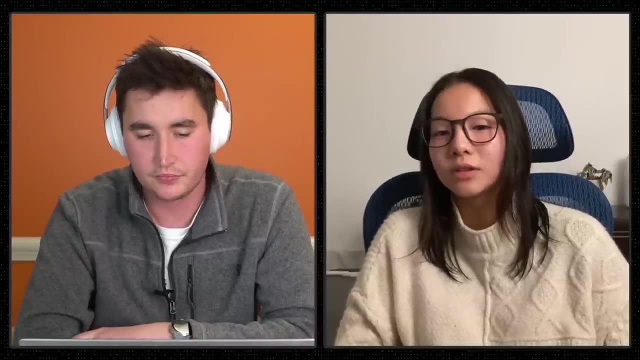 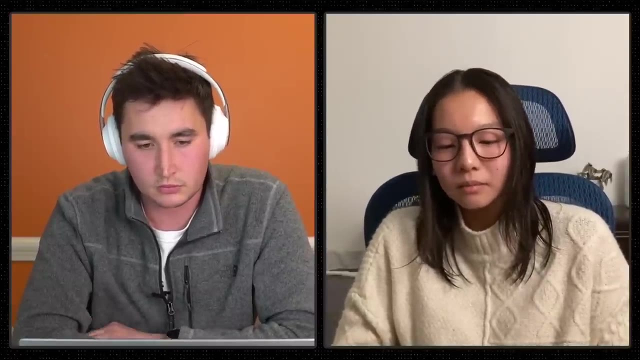 be tagged in a million things. Nobody wants their entire- what's it called- notifications to just be bots spamming them right, And I also think that bots take away from the real conversations that might happen on this platform. So to reiterate your question is, I guess, the current issue that 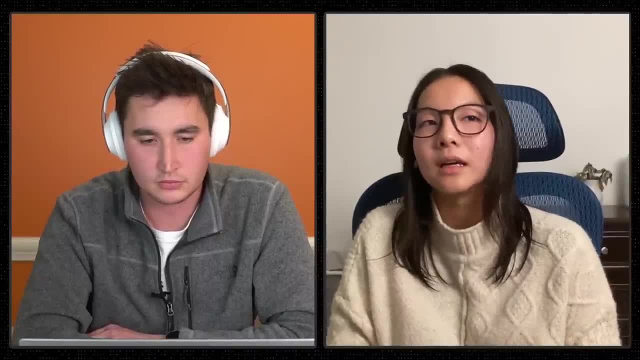 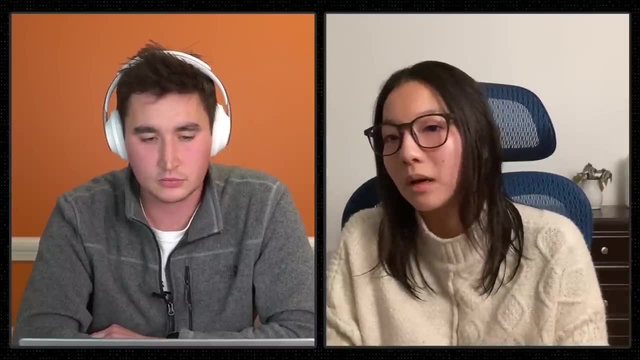 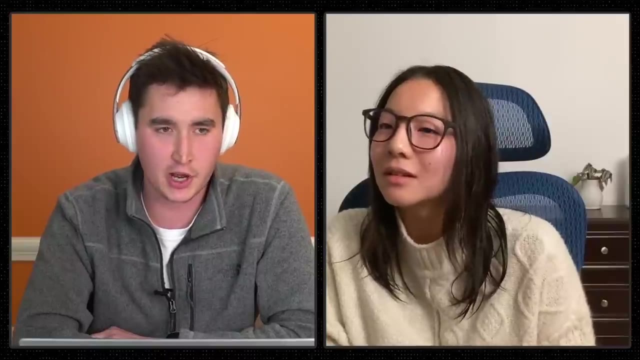 you're trying to solve is that there are all these bot attacks And, you know, immediately after posting, things get really crowded with these coordinated messages and spam messages, Like what else? Yeah, this is an exploratory question, I'm just curious, And you know. 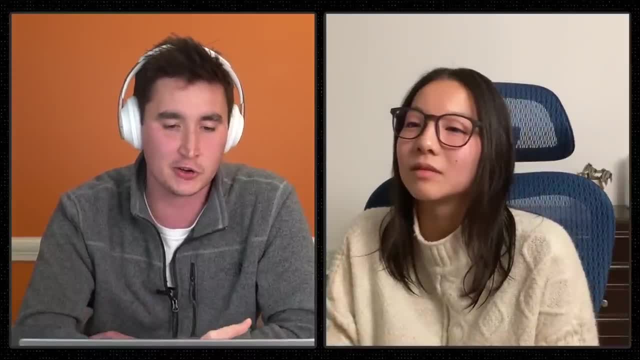 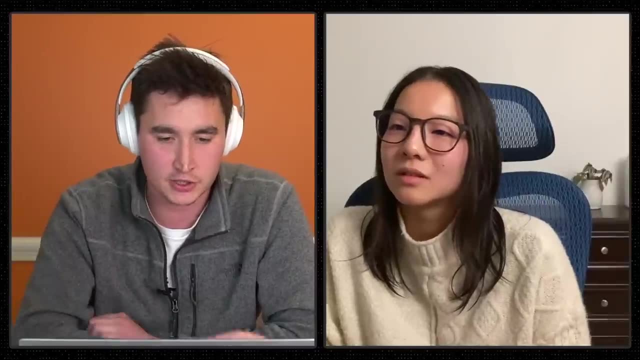 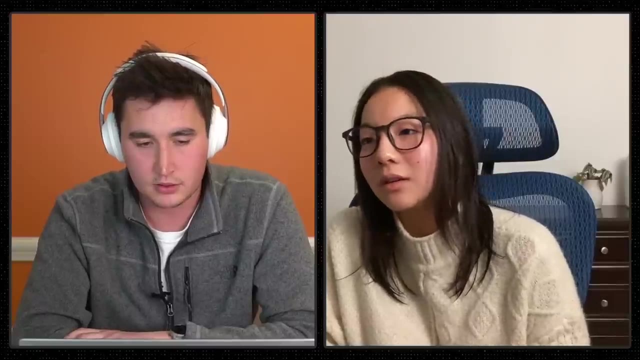 it's not really data science, It's more platform driven. I'm just curious, you know, pick your brain and see if you have any other ideas of like potential issues with having serious, you know, bot issues. Yeah Well, I mean, I just think that it like like I think bots are there to. 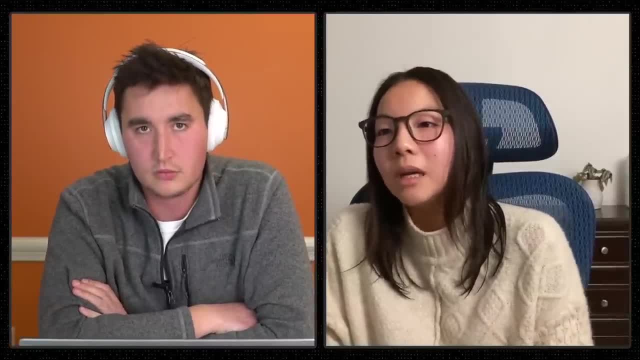 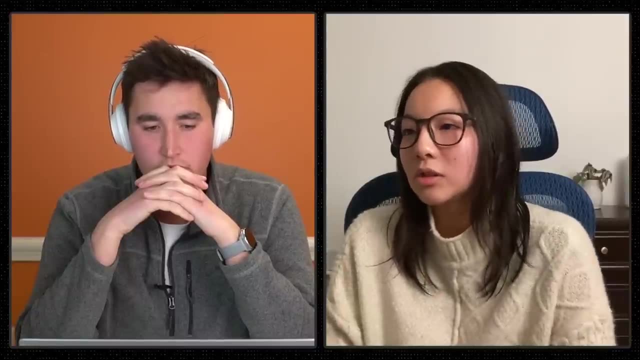 target a specific group right, Like all these money making schemes like: do you really think that they're making money Or do you think that they're making money? Like, do you think that they're making money Or is it just trying to scam people? And like: I know that, especially in a 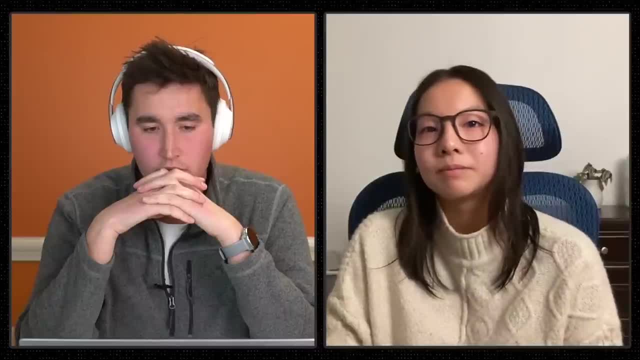 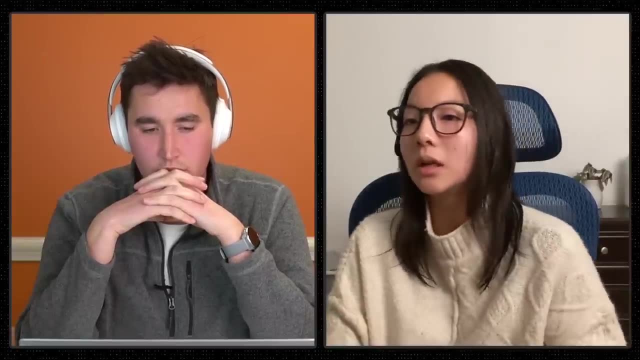 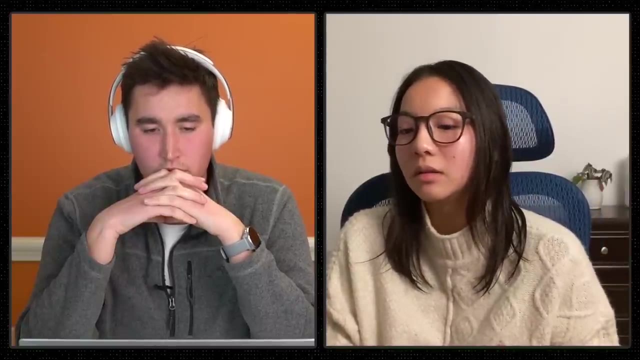 lot of the crypto world. there's a lot of bots that might that might just be links to these fraudulent sites which end up draining your wallets or stealing your NFTs or I don't know all these different malicious schemes, And so that's definitely one reason why like bots are. 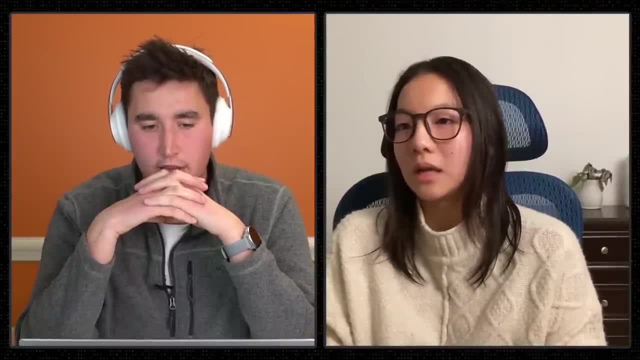 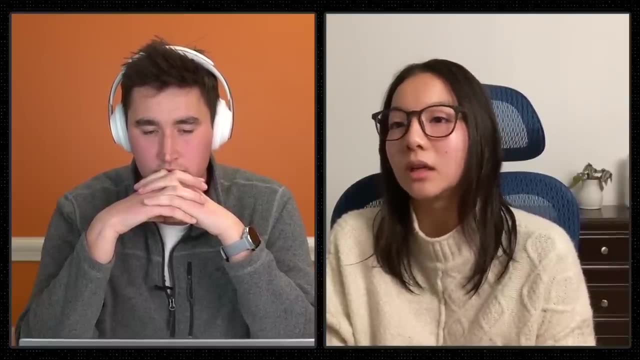 bad right, Because it's not just that it's crowding things, It's also that your users are literally being the ones scammed off of, and that does not create a good reputation for your company. Yeah, definitely, I definitely agree, And you know, obviously that's what we're. 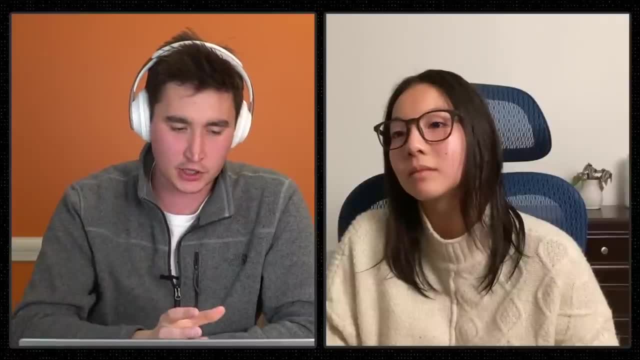 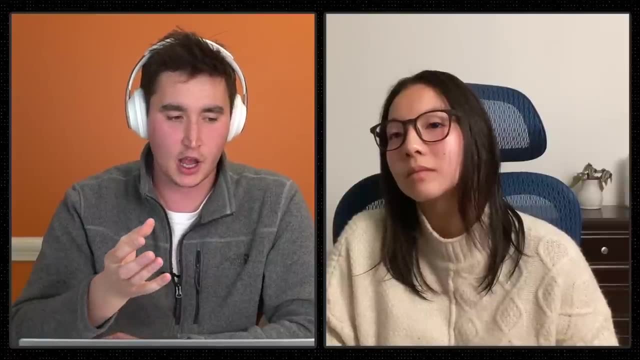 trying to avoid. So also I'm going to get into more guided questions. But also, like, given this context and just you know your background as a data scientist, you know, do you have any, any initial thoughts about the problem? Anything that immediately? 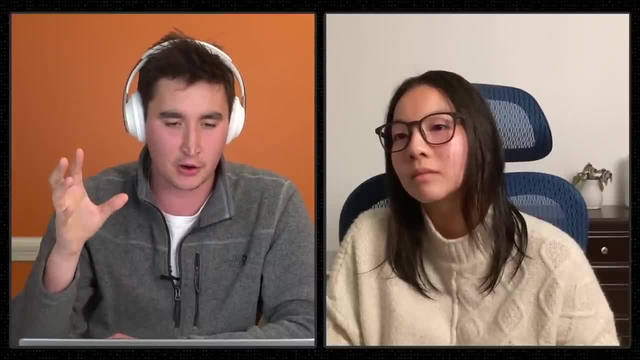 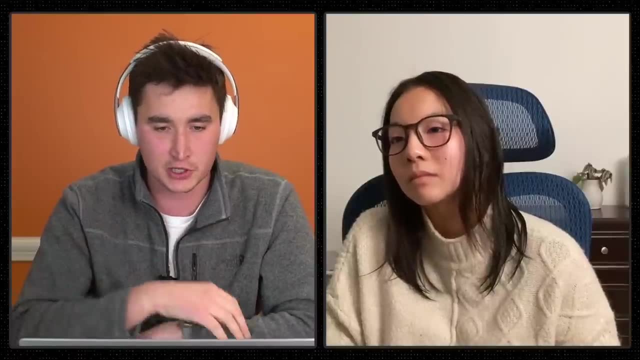 sticks out like that you would want to investigate about. you know just this high level I guess issue And we'll dive into you know guided stuff. But I just kind of also want to just gauge your high level. you know thoughts on, on the situation. 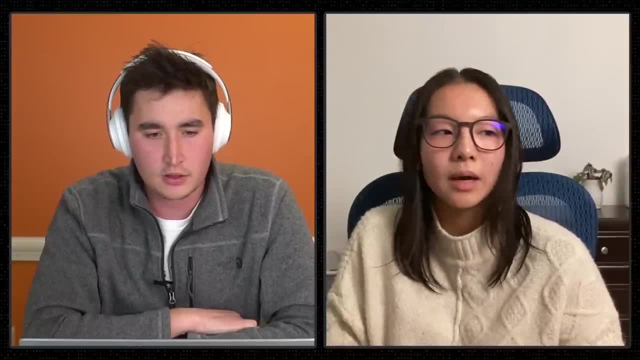 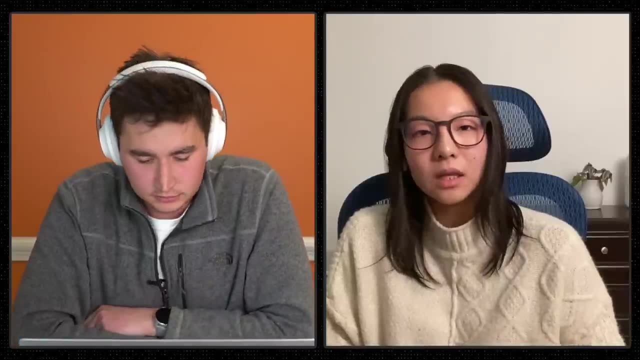 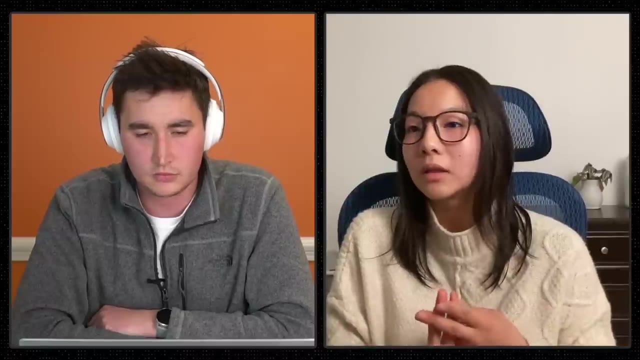 But like thoughts on the situation, do you mean just like what my first thoughts are on how I would tackle this problem? Exactly, exactly, Yeah, so I definitely think that with these bots- you mentioned a few different things- right that it's coordinated, that it seems like they're. 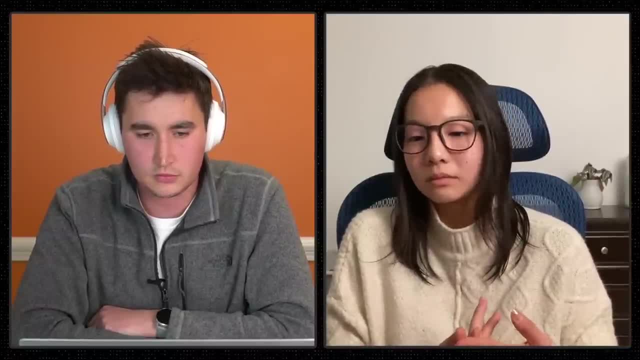 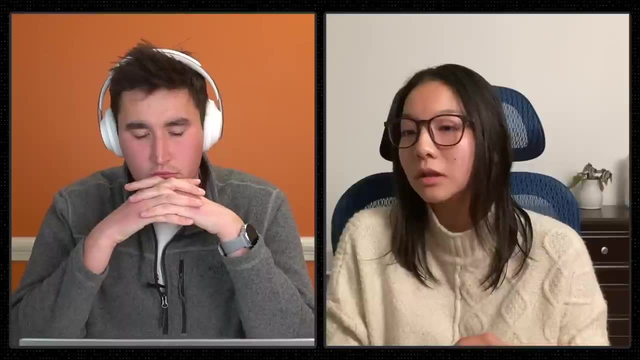 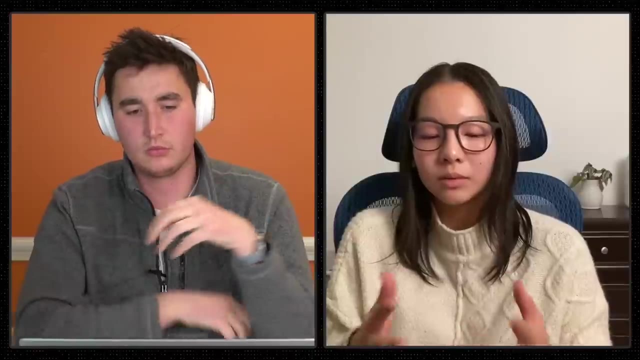 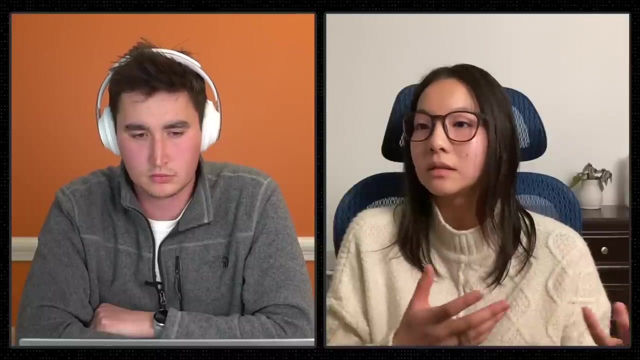 filling up immediately After a post has been posted. It seems like you know there might be links to certain things or certain themes that the attacks are always about, And so I would start maybe investigating a bunch of these things and trying to figure out certain features of these attacks or these spam. 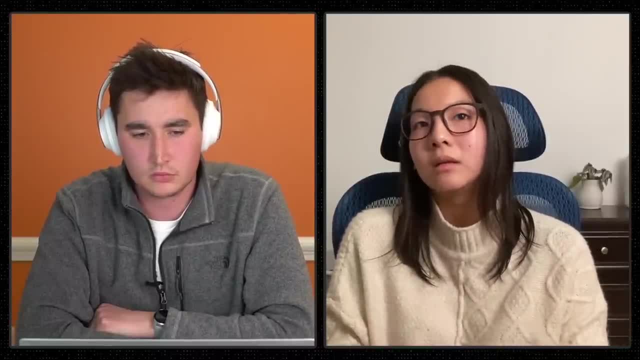 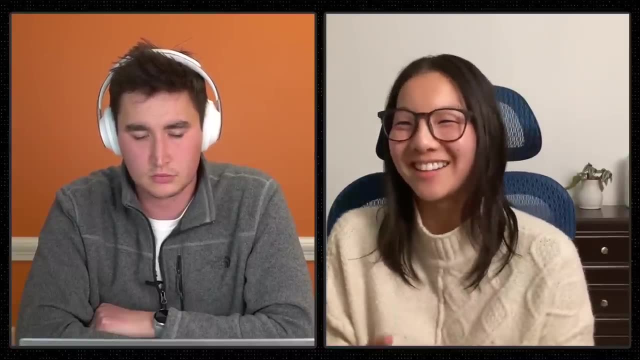 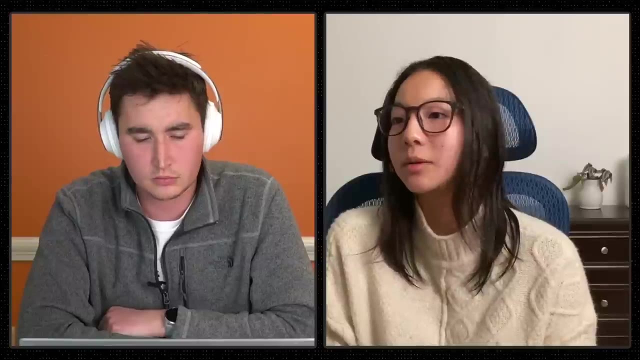 messages that might be able to for us but certainly say whether or not this is a spot, a spot, a spam bot attack, Yeah, And I. I also think that you know there are certain other attributes, such as if they tag a ton of people right, or if a single account posts multiple times, or maybe the account follows a ton of people but nobody follows them. I think these could all be certain traits of a spam bot, And when you have multiple of these things in conjunction with one another, then that strengthens. 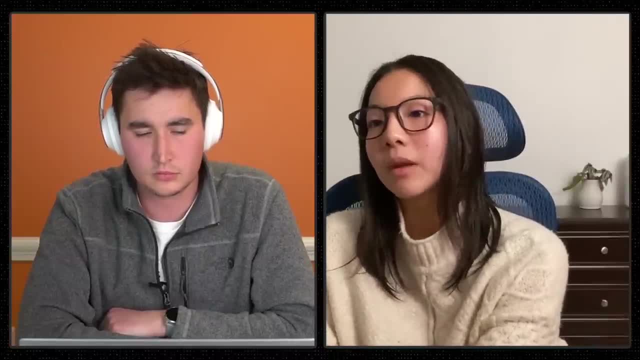 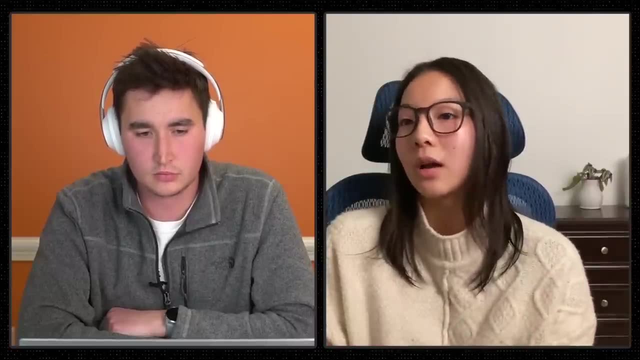 the case that this might be, you know, spam. So I think that those are all different things to consider And maybe we can train a model based off of that to classify whether or not a message is spam. Awesome, Yeah, And you're kind of, I guess, getting ahead of even what I was, I guess, planning. 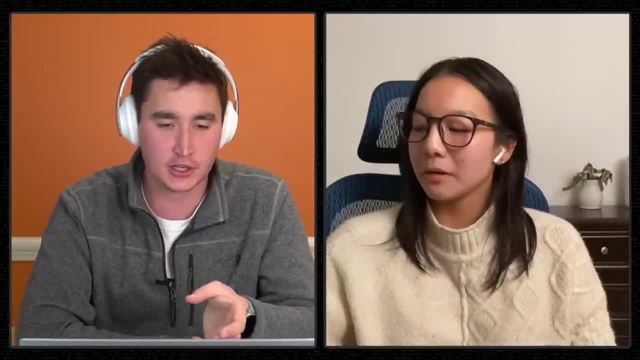 on asking next. but this is exactly kind of where the discussion is going And I think, I think, because you've already kind of hit on some of the things that we've been talking about, you know you've already kind of hit on some of the things that we've been talking about, you know you've 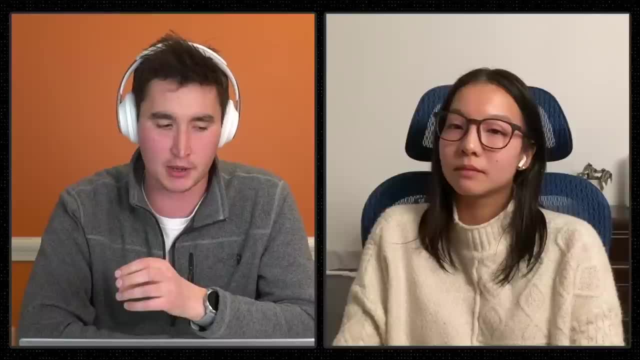 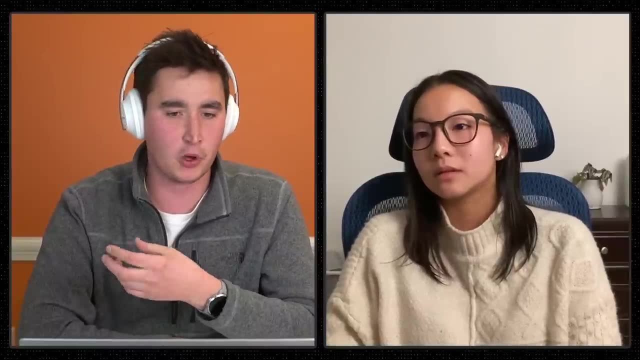 already hit on some of these points. I think maybe it would be nice to kind of drill down a bit more on. you know some of these features that we're talking about here. So what I'm going to do? just because I think it's helpful for both. you know myself as the interviewer as well as you. 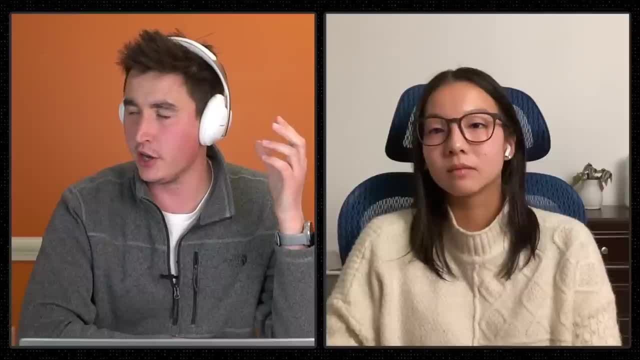 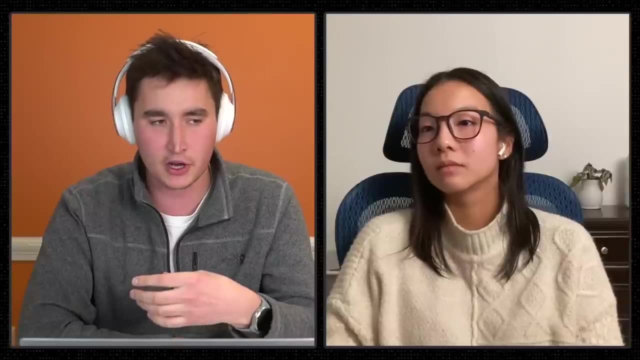 you know, you know brainstorming and thinking about these things. I'm going to share a Google doc and let's try to, like I guess, get some of this on paper and we might drill into some of these a bit further, And then I'm going to kind of ask some additional questions about this process. 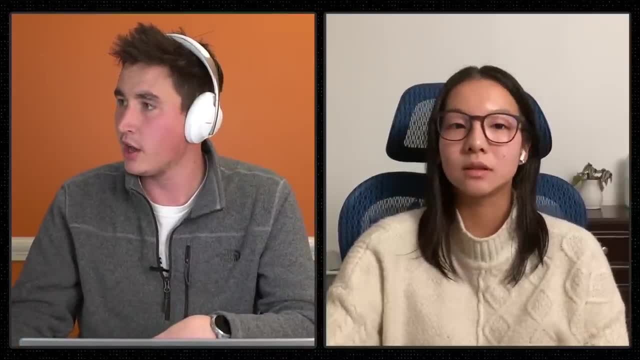 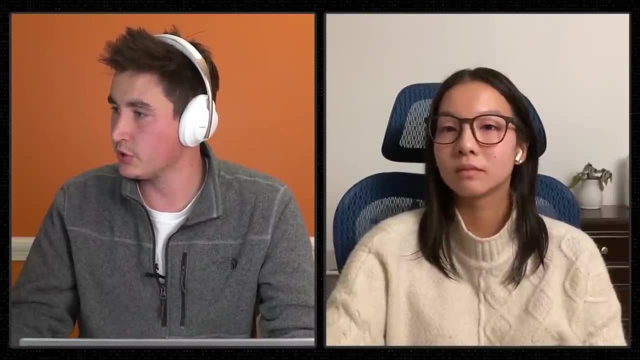 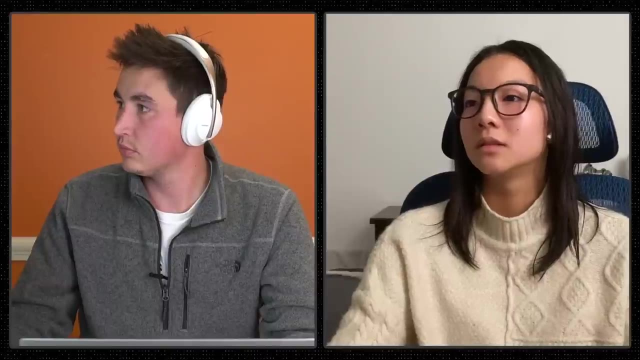 and we can dive into those aspects. Okay, further, So great. I will share it just through the. the zoom One sec. The zoom chat Sweet, Oh, no, no, Is that? can you see the screen? Yep. 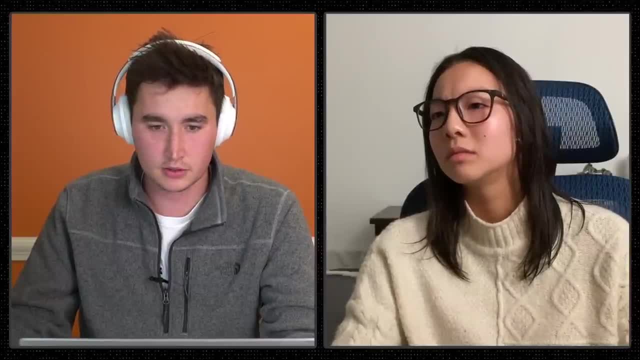 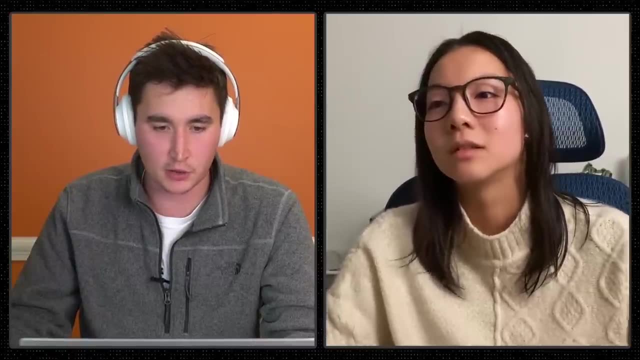 Not on zoom anymore. Oh, not on zoom. Interesting, It's like a really thin line right now. Oh yeah, There we go. Let's try that again. I think it's because I switched where it was on the screen I have. 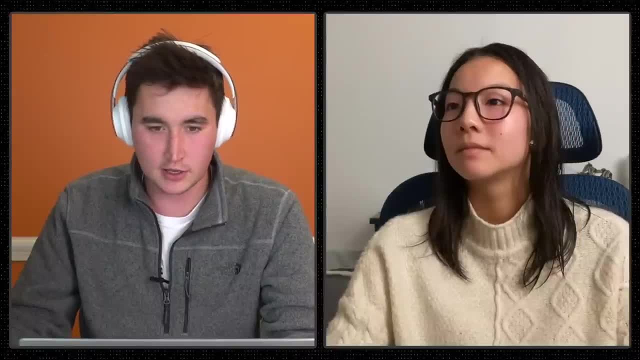 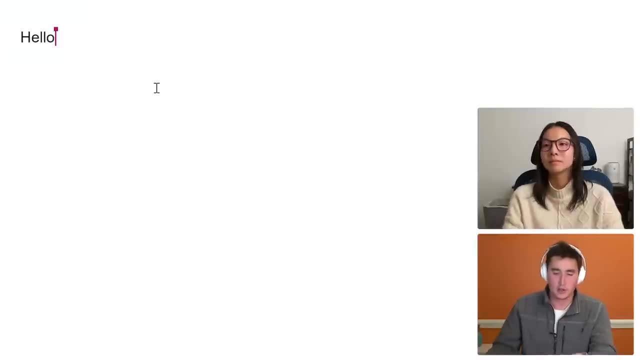 two screens open. I switched the screen. You know how it is, So can you see that on zoom? Yeah, Cool, All right, So I guess let's just start off. Hello, as well, I'm going to delete that quickly. 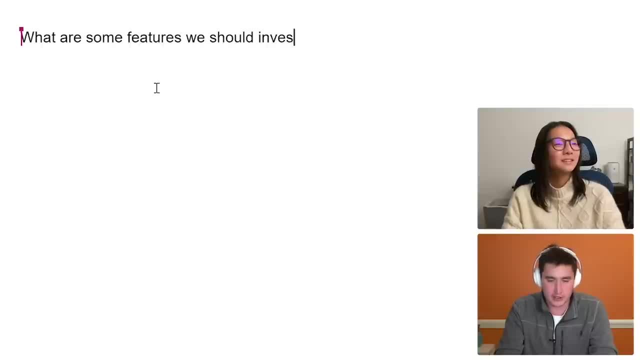 What are some features? Yeah, We should investigate. So I I labeled the question as what are some features we should investigate. You can kind of interpret that as you will. just basically, let's just drill down and just get some bullet points, Maybe some of the things you just mentioned, just because I'm going to be helpful for reference. 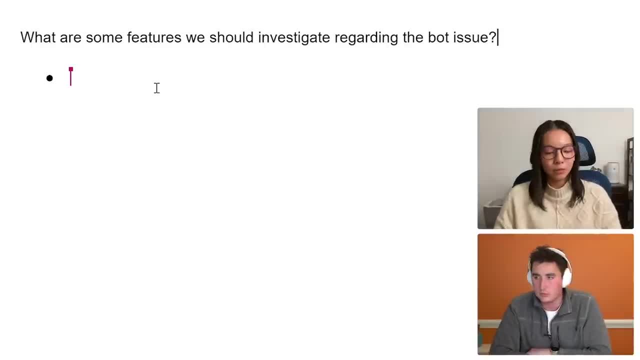 throughout. Yeah, So I definitely think that when you look at some bot attacks, I think that there's there's probably a few main things to look at, but the two that stand out to me are the content of the specific, the specific post. So, content of the post and then, as well as the person or 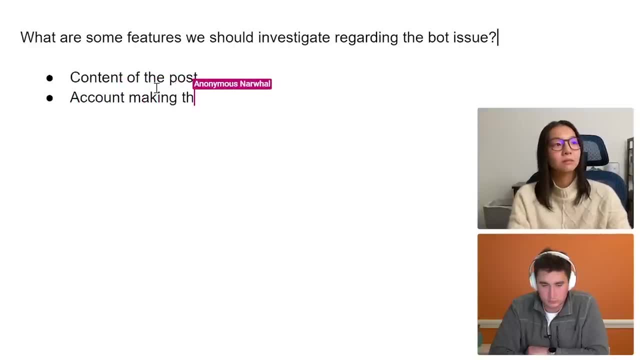 the account that's actually making the post. So I think, in terms of content of the post, these are things such as: um how many people do they tag how many tags? or, for example, um timing of the post, or words mentioned in the post. um what are other things? maybe links, maybe, maybe images, um. 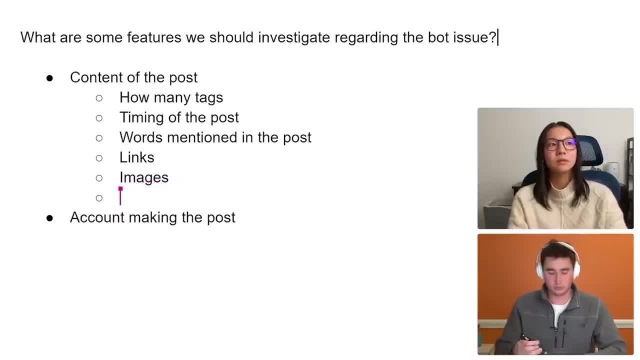 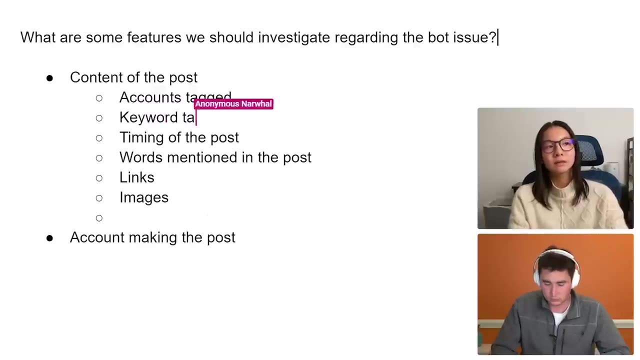 let's see what else. when i make a post, i type something, send it out, maybe tag. oh well, okay, by tags i mean accounts tagged, but also i think like keyword tags could also be another thing to look at. okay, it's like hashtags versus accounts tags. yeah, yeah, that makes sense. yeah, yeah, hashtags. 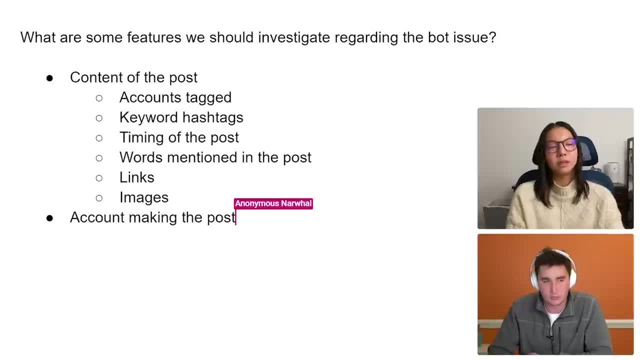 that's that that covers a lot of like what would be in a post, and then the account making the post. we might want to see, like, how many followers- yep, they have. um, maybe the number of accounts following or followed. yep, so, followers and following, following um. 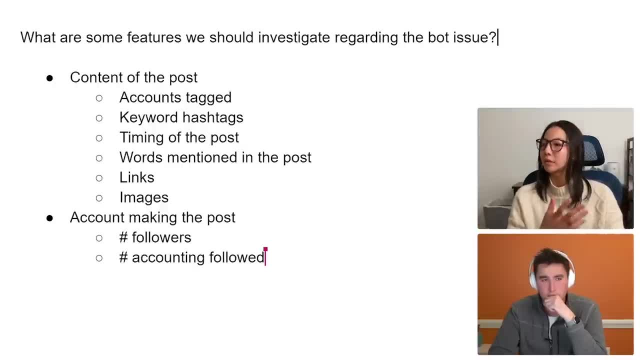 and i think maybe like looking at a ratio between. that might be a good idea as well- say that one more time, i missed that- maybe like the ratio between, okay, the number of accounts that they follow and then how many followers they actually have. yep, um, i also think that if you 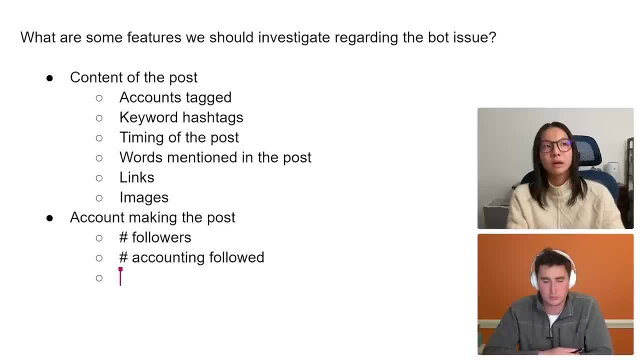 want to look at the followers, maybe, um, who the followers are. because, for example, if we've already labeled a few accounts as specific spam accounts, then when we- i mean if if one accounts followers are completely spam accounts that we've already labeled, then it's very likely that that account itself is a spam. 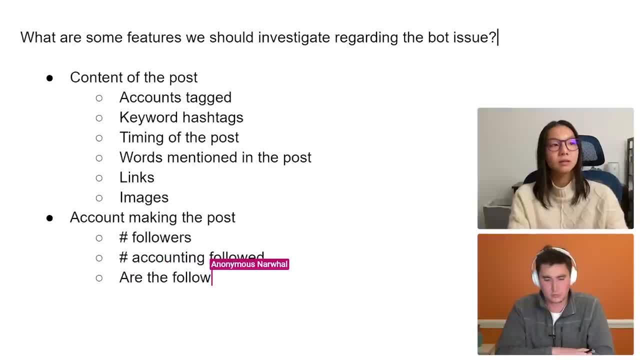 account, right. so, um, are the followers spam accounts? um, and something else could be, um, like the types of posts that they make, like, how repetitive are the posts that they make? so, if the account is posting the same thing that they're posting, the same thing that they're posting, 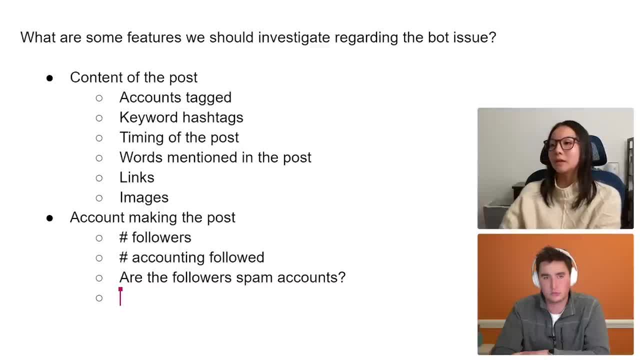 every time like: hey, check out my like, yeah, youtube video. and the same link every single time, then it's likely that that's spam, right? um, content of account posts, and i think one more thing to consider could be: like for the content of the post and the account like. so i do think that 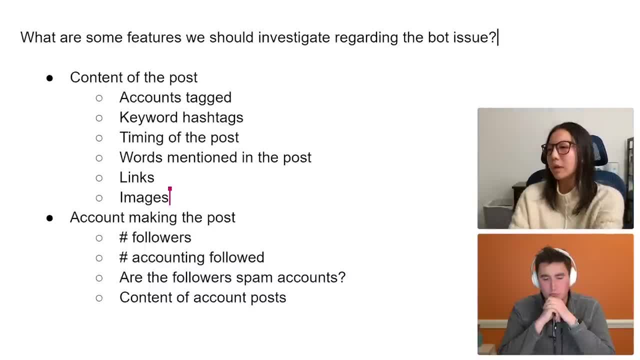 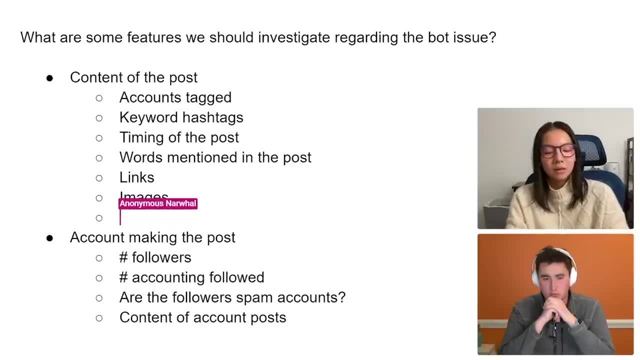 you guys have probably a report spam feature, correct. yeah, yeah, we do okay. so i would say, like i mean something that we could do is how many times has it been reported spam? um, or like how many times has something similar been reported spam? but i do think that is a big. 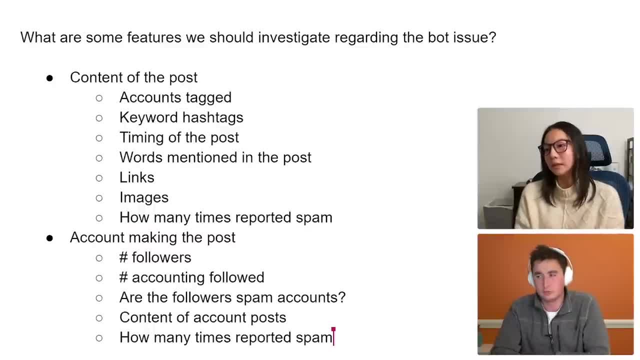 indication in terms of both the content and the account itself. yeah, definitely, i think this is a definitely a good starting list. um, anything else that you can think of and maybe kind of think a bit outside the box here. uh, it doesn't necessarily have to be outside the box, but, um, i guess one thing that i immediately see: 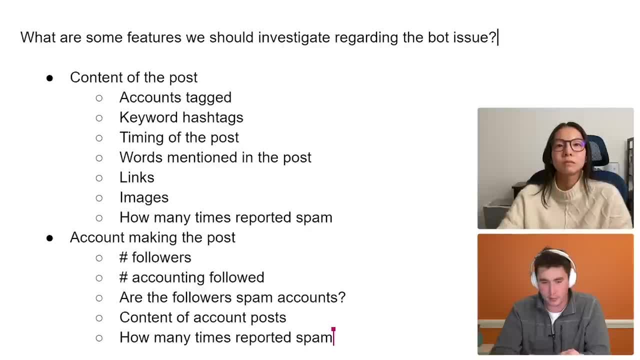 is that you know all these things are very publicly facing. i'm just wondering too, you know being the system administrators here, is there anything else, maybe on a more internal level, that we might be able to factor in on the the box here? yeah, i think that's a good question. 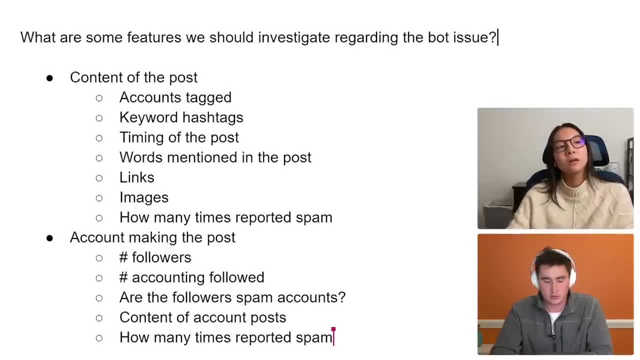 yeah, so well, okay. so i do think that one internal thing would be like this reported spam: yeah, definitely. i also think maybe another could be. you know, you mentioned earlier that there were these coordinated attacks. so i think, if you see like a cross, like if you see a spike in the number, 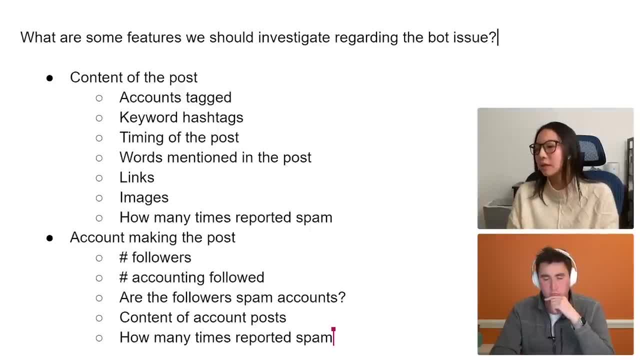 of posts being posted within like a five minute interval or something like that, and the content of all these posts is somewhat similar, like the- i don't know- documentation distance is somewhat similar or something, then perhaps those would all be, um, that could be like a coordinated attack, right? yeah, yeah, okay, yep, so like similarity in amount of posts. so if 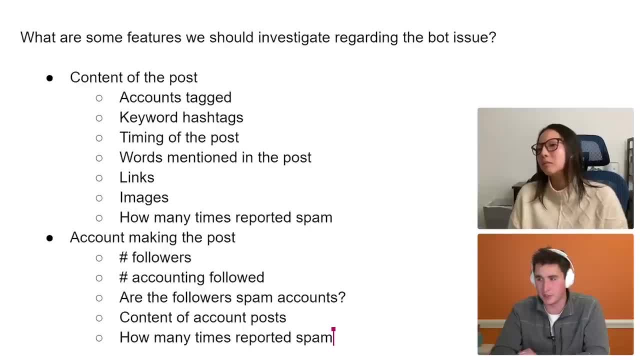 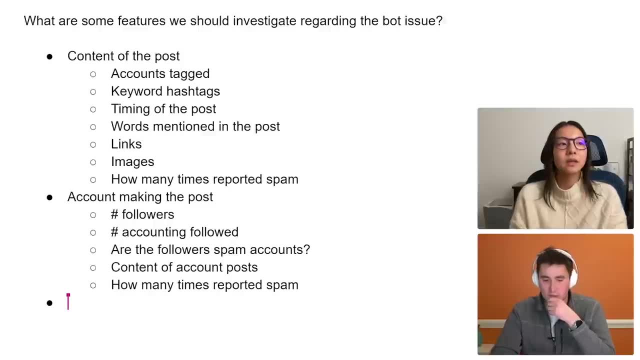 you just see this massive spike, then basically that might be some sort of indicator. so somehow to capture that spike, yeah as well. so maybe i'll. yeah, so maybe i'll add like a separate category and just be, and this could be like um, aggregated action or aggregated things, so maybe one of them could just be similarity of posts, um, in small time frame. 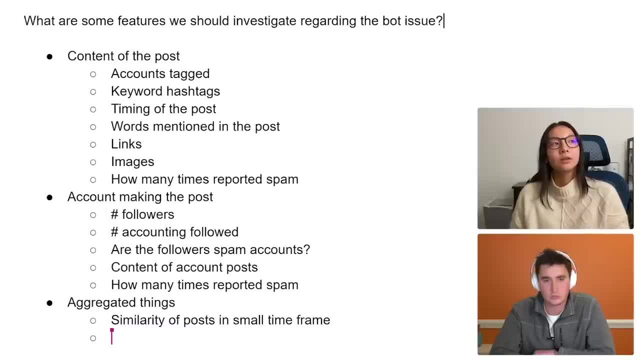 um, something else that twitter might have access to or the platform might have access to. uh, okay, let's see, i have like, well, okay, so things that are private to an audience but are public to internal, uh, twitter might be the emails, even email addresses, of the account. yeah, so that could go under the account making. 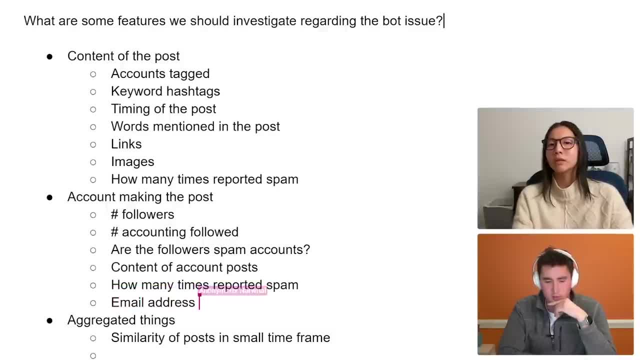 the post. so like email address, um, i don't know whether or not you require all these emails to be verified, but maybe, like, maybe if it's not a common domain, or maybe if, um, if you're like, maybe, if, um, maybe, if, like, there's a lot of random letters in the email, like the prefix, then those 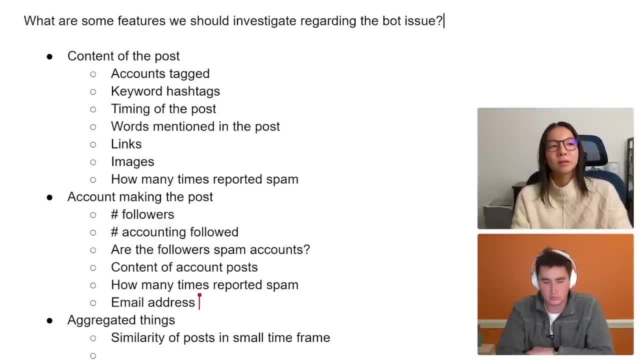 could all point to um more spam, like- and i think that this could be a little bit tricky because you know, back in the 2000s we all made like really dumb email addresses, right, uh, so i think that this could get a little tricky, but i definitely think that there are indications. 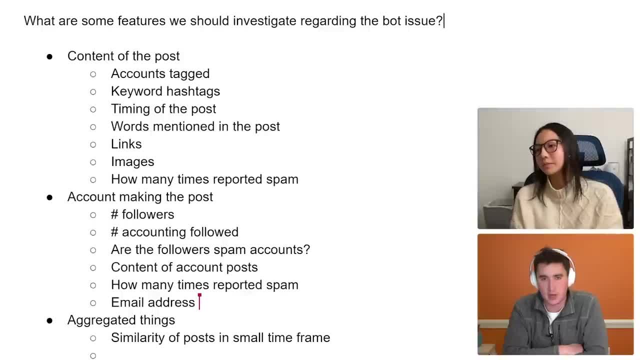 of whether or not something is more spam. like definitely, and i think that you made a really good point there- with domain name. uh, just, you know, for context here too, like uh, you know you, you're more likely to be able to trust a gmail address, maybe than a, you know, random address. you've never. 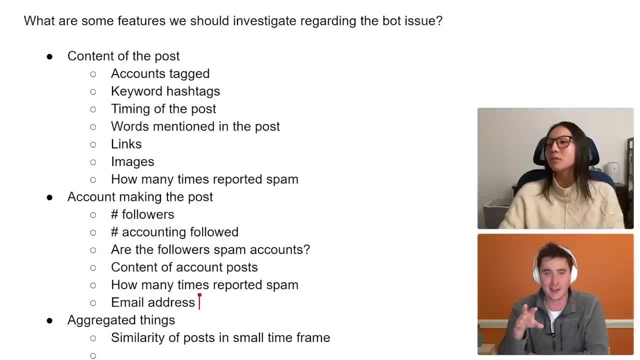 heard of. so, like some sort of waiting scheme could be interesting here, right? uh, i guess, an aside- the reason- yeah, the reason why i was kind of like hesitant about that as well, was because, like, for example, you might have your own domain name, right? yeah, geethcallycom or something like. 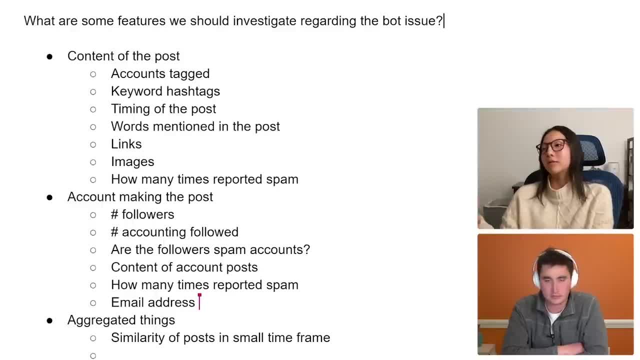 that, and so your email might be like info at this rent this like custom domain name, in which case we would want to make sure that people using that email address that does not get caught up in this like spam filter and filter too harshly that just because of the email it's considered spam. yeah, i. 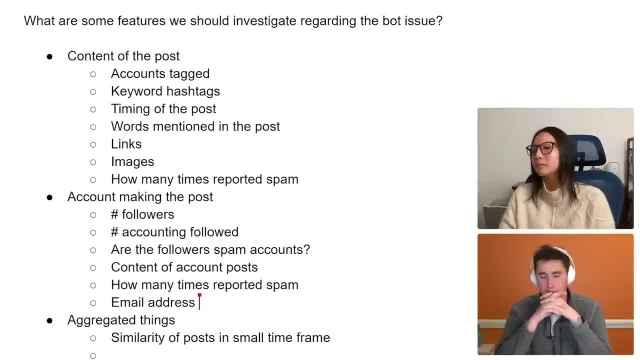 think the way that i would look at it- and i think that you know, i think that's a really good point you're kind of hitting on this- is that it could be an indic, like i think a good domain address could be a indicator of, like a valid account, whereas maybe a bad one doesn't say that much. 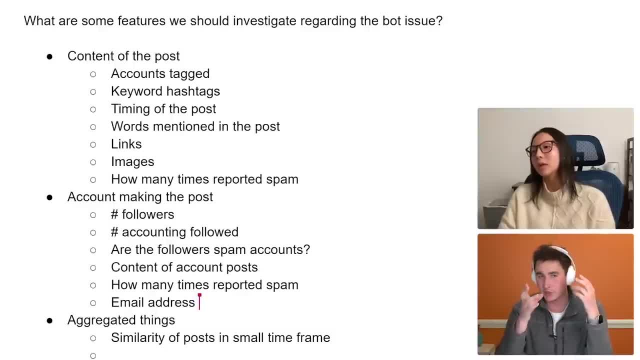 i think that's kind of the point you're making. yeah, interesting thing just to note about gmail, just because i've been through this experience: gmail very much limits the amount of accounts that you can make um for a certain ip address. so that definitely would help, you know, capture some positive emails, because they could only make some. 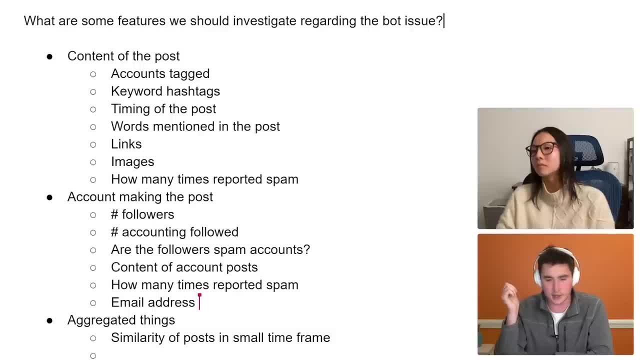 money easily. uh, cool. i think this is a great list. i think the only other things i might add here is just like post engagement, um, but i think this kind of encapsulate is encapsulated in a lot of the other stuff. like you know, post engagement likes retweets, all that, or yeah, yeah, as well as. 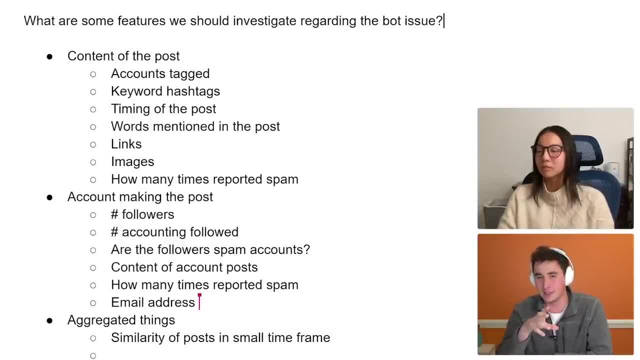 looking at the, the details of who is liking these things, if it, as you mentioned, with the followers, if it's always the same spam accounts that we've identified previously, probably not good engagement, not organic engagement. so i think this is a great list. um, for this portion, i think we can kind of move on to. 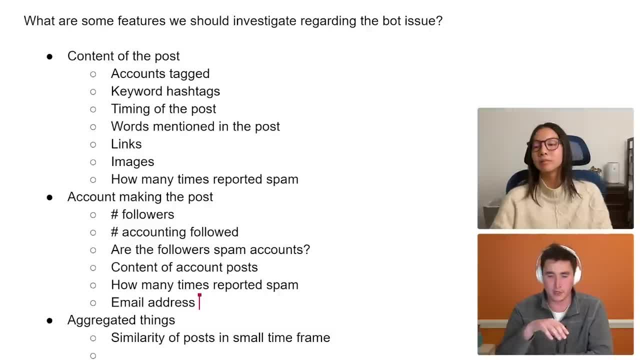 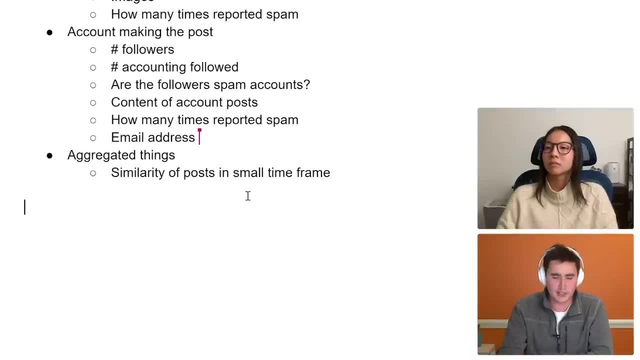 some of the other questions about the task, but we'll keep this here for reference, so i'm gonna go and scroll down a bit on this post. um, the next thing i want to discuss- and you know you can maybe start jotting up some thoughts on this- is like: okay, we have all this idea of what we're looking. 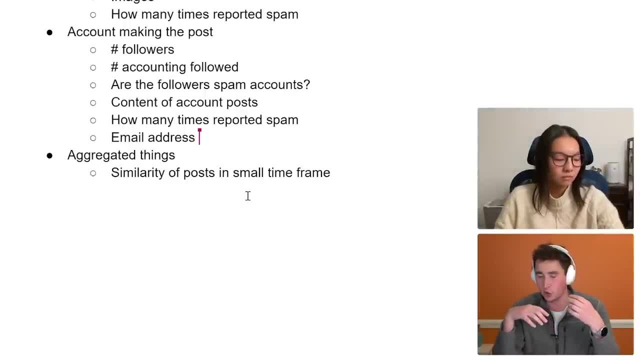 for i mean a big portion of building. let's say, our goal as a team was to build a model that could identify and potentially remove these bots. um, you know, a big portion in training that model is having, you know, a data set to work with. so i think thinking about the concept of a data set, 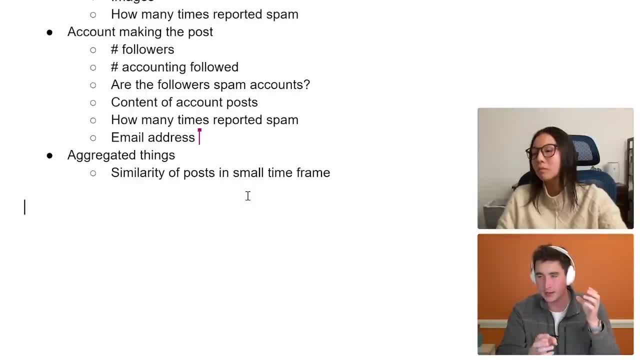 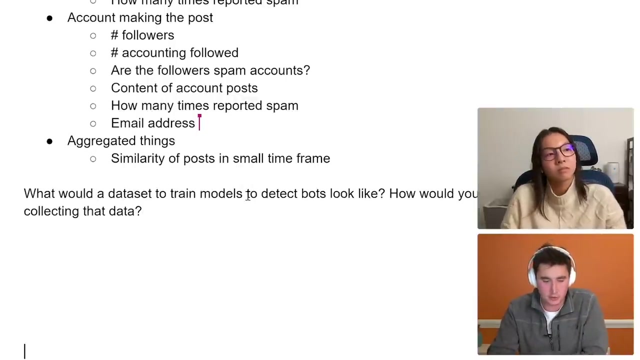 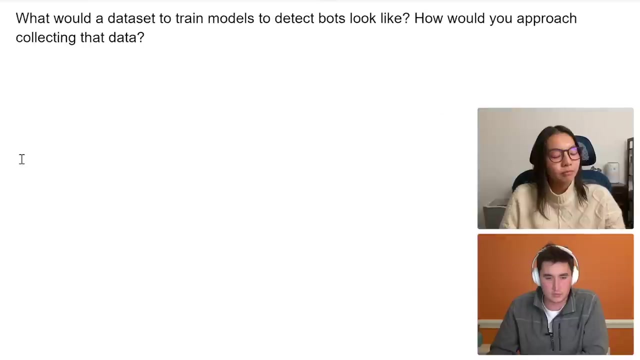 here. you know, what might that data set look like and how would we go about? one second, let me just write this out as i speak it out. yeah, and then how would you approach collecting, i guess, that data? so kind of an open-ended question, but i think it's a good one to. 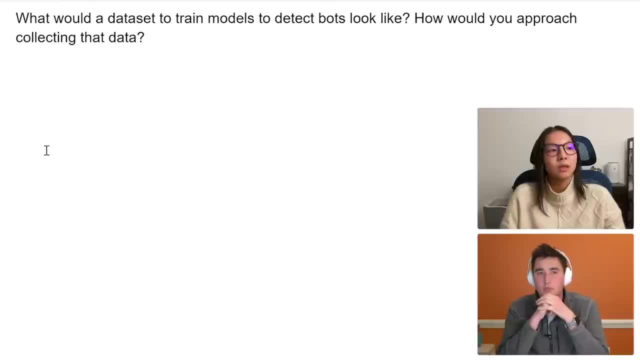 you know, start discussing, yeah, yeah. so, um, look at this first part of this question: like, what would a data set to train models look like? okay, well, so what exactly are the models that we're trying to train? right, and i think that you know of a lot of the the models out there. um, i think many of them would look very similar. 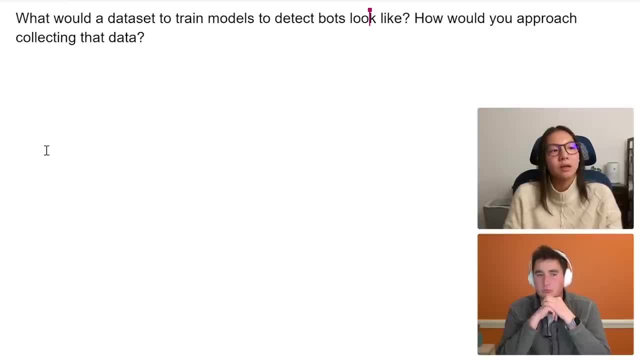 and i think that, specifically, uh, we want some sort of feature vector to be able to feed into these models, and that feature vector, well, it should probably summarize all the things that we just mentioned above, right? so, um, i think, in terms of, so, i think, this question also 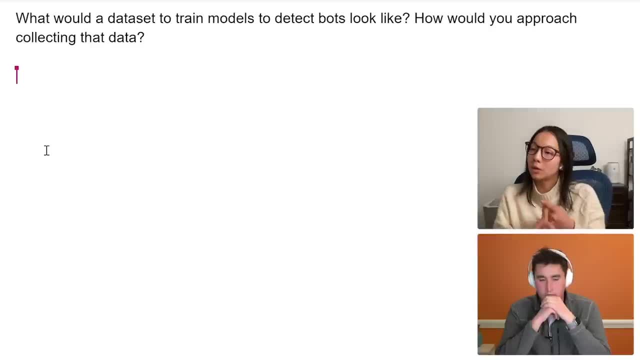 um, so i think this question also. so i think this question also comes down to: are we trying to tag the post specifically like: do we have a model that are detecting spam posts or spam accounts? and those are two different questions that we're trying to ask, right? yeah, actually, yeah, which i 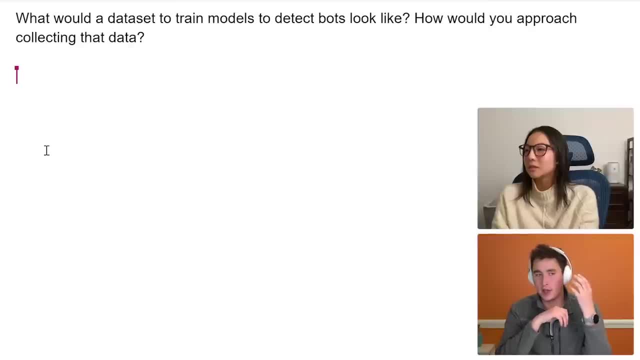 would say in the context of this question. what i was thinking about was a- i think that it's good to you know, think about both, because you know one model probably wouldn't work for the other use case. but i was thinking specifically about bot accounts and trying to detect those bot accounts. 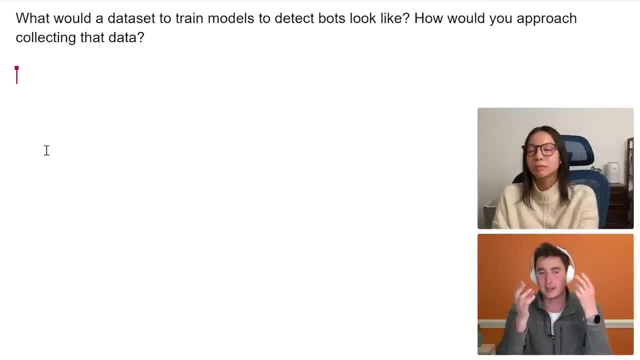 right, you know, as a model, how do we kind of like train these bot accounts? okay, and then you know what the data set might look like to help train the model to you know, predict and and detect unknown- right, you know- accounts, okay, so if we're trying to specifically target these accounts, then i might 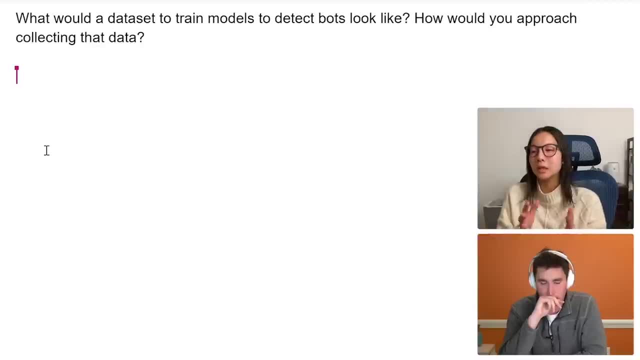 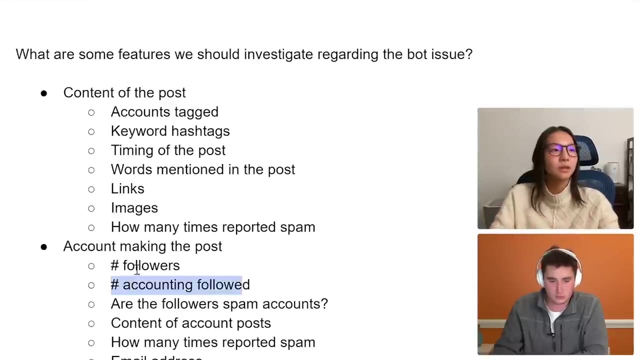 focus on more of the attributes of the account, making the post that we had listed above. so that so, uh, the bullet points under that are such as: number of followers, number of account and page that follow them. so counts, yeah, and then are the followers also spam accounts? 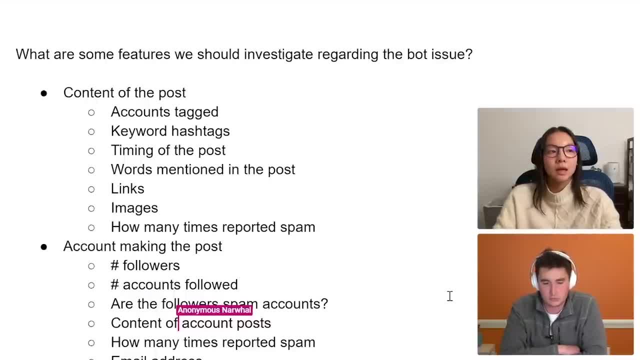 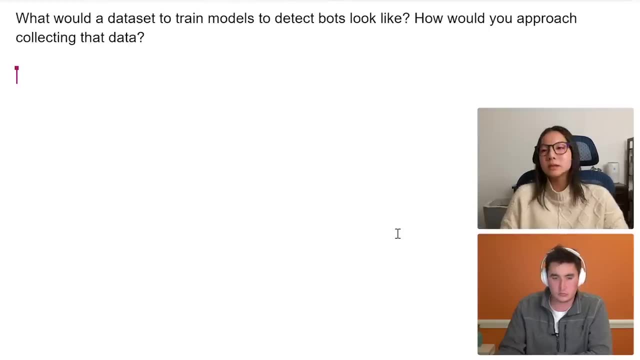 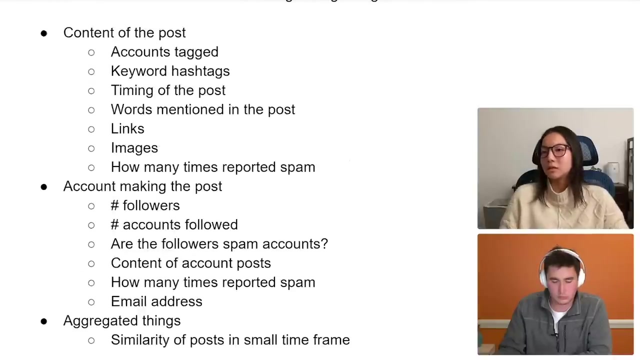 maybe the content of the account. so maybe we can look at the last few posts, how many times this account has been reported spam, the email address of that account, and I think that the most basic thing that we can do is just feed everything into kind of an URL net. right, I'm gonna leave this so for certain. 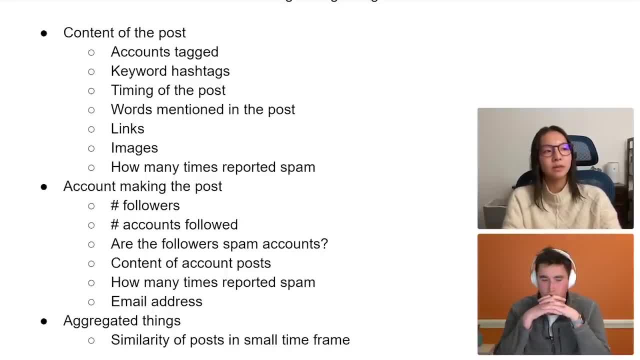 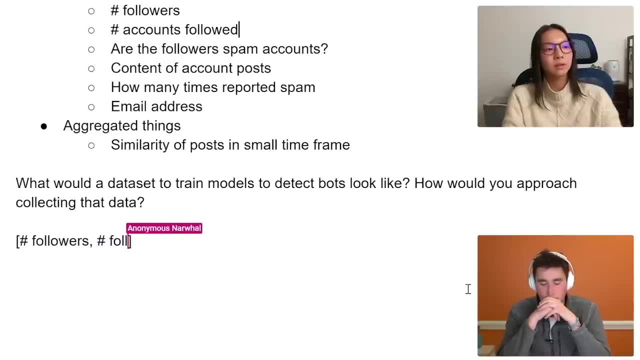 attributes. I won't mention them yet, but like a feature vector, for that might look like number of followers, number accounts you, or i guess, number following that would be a better way to describe it. those are very um, black and white numbers, right, so there's no question about whether or not we can feed that. 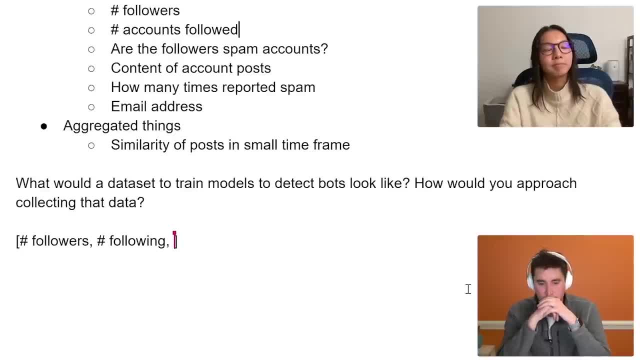 into a neural net, yeah, or some other model? um, now this next question: are the followers? spam accounts? so that's kind of this like almost circular logic, so i will maybe leave that off for now. um, the content of the account- i will come back to that- and then how many times it's reported spam. so 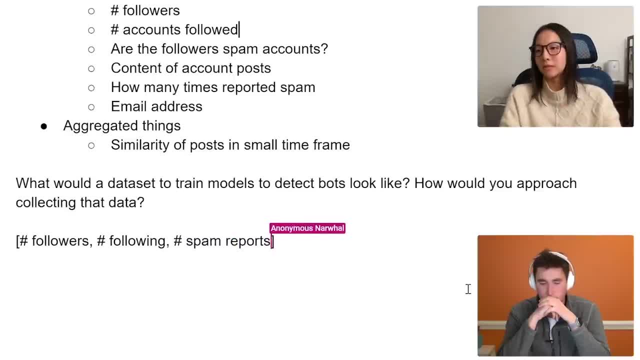 number of spam reports on this specific account. yeah, um, and then the email address. okay, so i think that this is a good start, but obviously it's not enough. so let's talk about maybe let's go with the email address first. yeah, so the thing is in here. 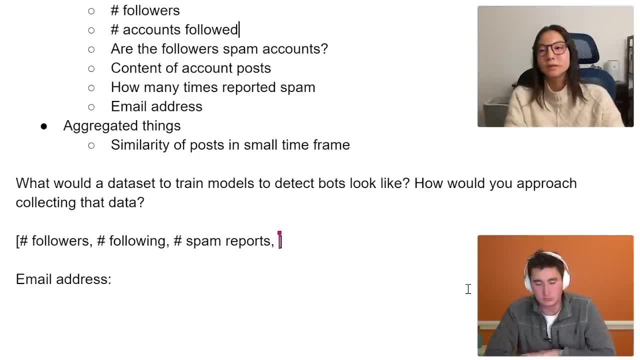 here. i would want to maybe sorry letting the sirens pass. can you hear it anymore? i can't hear it before at all. oh, really, i never heard sirens. wow, oh, okay, um, so right now we have three different things: the number of followers. number of following. 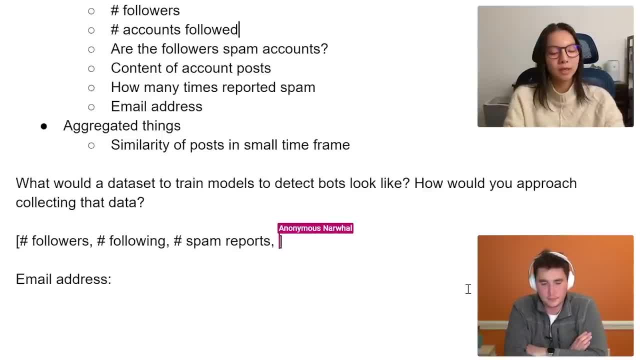 and then the number of the spam. uh بي, we have three different things in here. and then, and i think the email address is easy to use. uh, yeah, um, like what um? but some things are kind of a nous worked for it. huge number on here, right? 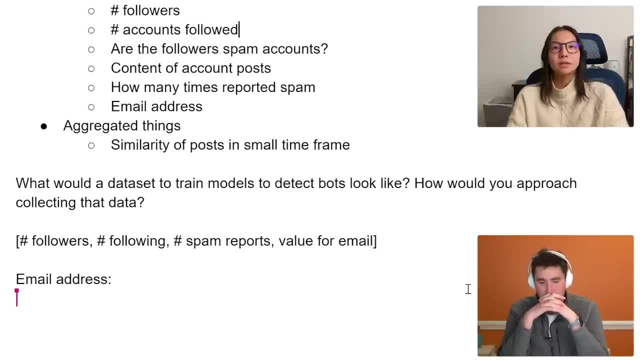 so people use what numbers? yeah đ wait, i catch something here. so um should that I? I s mean i have to domain names that, like you know, of um that are popular, that are common out there, and we would want to get you know many different countries, not just what's popular here in the us, but suppose. 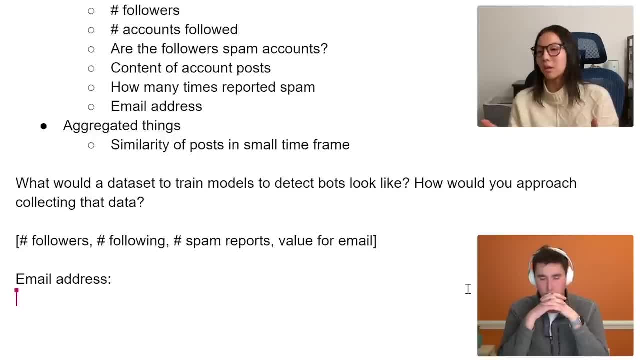 you have a bunch of like domain names that are popular, then this could be a very simple like one zero, like whether or not it has that uh opposite of prefix, that like domain name in the email address, right, so like one for uh at gmail. oh, okay, wait, oh, you can't see that. okay, but anyway, one for. 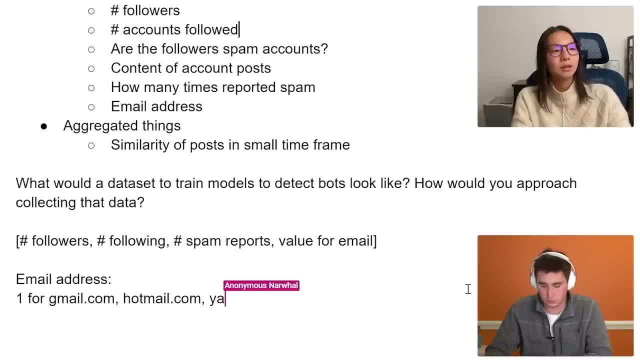 gmailcom, hotmailcom, uh, yahoocom, etc. right, um, and then zero, otherwise, yep, yep. so that would be a very basic value for email. now to get into things that are maybe something a little bit more complicated: um, we could even train a classifier on just emails, right, if we? 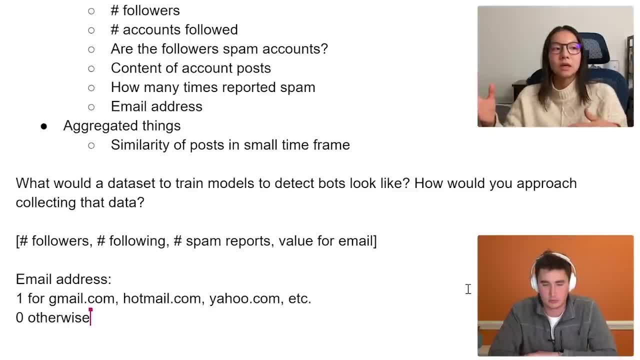 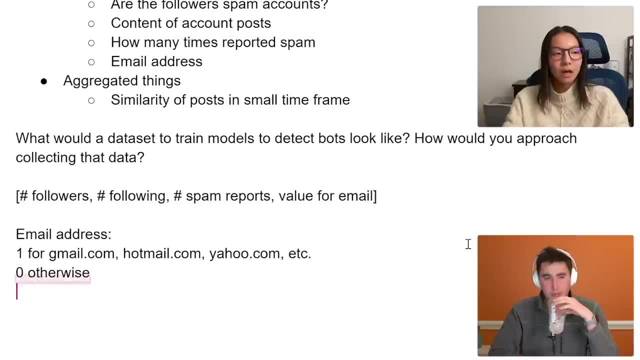 had an entire data set of emails that are, um, that are good and bad, that are, you know, not spam and spam. um, we could train a classifier on that which would spit out a probability, um, or yeah, which has been out of probability, of you know how likely it is to be spam or not spam, and 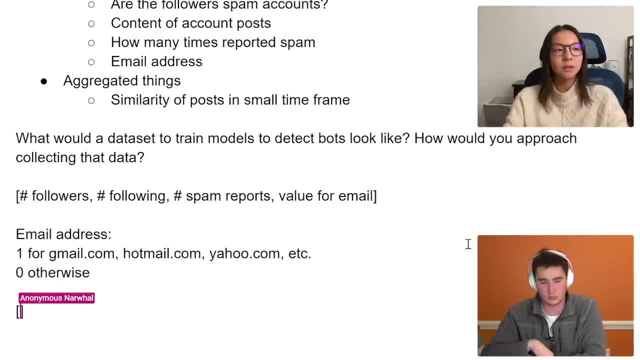 so maybe certain attributes of that email address could be, in fact, this domain name: uh, so maybe we have some sort of um one hot, uh encoding system for these. so one hot encoded uh domain name and then maybe um, um, um. can you just quickly explain what a one hot encoded domain? oh yeah, what would that would look? 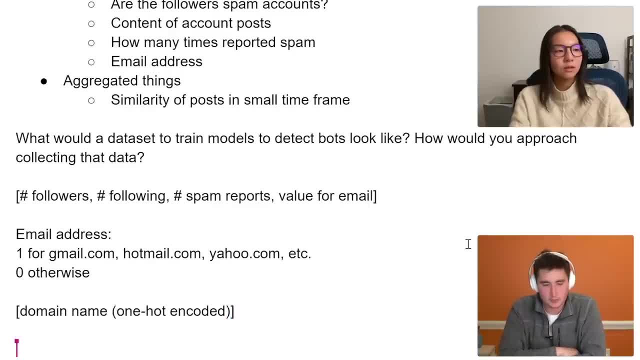 like just so clarify: yeah, yeah, yeah, so, uh, let's say that. so, basically, in one hot encoding, you are using zeros and ones to encode a certain value, and so by that, what i mean is, let's just take these three- gmail, hotmail and yahoo, yeah- and put them into like a list like this, right? so position one: 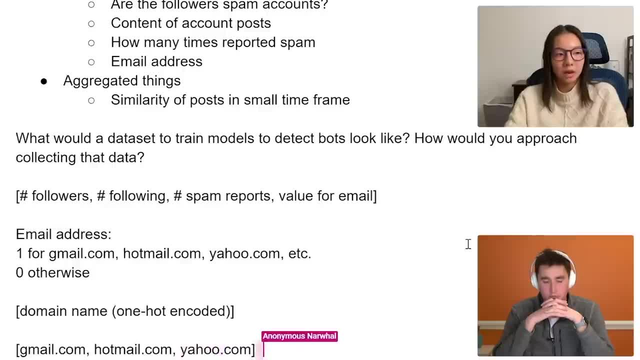 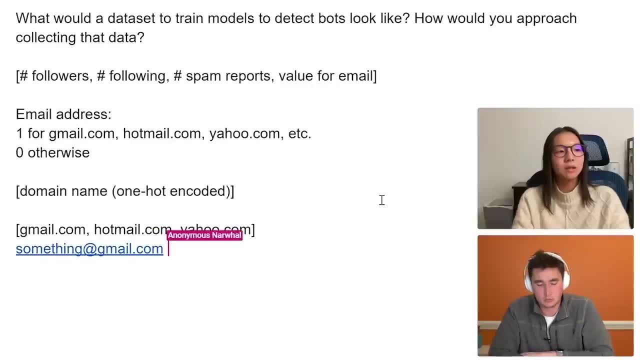 would be gmail, position two is hotmail and position three is yahoo. so one hot encoding for this, for like something at gmailcom. this email address would then be encoded as one zero, zero, then maybe something at hotmailcom would be zero, one, zero, and then something at yahoocom would be zero, zero, one. now, if i have, 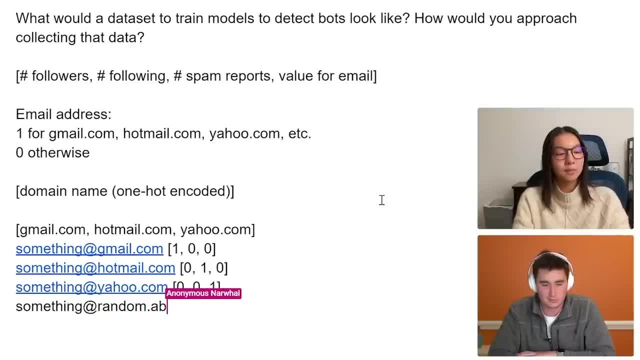 something at random, dot, ABC, then this would actually get encoded to 0, 0, 0 got it. but basically, what one hot encoding is doing is it's trying to assign a numerical value to something that is not numerical, because our computers are very good at understanding numerical values, right? yeah, it's trying to assign. 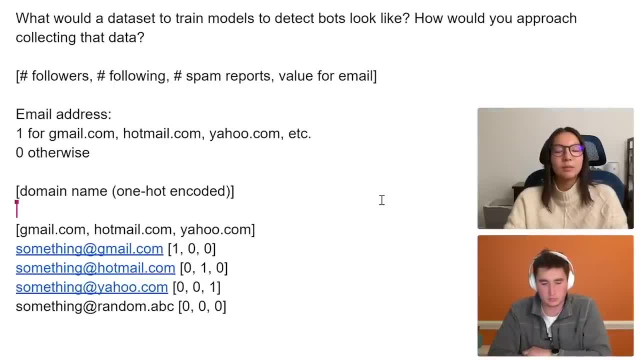 something numerical to something that is not, and it's trying to make it so. there's no association with one another. so something that you might be asking is: why can't we do one, two, three, four and just call that a day? right, that's because this is telling us: okay, one is closer to two numerically than it is to 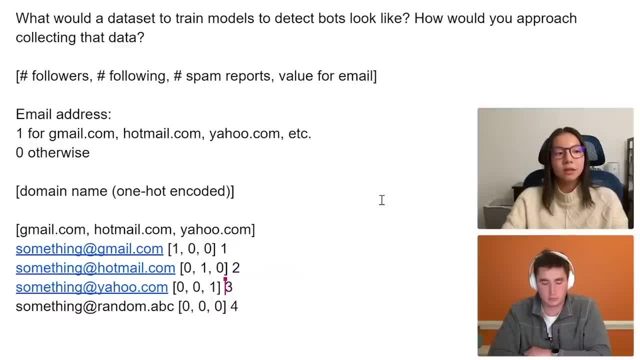 three mm-hmm. but it shouldn't matter in our case, because Gmail should not be closer to Yahoo than hotmail is to Yahoo, right, they're just different categories. they're not more similar or less similar mm-hmm. so that's why it's telling us that it's closer to two numerically than it is to. 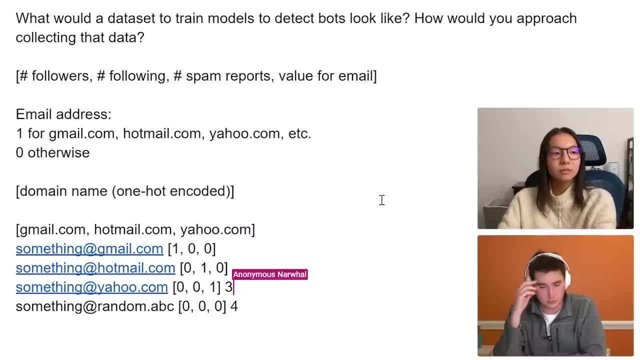 three, but it shouldn't matter in our case, because Gmail should not be closer to zero. so that's why we're using this one hot encoding, got it cool, and something else that we could do. so I do want to use, like the characters in the email itself. yeah, for this classifier I'm trying to think of, like 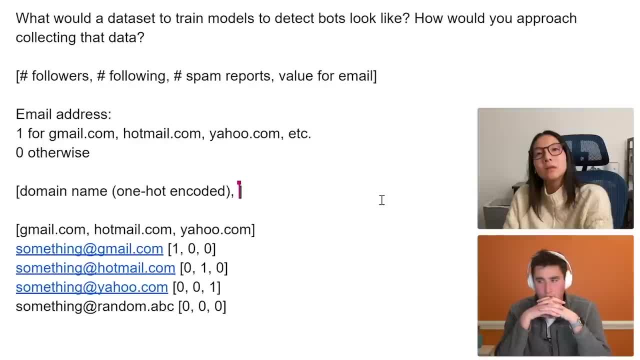 how I would do that. I might well. so I do think that if there's a name or a, a word in the email, it's probably more likely to not be spam, Yeah Right. So I think that maybe like having a list of common names and common 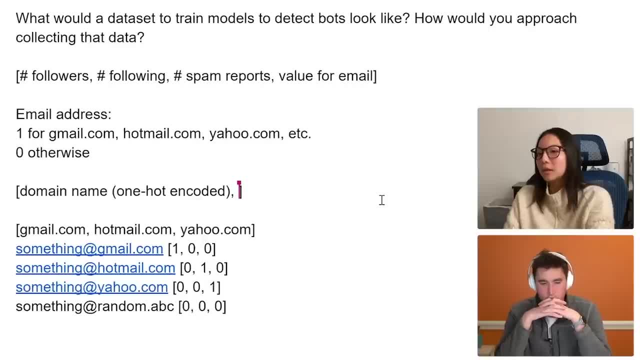 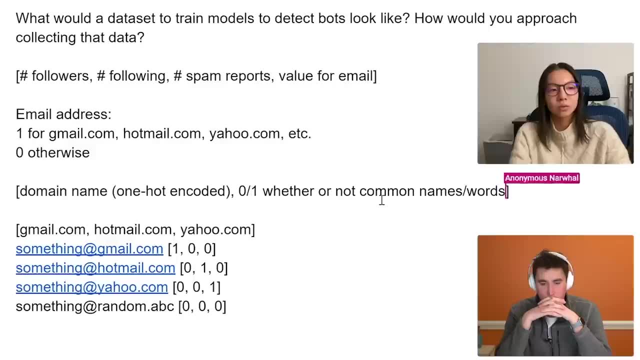 common words. Yeah, that we could check that against. So that could just be like a 01 binary encoding for whether or not common names or words appear in email. And I think this one's also kind of tricky because I do think that you have to consider different languages. 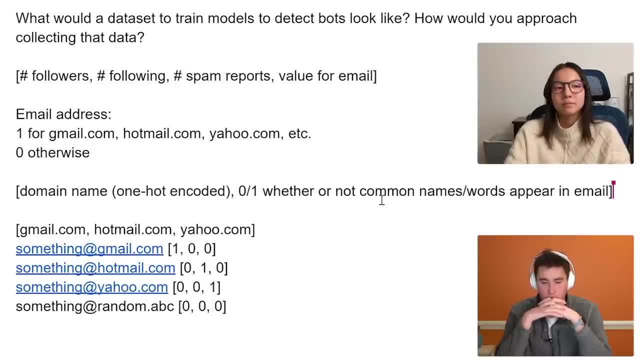 Right, And and so this- this would be something to think about. if we were actually building this model- is like we would think about the different languages and different names and different languages and stuff like that. So for now, what I might do is just this simple encoding. 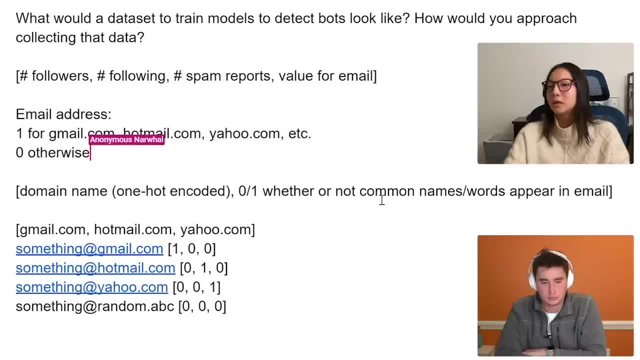 scale. I think that would be enough for us to be able to get a bunch of common address domains and then zero or one for that. I think that would suffice for now. Yeah, Now, in terms of this. Now let's go back to this like content that the account is posting. 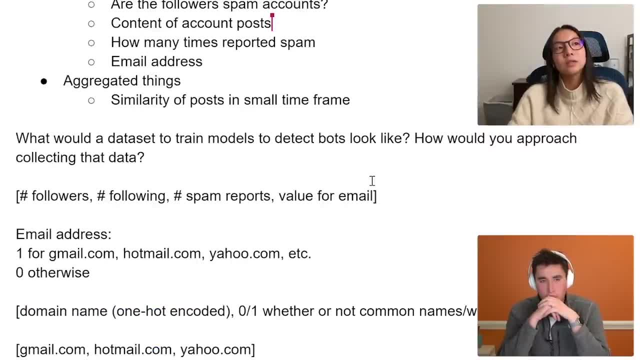 So I do think it makes sense to not scrape the entire like post history of the account, because I think that would that might be excessive. Like I think if it's a true spam account, then like the first five or ten should suffice. 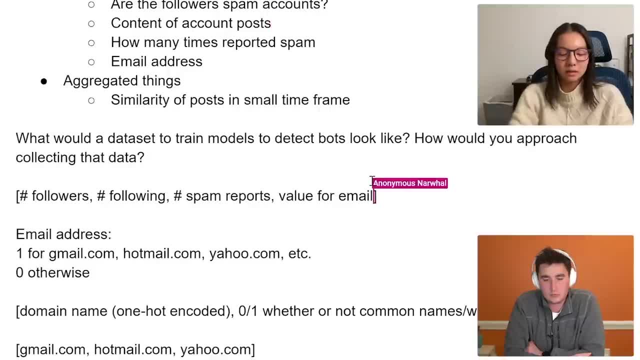 Right. So I think what we could do is, in here, have certain features for, like post number one, post number two, et cetera, to post number. Let's say we do ten, Yep. And now, scrolling down a little bit, 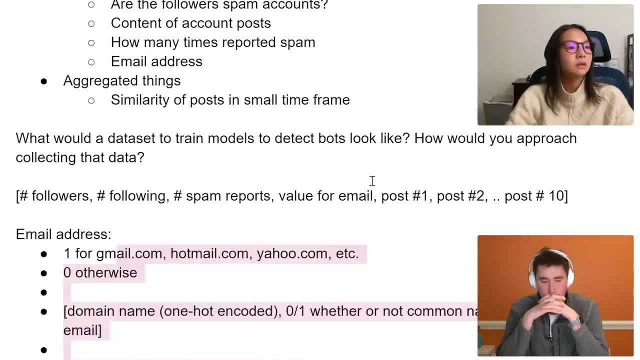 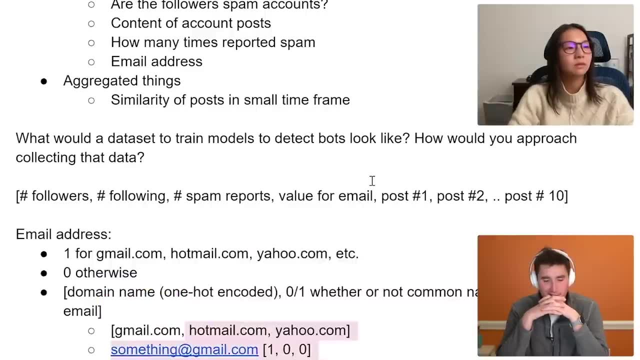 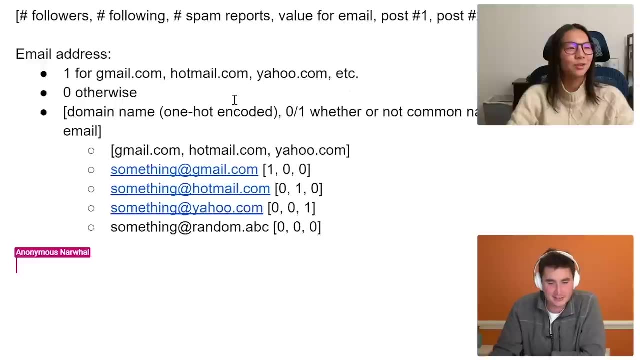 let me indent all of this. Why did it make a bullet list? or was it a bullet list? I guess some of it was No, but I made it. I did that Nice Yeah, Just for organization. Yeah, I appreciate organization. 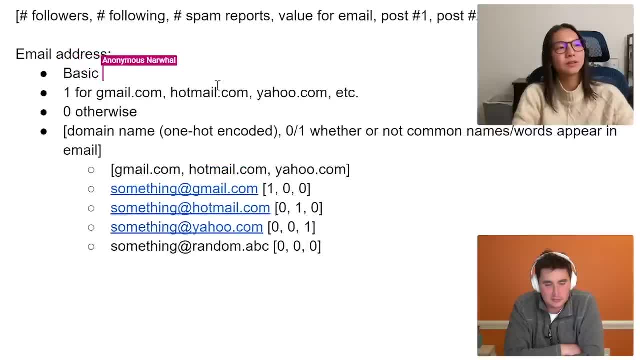 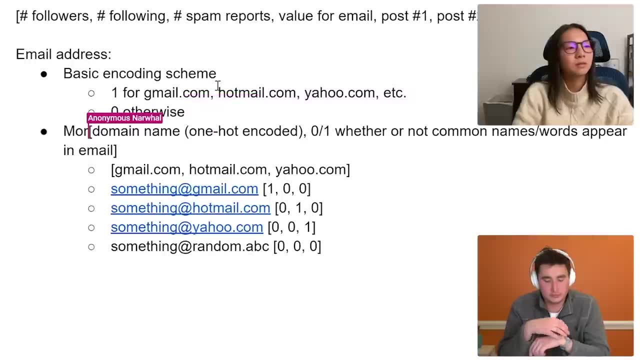 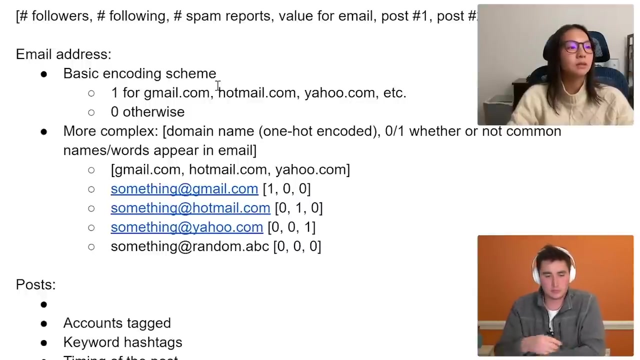 Yeah, Here. So this is basic encoding scene. Something more complex? Yeah, This would be this. Okay, So now let's think about the posts. So with the posts, that would be a lot of this stuff from up here which I'm just going to copy and paste down here. 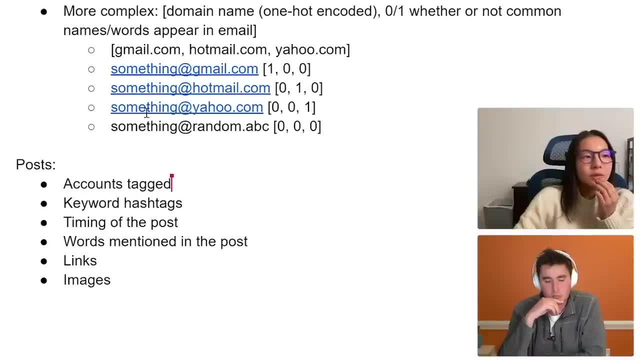 Okay, So the first one could be accounts tag. Okay, What are the simple ones? The simple ones are things such as: how many times number of spam Reports for that specific post? Yep, Um, maybe Okay The time timing of posts. I think that can be easily converted to like an epoch value or something. And the only reason why I want to consider the timing of the post is because if, for example, the last ten posts were posted within like one second of each other, Yeah. 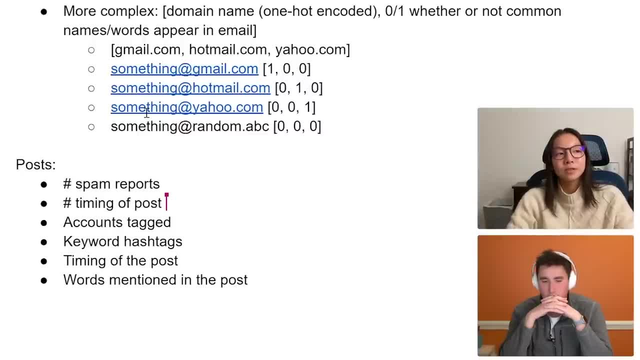 that probably indicates a spam bot, right, Um? so that's the only reason why I want to consider this timing, And I think that it would make sense to maybe use some sort of integer representation, So maybe like seconds or milliseconds since epoch. 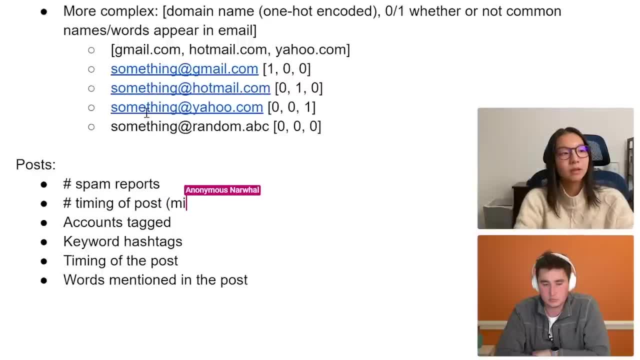 Mm-Hmm, Um, like So, yeah, Uh. and then next I would think about: And just just because you know, with our team we have to communicate these things to, you know, business stakeholders that sometimes don't understand some of these details. 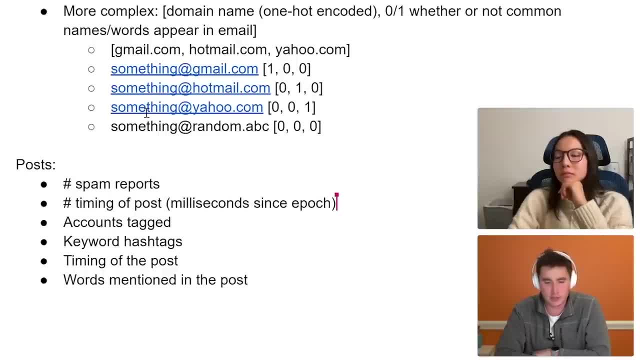 Can you just kind of a very, I guess, simple terms. What is it mean? milliseconds since epoch? It literally means number of milliseconds since, like I think, it's January 1st at midnight in 1970 or something like that. 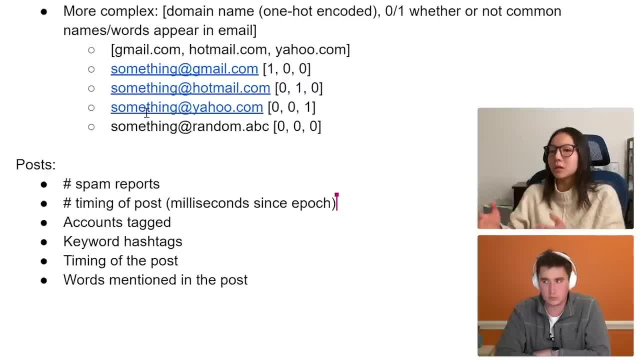 But you can think of it as literally just like number of seconds or number of milliseconds since a certain time period, like 30, no 50. Oh man, 50 years ago, Yeah, Um, yeah. So it's basically a discrete discretizing time such that we can measure it as an integer. 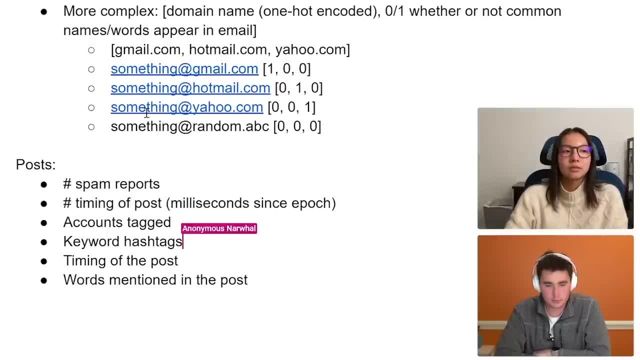 Yep, Okay. So then next, I think we have to think about all these tags and the content In the post, Right? I do think that one easy thing to do could be like for the words mentioned in the post to have some sort of 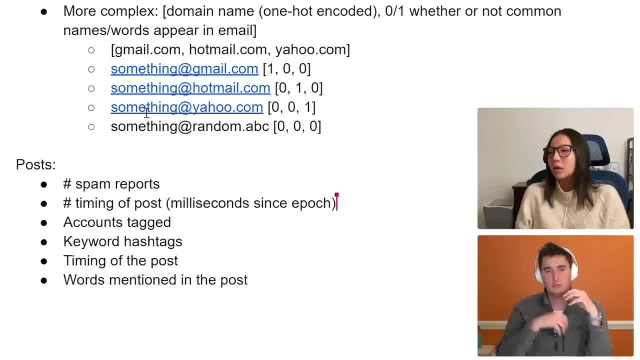 again like one hot encoding for very common spam words, Yeah, So, such as like: claim free- I can't think of all the ones off the top of my head, but yeah, yeah, I'm not. I'm not a spam bot, but that's good. 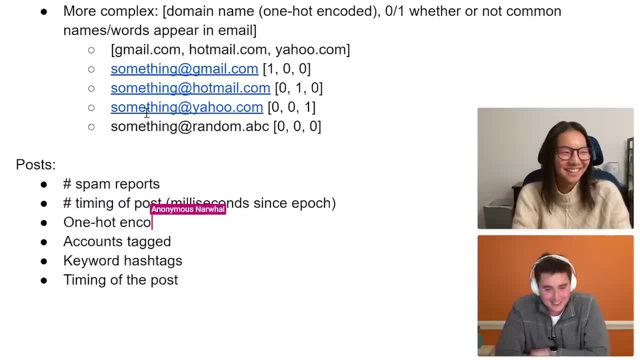 That's good. We're not hiring spam bots right now, So, yeah, So maybe like a one hot encoding of common spam words, Cool, And I think that maybe this could also be similar for like the hashtags as well. But I think that this could. 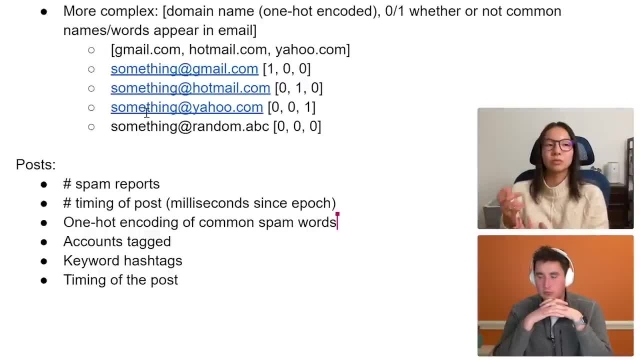 Encompass the hashtag, right? Because if we're just looking for whether or not these words appear in the entire string of of words, then like that would cover the hashtags as well. Cool, And I think honestly. I'm just looking at the time here. 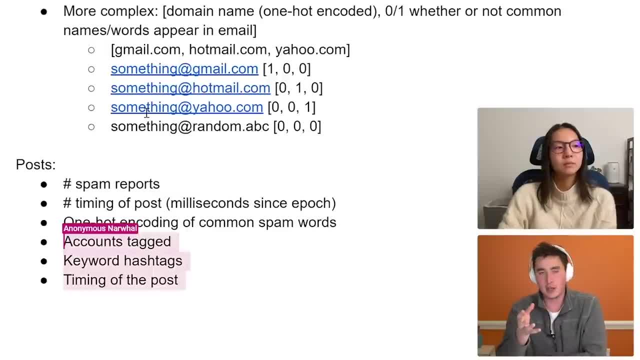 I, I do want to kind of switch gears a bit. I think this is a good, you know, high level description of an implementation. Um, I do want to just ask some kind of follow up questions to these things. Yeah, So I guess, just circling back first, I think that really you dove into the details of 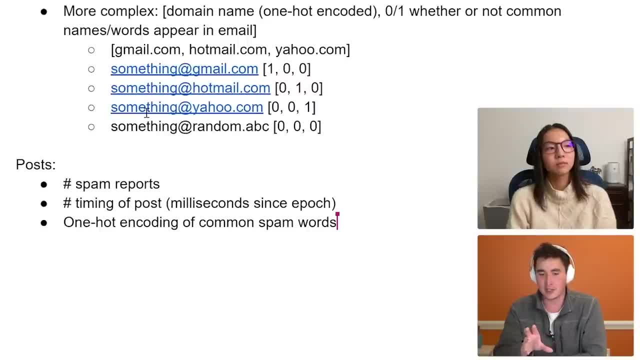 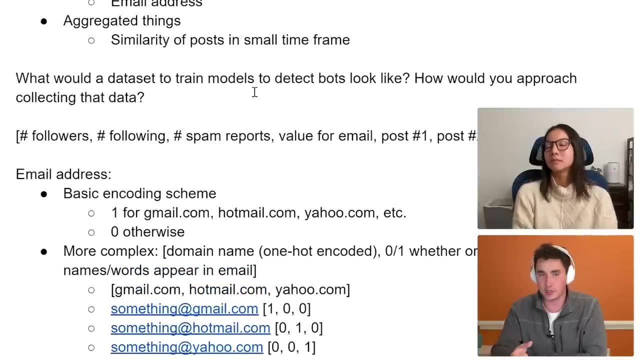 Implementation. I think that this is a solid approach, using this feature vectorization approach and, kind of you know, I think you did a good job explaining some of these details, but I do want to revisit, Kind of the uh, one of the initial questions, which was: you know, we have this way of building this model with these feature vectors, but you know, at the end of the day, we need to train these models and we need a data set to train these on. 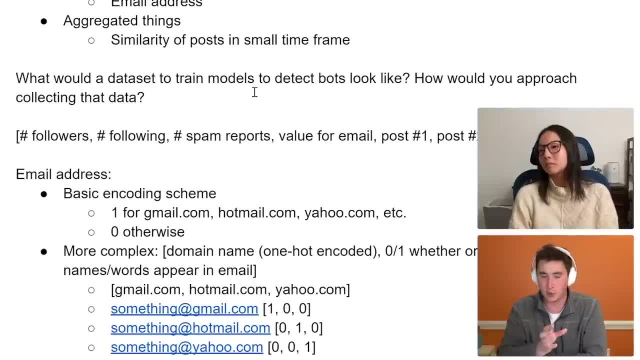 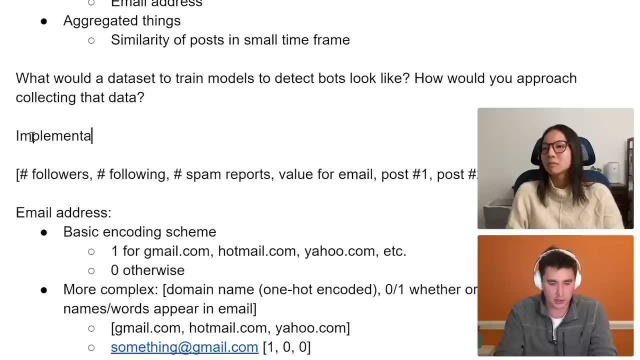 So I guess I just really want to drill down specifically on that. Like what would the data set that we need to Use? this approach maybe look like and just any I guess thoughts on that And I'm going to just break this apart real quick and just say um, implementation approach or something like that, just to separate it a little bit visually. 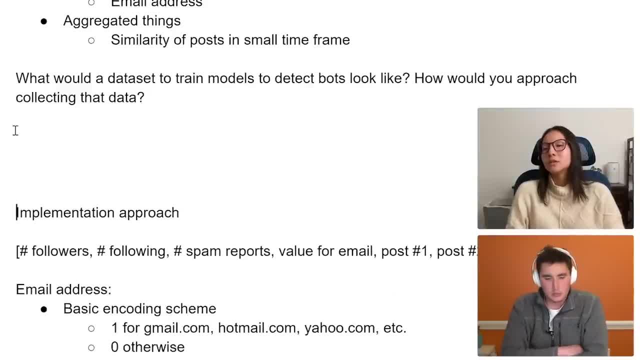 Does that make sense? What I'm asking, Yeah, So you're just asking, like, how would I collect that data? Yeah, The data that I just described. Well, I guess what I'm thinking about is the data you just described. I think is fairly straightforward to collect, but at the end of the day, we need a 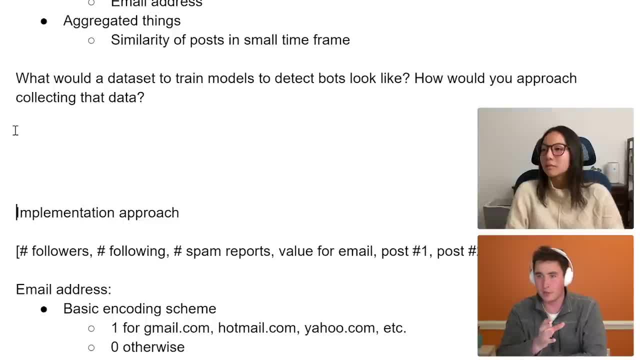 I guess the two questions I want to drill down on is what makes an account a human and what makes an account a bot Like. how do you, I guess, get data on bot accounts and bot and maybe human accounts Like cause? at the end of the day, we need that to make this a meaningful model. 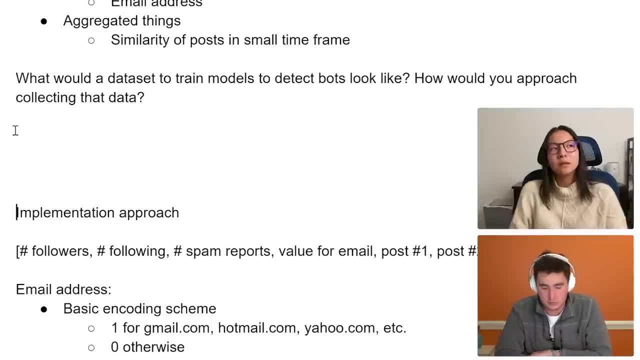 Right, So I do think that, um, well, okay. So at the end of the day, who is the person who can distinguish the Bots? right, It's humans. It's humans because when we get annoyed at seeing spam or something like that, like that's when, that's, that's what makes, that's what literally makes this a spam post. 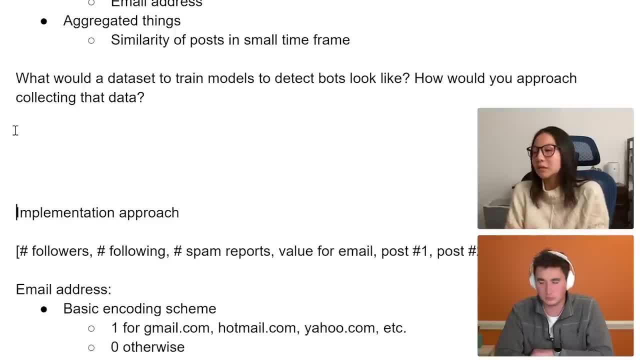 It's when some human it decides: I don't want to see this content and this is spam. So I actually think that one of these things that I kept mentioning, which was how many times has this been reported spam- I actually think that that could be our label. 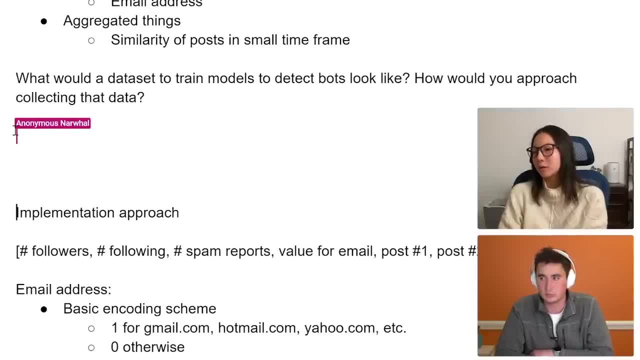 Right For whether or not the account is spam or not. Yeah, So, um, this, this is how we can label spam, because, at the end of the day, this is a. this is a classification problem, It's: is it spam or is it not spam? 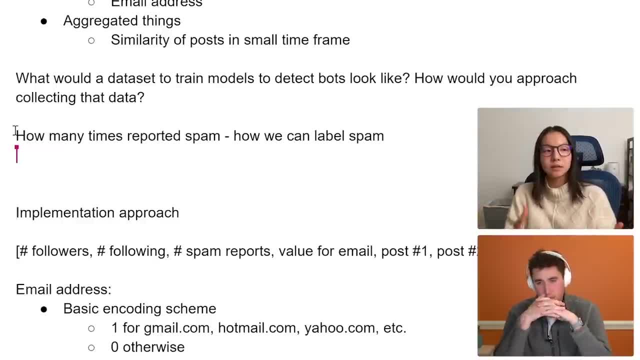 Um, and what our data is collecting is: we're collecting all of these features, but then we need a label for that feature. Right, And that label. we want two different categories. Is it spam or is it not spam? Yeah, Um, and obviously, the more times something has been reported spam, the more likely it is to be under category one. 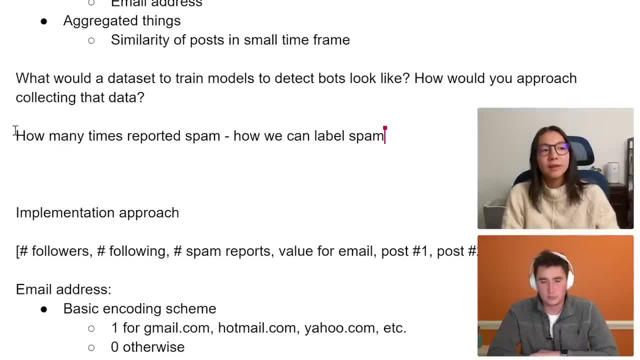 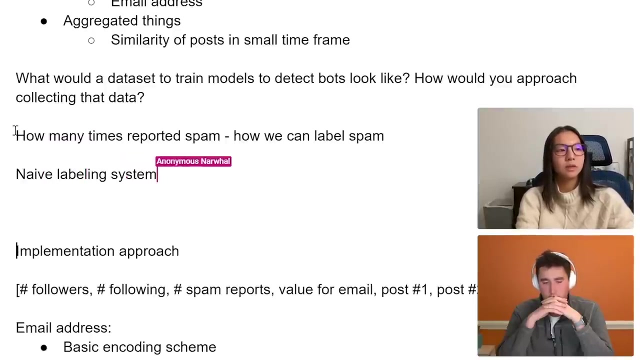 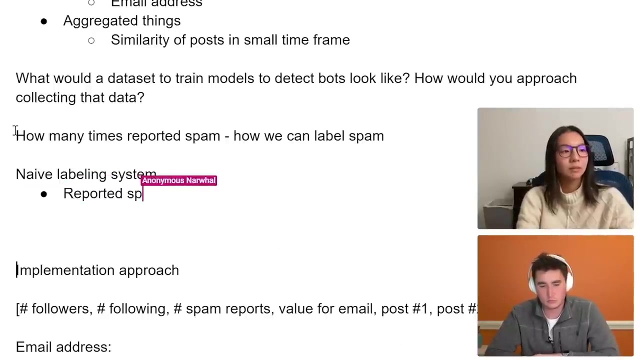 Yeah, Right. So I think one of the most basic ways to do this uh could just be: if it's reported spam over blank number of times, then make that Like, then label that as spam. So naive labeling system could be: if it's uh reported spam X number of times, then label spam. 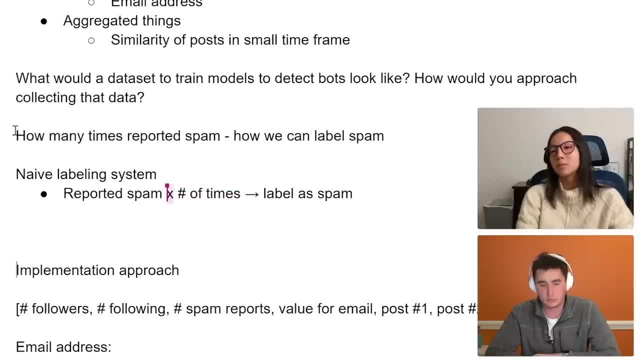 Um, and this X, this is really up to like what you're like Like how much data do you want to collect? Right, Because you don't really want to kind of fake that data, because you know, as I was trying to come up with these things down here, 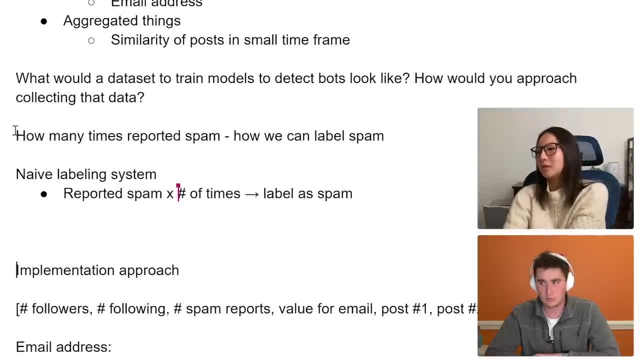 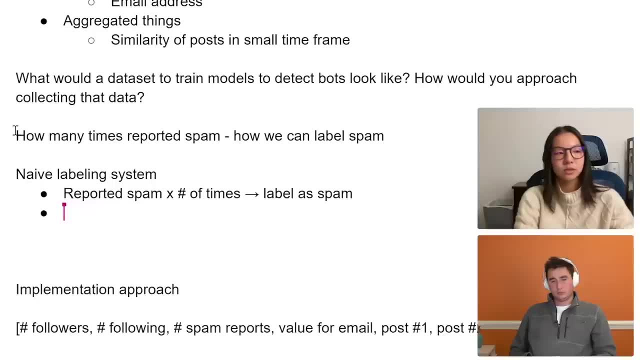 it's. it's pretty hard to fake being spam if you're not spam yourself. Yeah, Um, and then for the non-spam, I would just do like: if no reports of spam, then, uh, label as not spam. 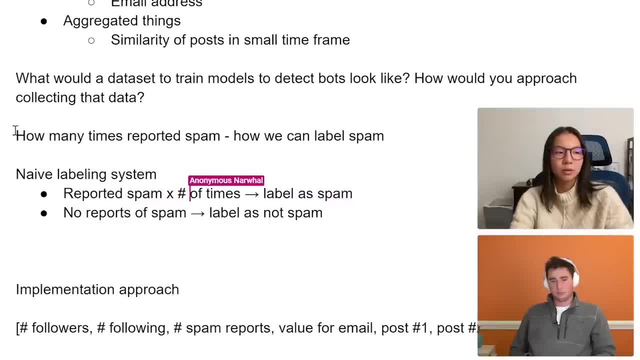 And also I think that these no reports and this report spam, Like I think that you should put some sort of time frame on this, So like since account creation, uh, for longer than a week, or something like that, if it's never been reported spam or if it has been reported spam. 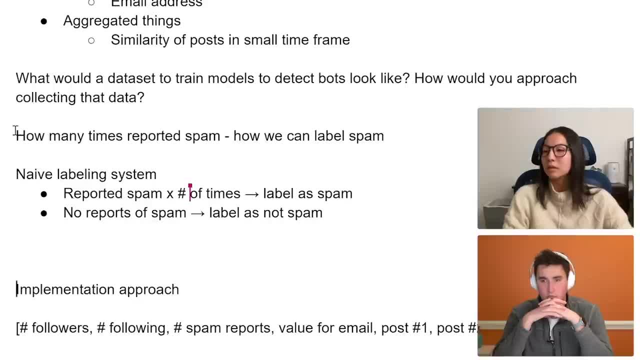 then I think that can give you a good um indication. or maybe not a week. You would have to set the threshold right. Yeah, But you don't want like a brand new account to be part of this system? Definitely makes sense. 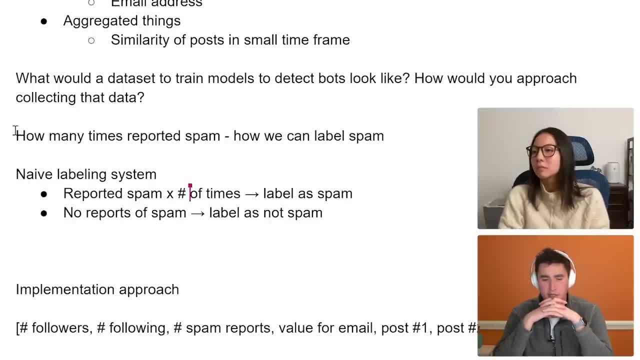 Okay, I, I, you know, I think this makes sense as a naive labeling system. You know, my big concern is here is like: I guess, what are the problems potentially with this approach? Like you know, how could we build this, make this more robust? 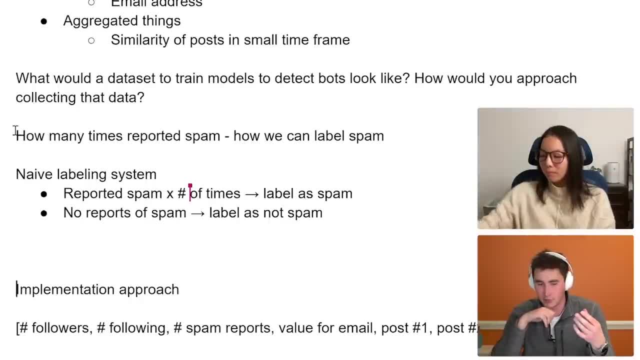 I guess either you know, maybe identify what could potentially be a problem here, or potentially just mention an idea or two about how could we make this more robust. Yeah, So I definitely think that, But this is relying a lot on user feedback, right? 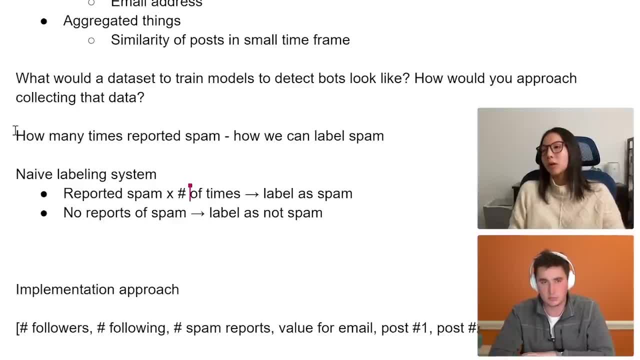 It's relying a lot on whether or not somebody has reported something as spam. Yeah, Um, I do think like I mean: okay, so one slow but sure way that you could label, uh, certain things as spam or not spam is that you could just have like, like you could just hire people. 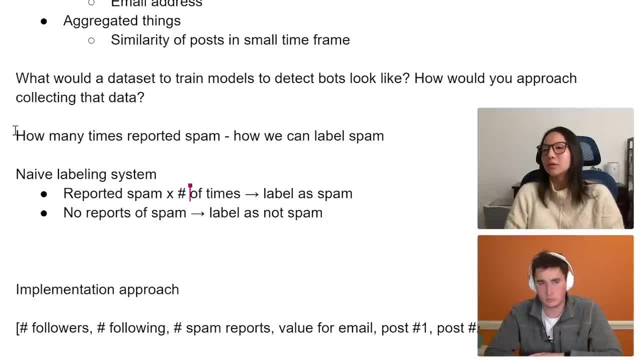 Yeah, To go through different posts and different accounts and say, oh, this one is spam, Like we should use this as um a spam account to model, to model after or to include our data set. Sorry, but that would then be also kind of tedious, slow. 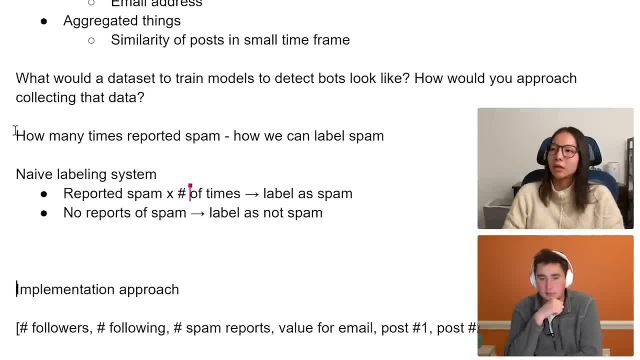 Um, you would have to pay more just to collect data that you already have. Um, another system might be: Hmm, Um, sorry, let me think for a second, No problem. So I really I I do think that this late, like this reporting spam, is a good indication, because it's similar to how, like, Waze works. 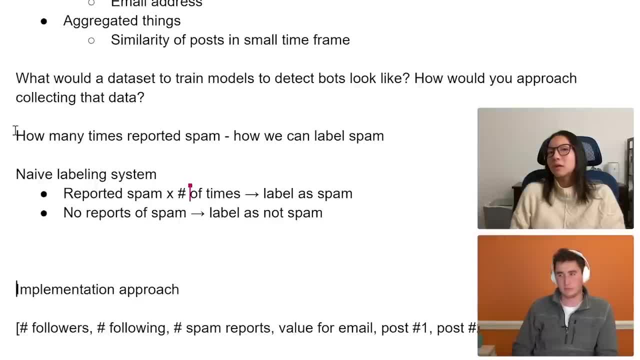 Yeah, Right, How like? oh, is there? Well, okay, One thing that you could do is you Could just implement something that makes it more incentivized for user to correctly label things as spam or not, Um. so, for example, uh, you could have a larger, an easier system of reporting spam or um, you could have literally a direct question of whether or not something is spam or not. 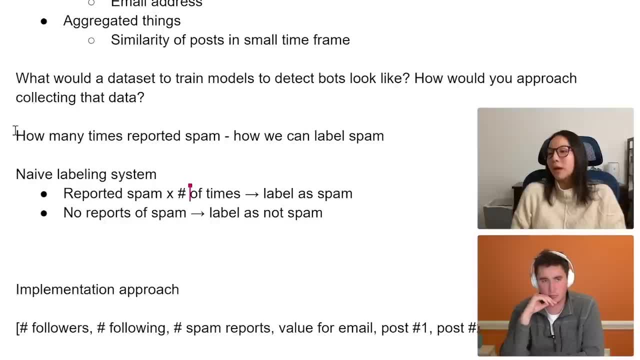 Yeah, Um, because I do think user feedback is Is probably one of the most important cuz. after all, you're building a product for your users, right? Yeah, And like their feedback, their classification of whether or not something is spam or not. that's gonna be what's important. 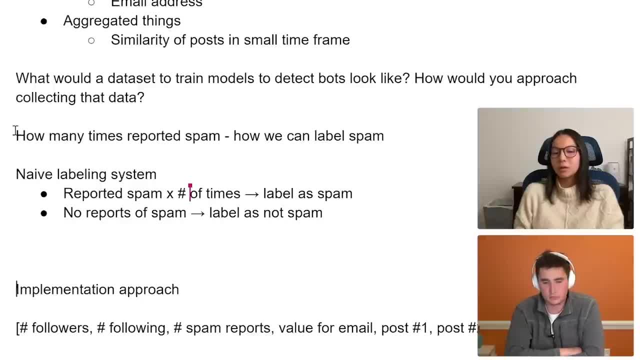 Um, so maybe, like, if there's some like, maybe we can start tracking some of these things and just coming up with something naive, like things that are obvious as spam accounts, Um, if those specific attributes pop up, then we could automatically just be like: oh, do we think that this would be spam? 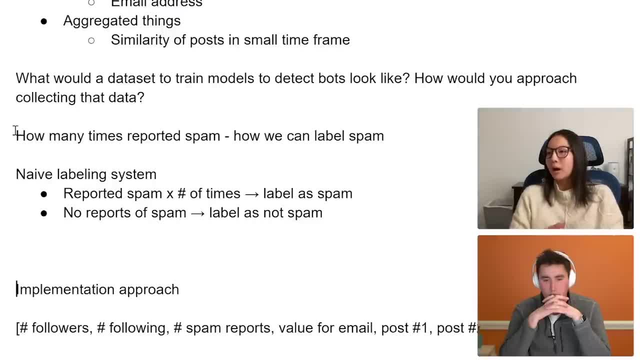 Like you could have a poll that presents to the the user, that would make it easier to label a spam or not. Yeah, Um, I think I think that that suffices. That kind of answers my question. I think the only details that I would add for my end here is that you gotta keep in mind that there's a lot of things that you can do. 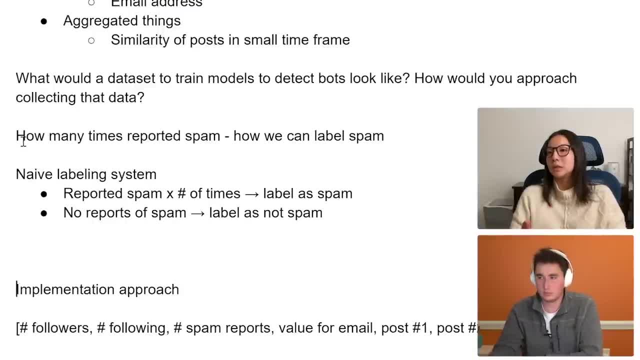 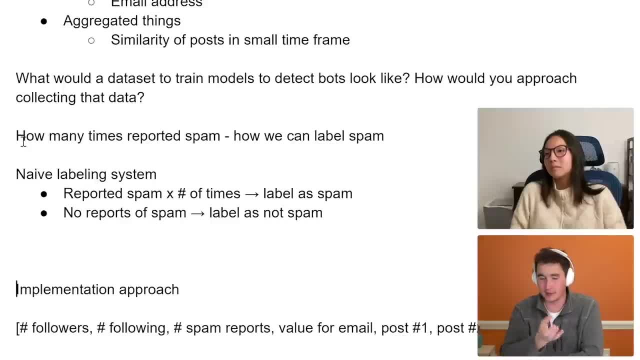 Yeah, a lot of people, Yeah, that are bad actors. Yeah, and when we're designing a system like this, we need to keep that in mind. There might be targeted attacks, people labeling Right something they don't like as spam. 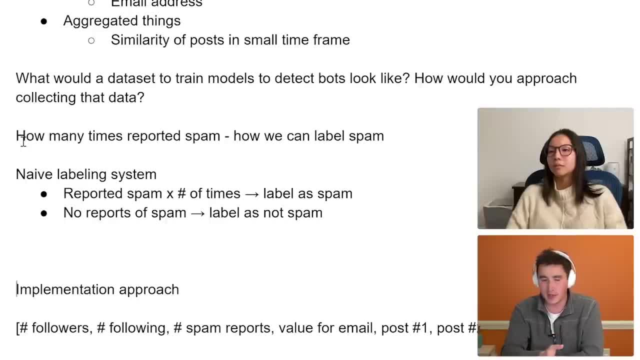 Right, So we also need to factor that in, And so that would be one component, right, I would add here: Right, Yeah. Another thing I would just Yeah, Am slowly mention to is: I: I don't think it's actually a bad thing to do a little bit of human annotation. 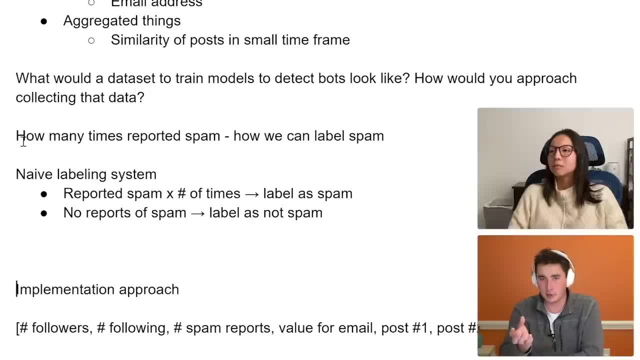 Yeah, I think a lot of Yeah you know, Yeah, tasks, Yeah, sometimes require that. I think the important thing is, Yeah, be paying a group. we might not be monitoring them super closely, so we want to make sure that they. 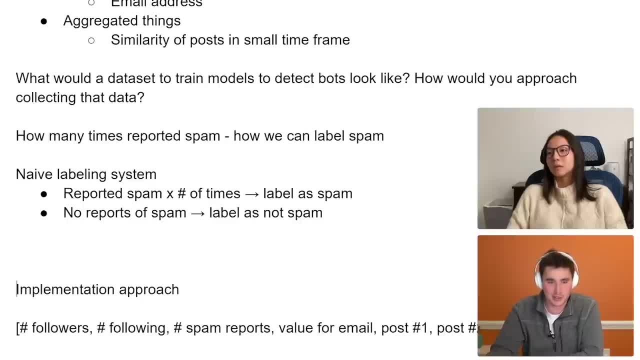 are not just ticking a random box, so you know something to think about there, right, cool. well, i also do want to add. one more thing to this is like maybe your threshold should not be like number of times, but maybe should be like ratio of, like spam reports to engagement, or something like. 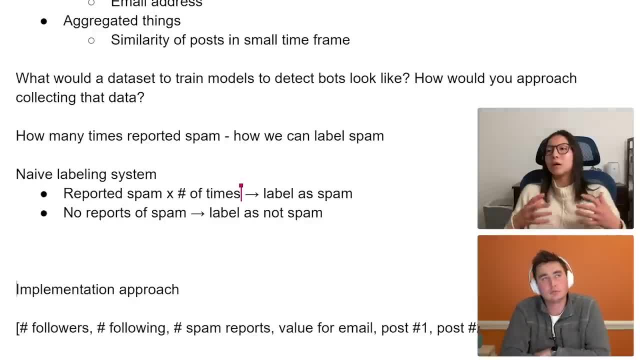 that right, yeah, um, because even if there are many bad actors, i do think that most people, uh, would act the way that you, yeah, would think that they act. so i think, like there can't, there probably aren't more than like 10 or 20 percent like people who would deviate from that expectation. 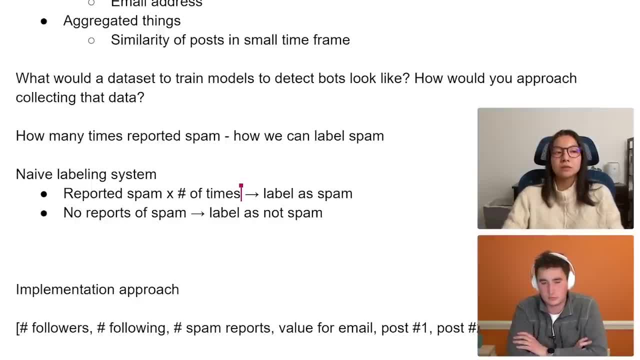 so, for example, if, like, i think that's that's the importance of this threshold, right, that's importance of saying, well, how strict do i want to be, such that, um, like, do i want the the stricter i am with this threshold, the more confident i am that this. 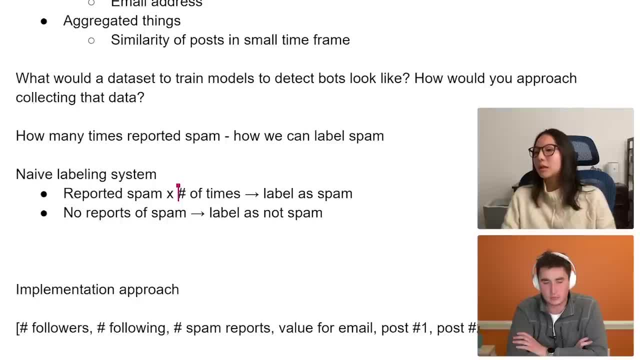 has to be spam. yeah, right, and so that's that's. the importance of this labeling system is: how strict do you want to be, because the stricter you are, the less data you have to train on is another consideration. yeah, okay that, yeah, that makes sense, and i i think that that ratio idea is. 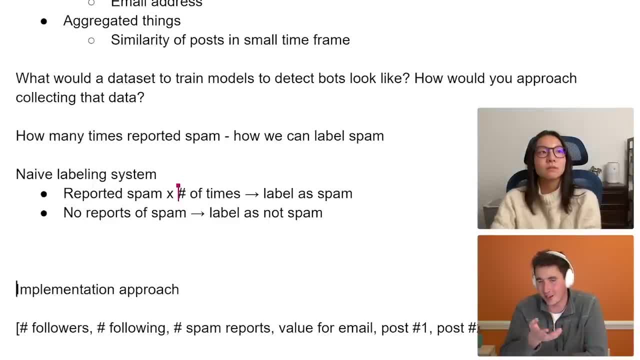 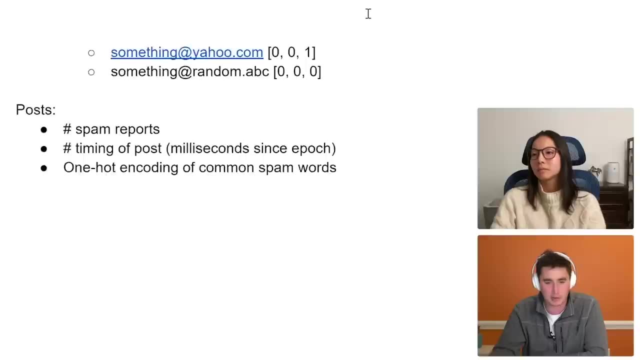 an interesting idea and, you know, the only really way to know is to actually try this out, test it. so it's hard to know with certainty, but i think the important thing is having these different ideas that are worth playing around with and attempting. okay, i'm going to ask one. just because we're running up on time, i'm going to ask, i think, maybe just one. 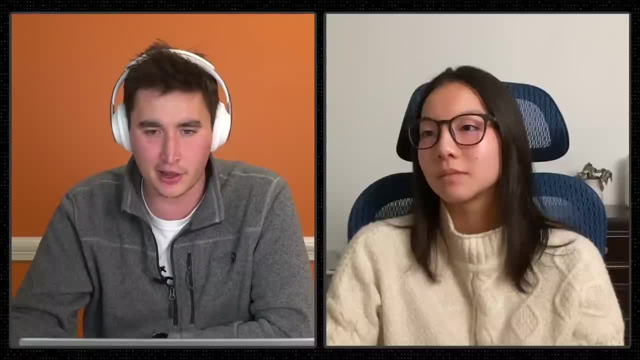 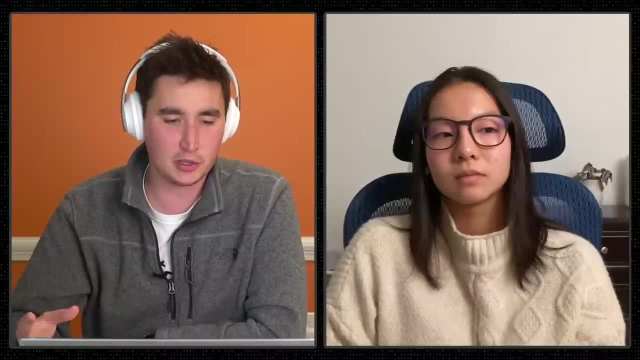 last question on this problem. i'm going to stop sharing the screen. you don't have to use the document anymore. we can kind of just chat about this. i'm just, you know, from a. you know, let's start thinking a little bit more about implementation of this. um, you know, thinking about 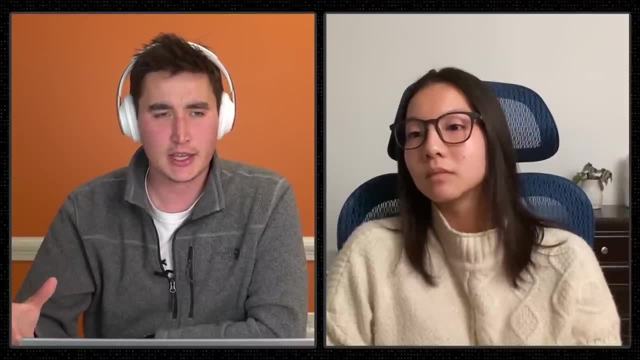 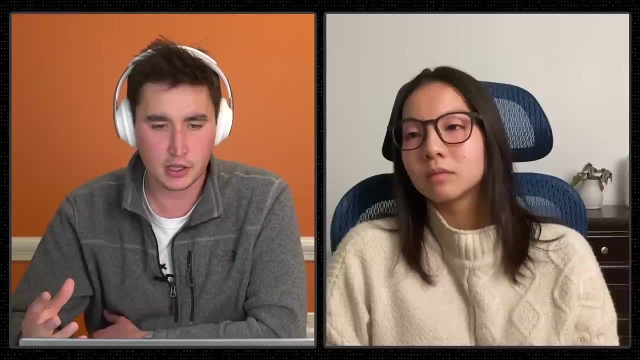 python and maybe the larger cloud ecosystem. like you kind of have a high level feel of how you might approach the actual technical implementation of this, and i think that's a really good question. you know, building this model or anything that keeps comes in mind, so maybe certain libraries. 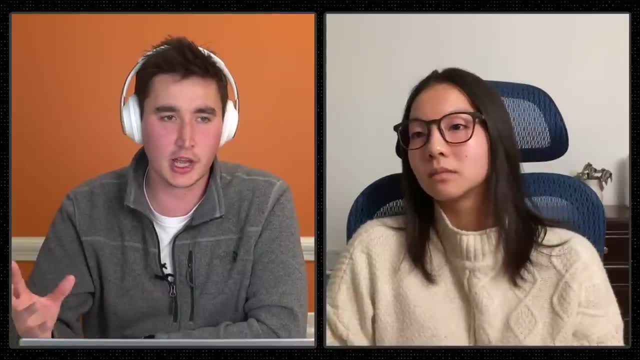 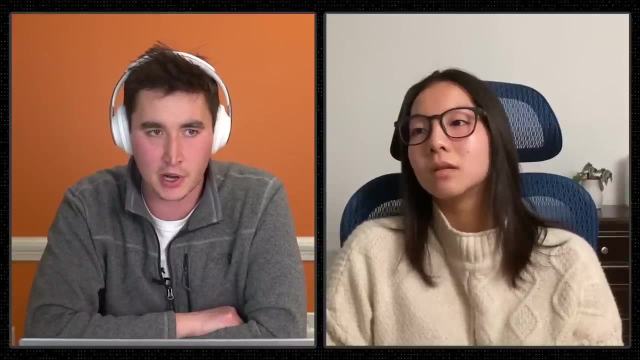 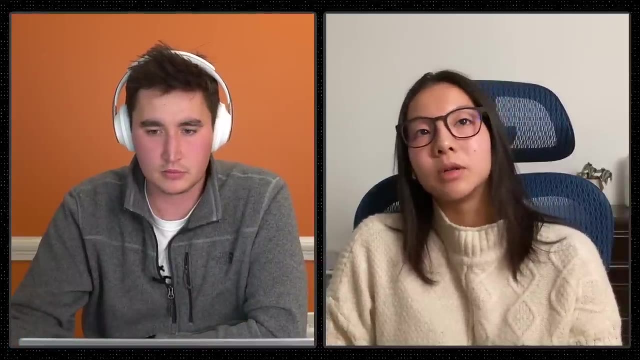 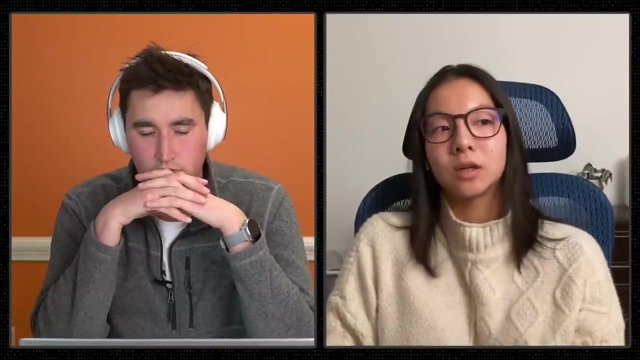 certain uh frameworks, certain just like cloud resources, etc. i'm just curious, you know, from a implementation standpoint, anything that kind of sticks out that you know you'd probably do from an approach? yeah, so i would definitely say i'm probably the most familiar with like tensorflow, so a lot of um. how i would be modeling this is i would probably start with my data. 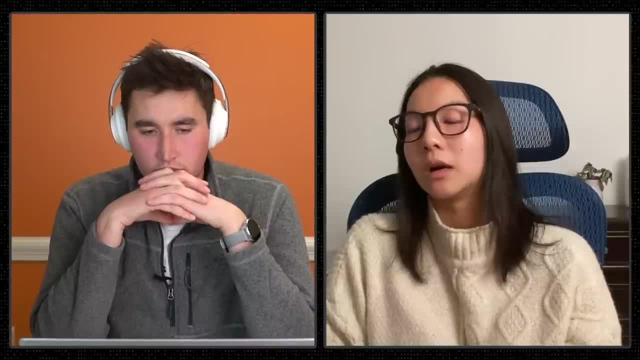 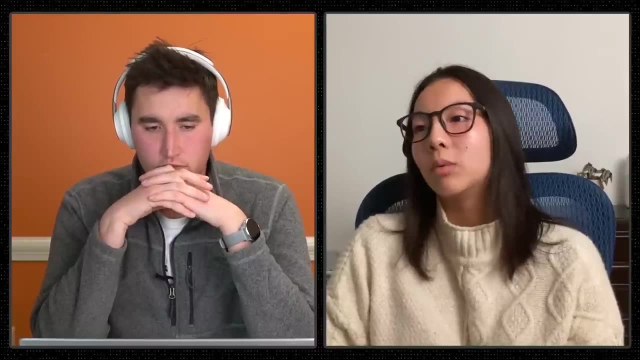 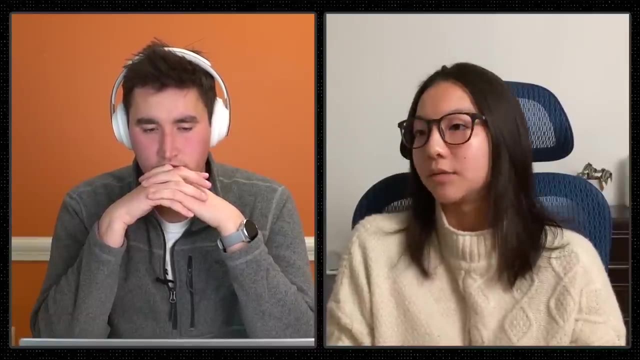 set and then i would probably go into like a jupiter notebook or, um, a collab notebook and i would try to mess around with it just to see you know what. what is the simplest model that i can make to have some sort of- okayish, um, classification rate, right, and a few things that you could use in. 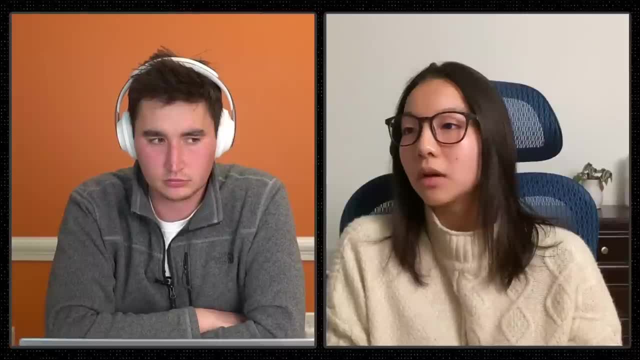 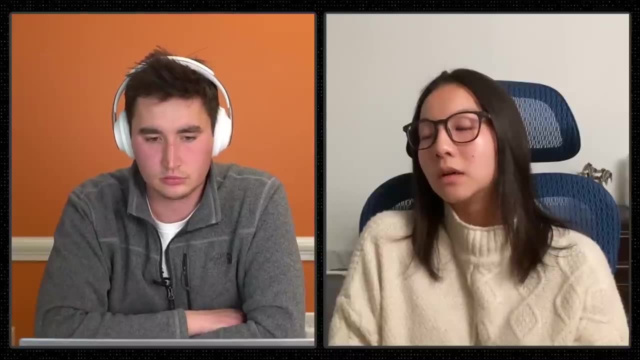 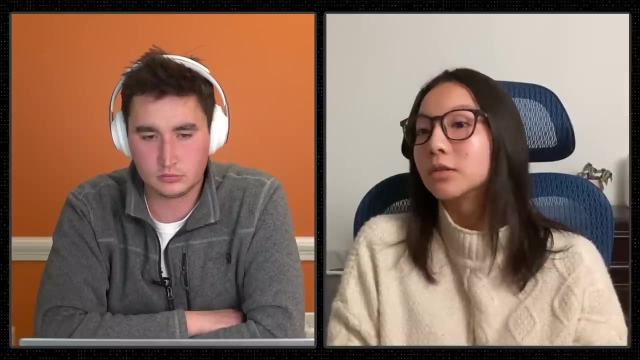 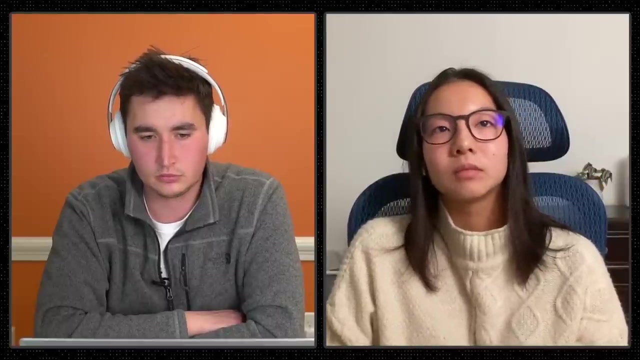 order to figure out how well your model is training, like it depends on how important to you falls positives or false. negatives are right, um and like, more so than accuracy, like i think those are things that you should be looking at and also i think that, um, yeah, anyway, sorry to get back to 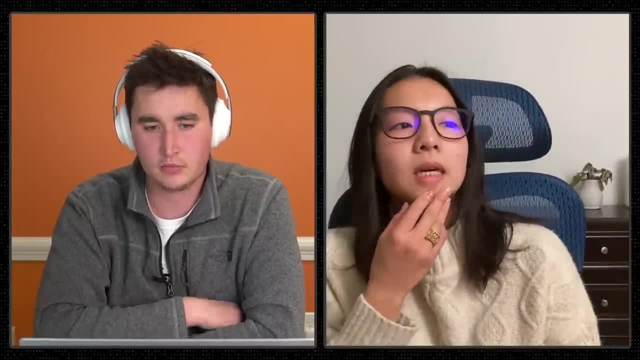 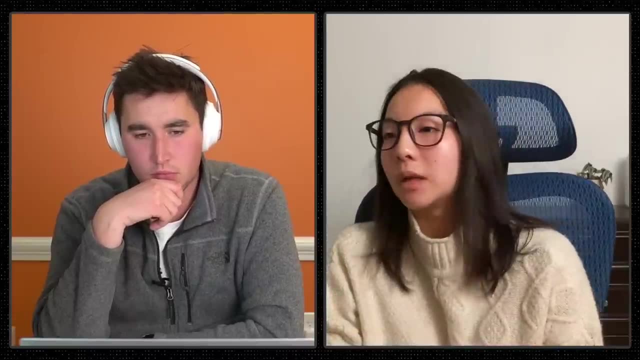 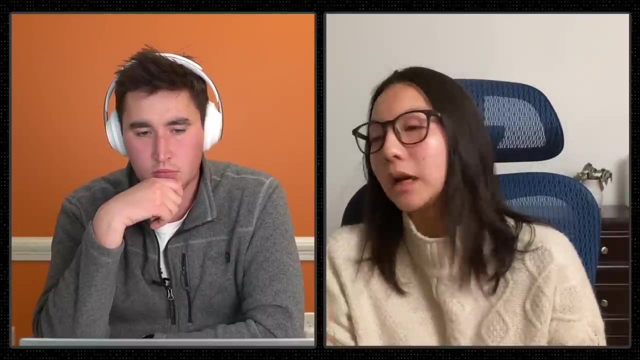 your original question is: that's how i would start this- and then, in order to deploy this- i'm actually not that familiar with deploying, uh, certain models, but i would assume that you use some sort of like gpu to accelerate the training and then um, or yeah, sorry, this is during still the training phase, but 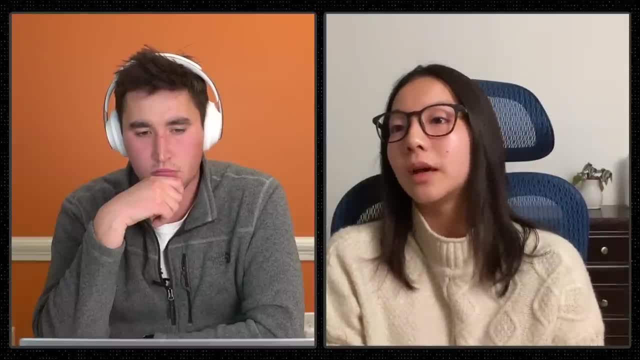 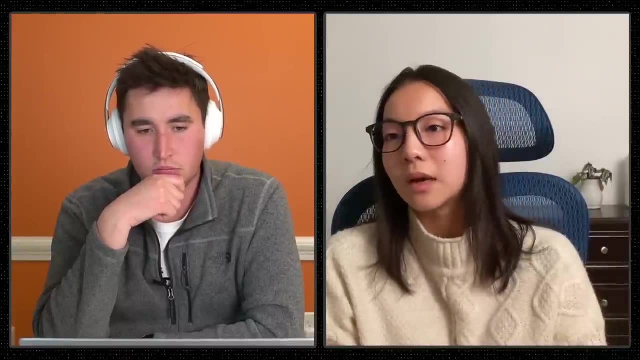 maybe you're training a much larger model than the initial one that we came up with in our notebooks. yeah, so you would use, like gpu, some other resources to train it. to accelerate that training process, you would parallelize um and then, when you actually deploy it, i mean, 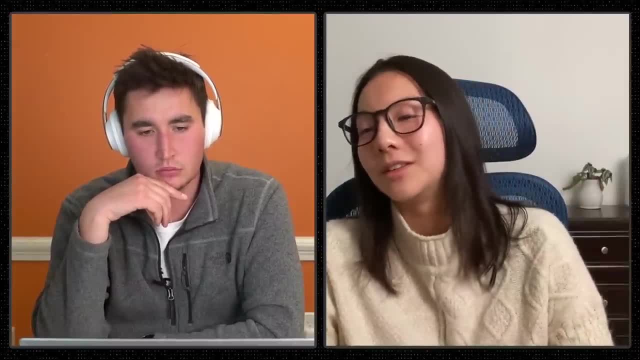 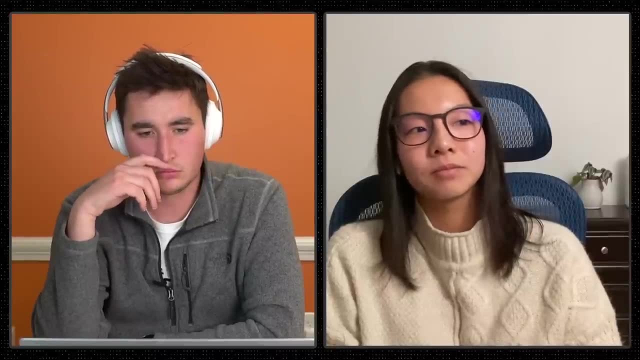 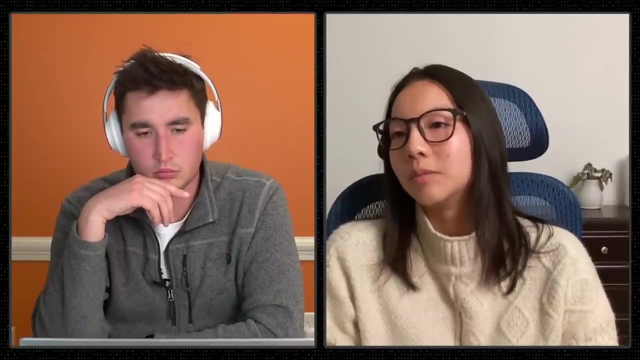 everybody uses like cloud technology these days, so i i feel like i would just deploy it to some cloud that serves the model and um, and every single time we have a new post, we can just filter it through: or not a new post, but maybe um, some new account that's flagged, or i don't know. 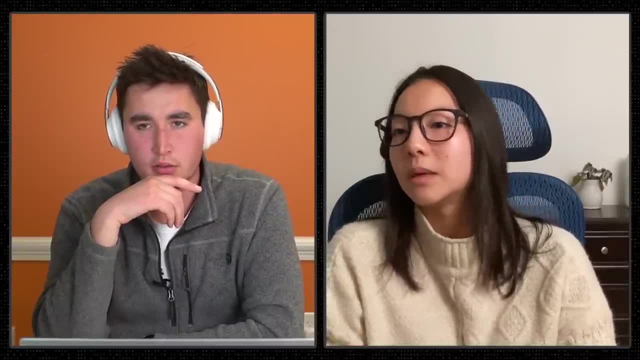 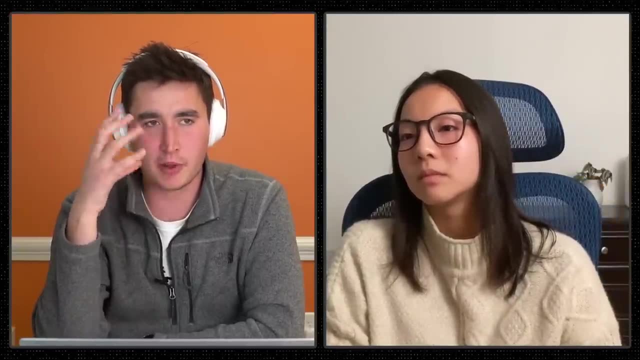 something like that. we can just go through this model and say, oh, this might be a spam account. yeah, would we want to do it? a single post or would we want to like? i guess i'm just trying to think about that. detail is like you know, each post goes through this, or is any other? 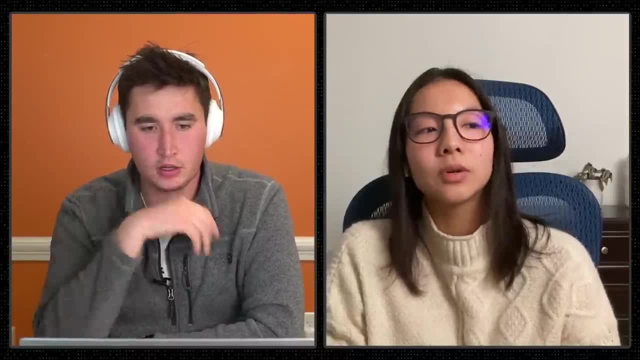 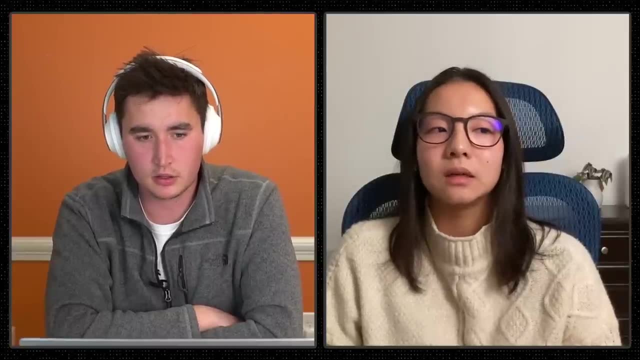 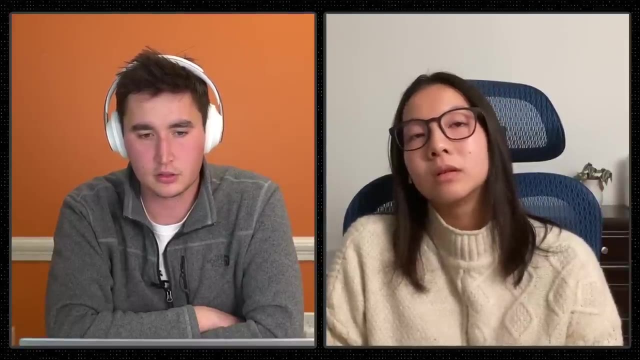 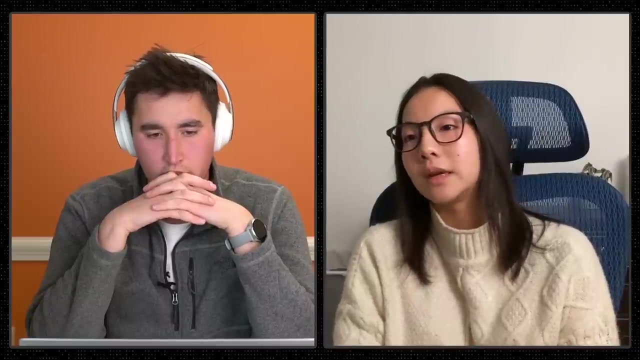 things that we might want to do here. well, so the way that we implemented this, it would be the specific accounts. okay, right, um, so i i do think that you would maybe wait for an account to have a few posts, but then, hmm, well, so how? i think the tricky part is: how do you catch a spam account before it posts any spam? 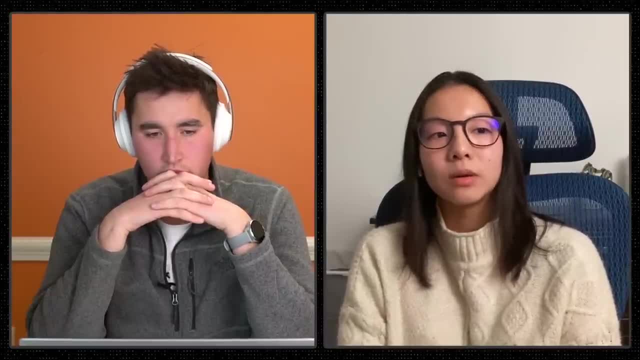 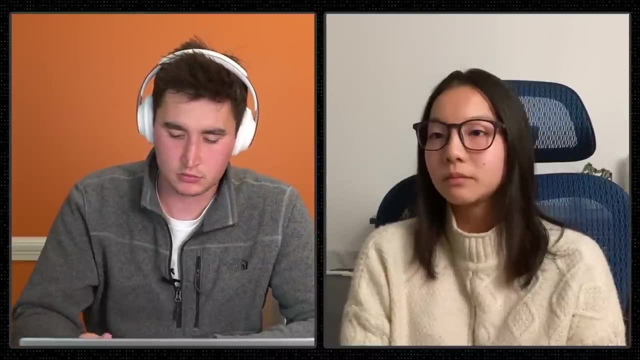 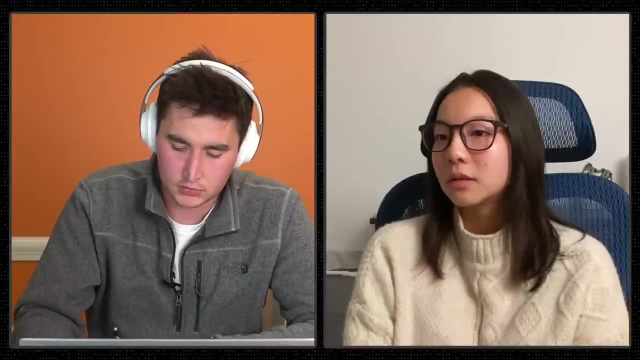 mm-hmm. right, and so the way that we've set this up it's it's to kind of go through existing users and label them as spam or not. i do think it could be interesting for a future model to to maybe assess the first post that an account makes and determine whether or not. 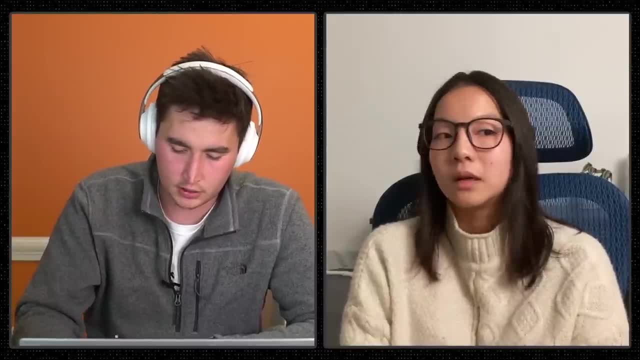 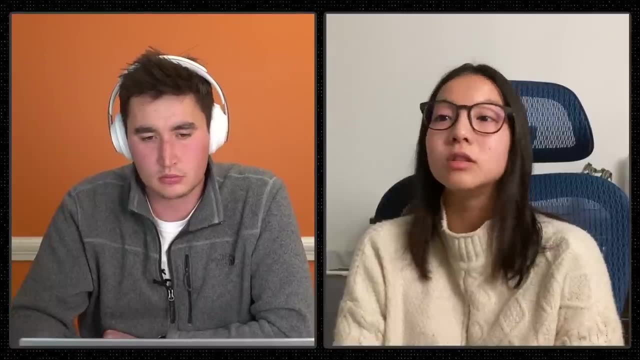 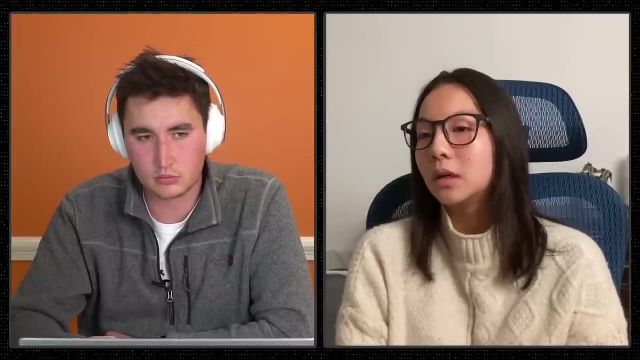 it's a spam, uh, post, yeah, and then from there you know if it's, if it determines that it's not and there's no way like maybe these newer accounts should just be ones that you keep monitoring for a while and you keep reassessing, whereas older- i guess you would say- legacy- accounts might have. 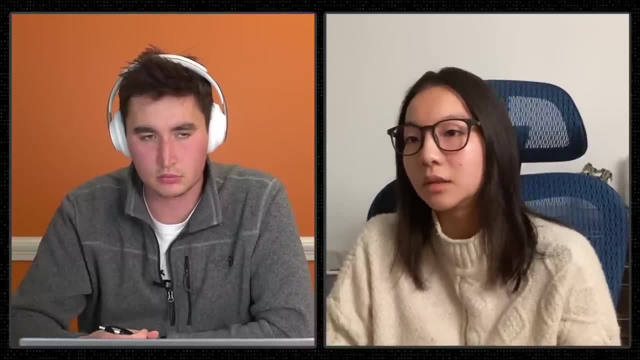 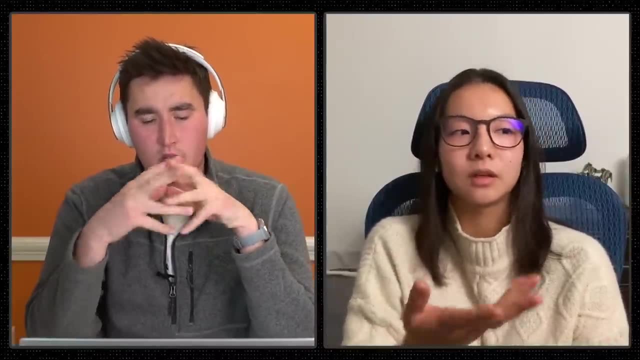 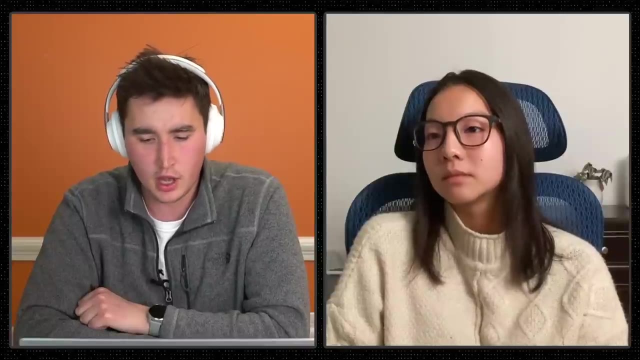 um, might have more lenience, right, yeah, unless maybe a ton of people start flagging it. yeah, that, uh, but hopefully our, hopefully our other implementation would be able to catch that. yeah, that, i think that makes sense to me. cool, i think that's all i have on this. 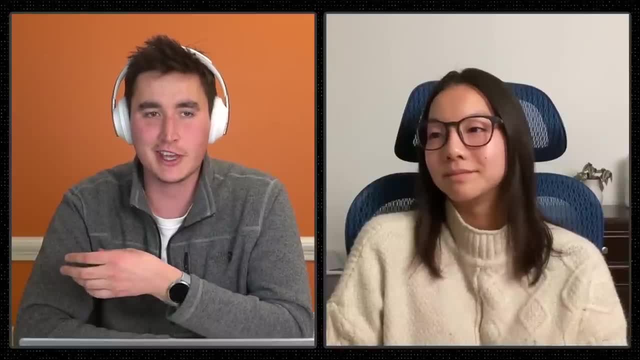 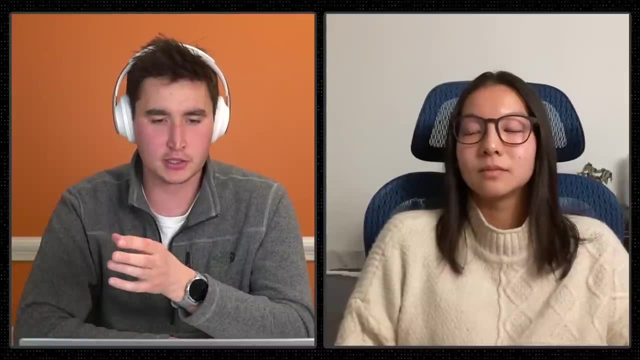 prompt. uh, this was an enjoyable discussion. uh, i think you know it's interesting to think about. i think there's a lot of different avenues you could go. so right, i know we're running up on time. i do want to just, i guess, quickly pause and, uh, just see if you have. 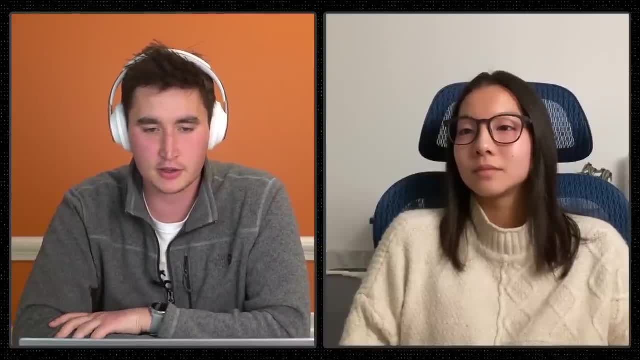 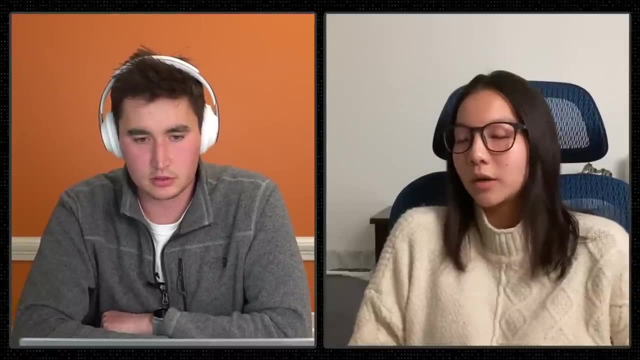 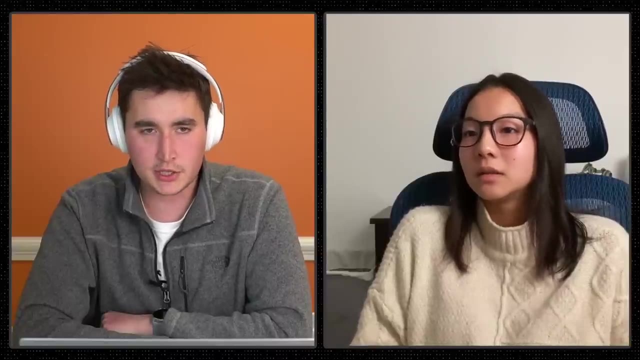 any questions for me before we kind of conclude this uh interview? yeah, definitely. so i'm just wondering, um, like, what are your favorite and least favorite aspects of you know your role as a data scientist at this company so far? yes, i think a big one is. i mentioned it at the start of the interview. 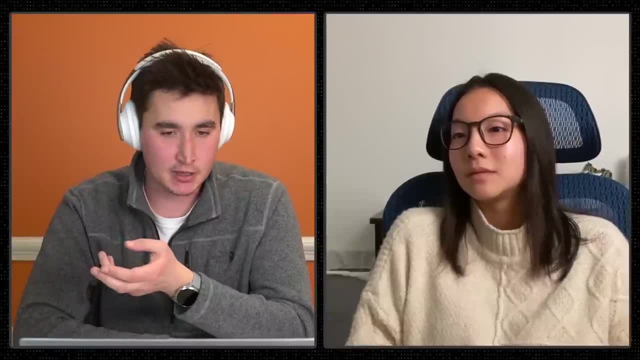 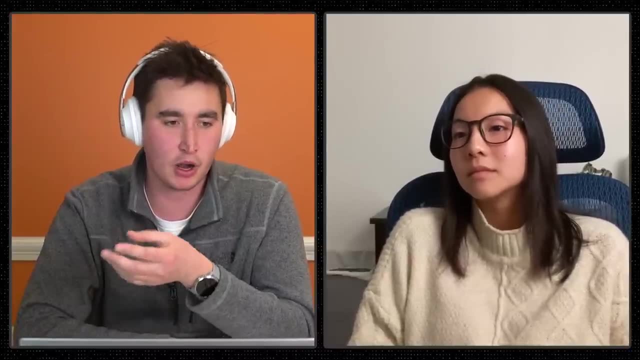 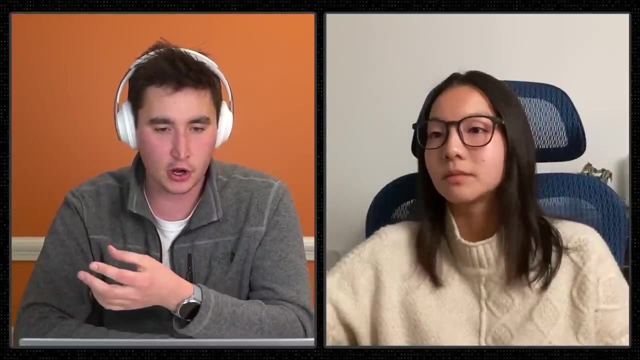 is just um the team. the team is really impressive. you know it's a diverse set of backgrounds, both people you know, phd type people from harvard, mit, but also just some really, really brilliant, self-educated, kind of just learn this stuff on their own. bring a different perspective to the. 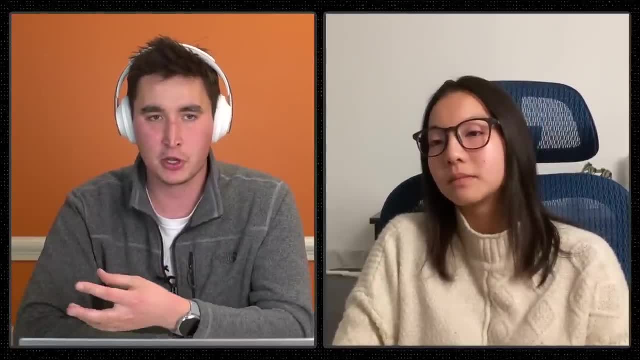 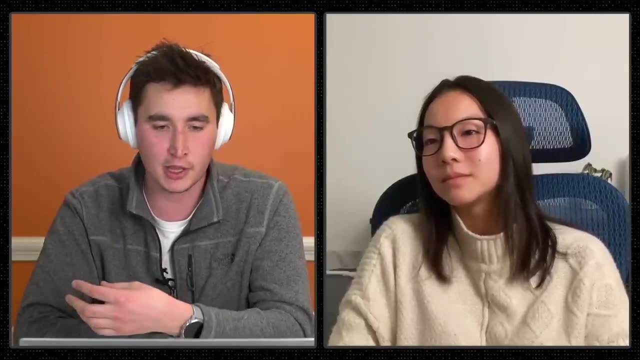 table people that are on this team. so, you know, from my perspective, you know, one of my biggest goals, you know, in this role is i want to continue to grow, i want to continue to develop. you know certain skills that i have. like i come from a natural language processing background. 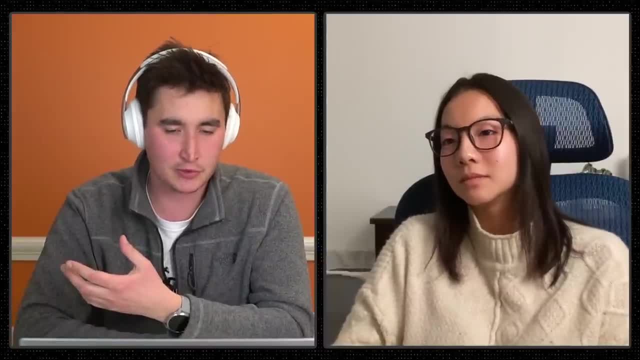 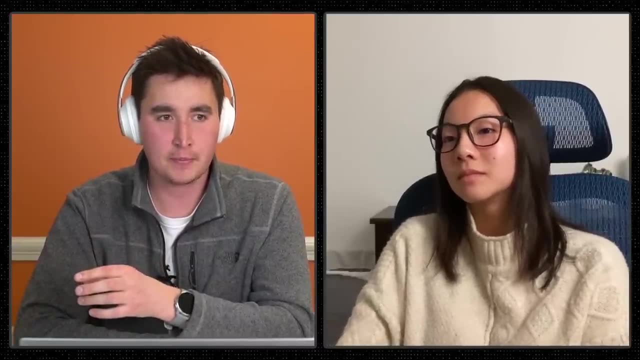 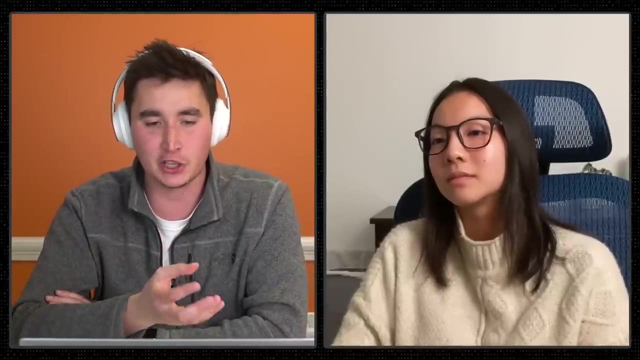 you know i can apply those skills, but i don't have as much of that systems background. i don't know how to you know deploy this on a production scale. so you know what i enjoy. um, you know most i think about this role is just the opportunity to gain, you know, those insights. just learn from people. 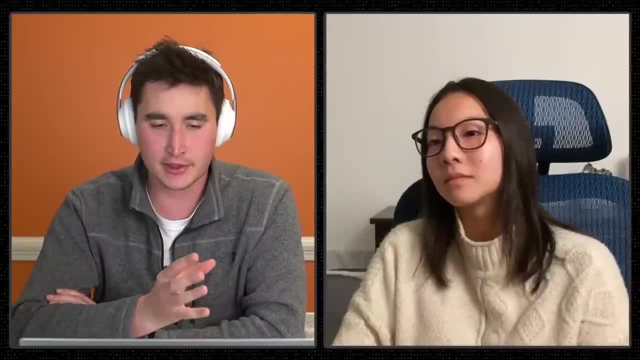 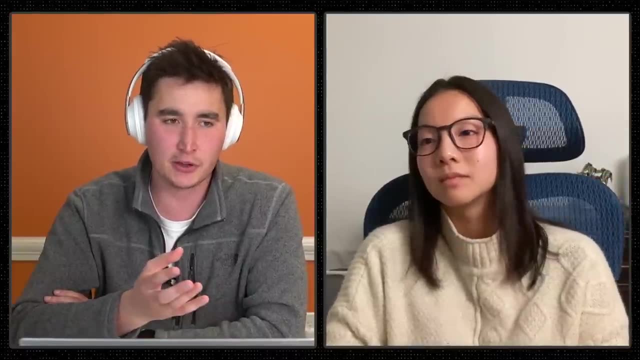 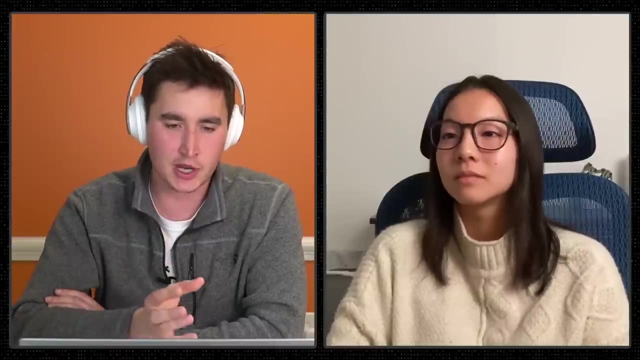 that have expertise and skill sets. i don't, because i think that that is helping me become a more real, you know, member of the team- i guess on a separate note, like that's very much like team based, but also there's just a lot of flexibility to move around in the role, like i've kind of stepped into. 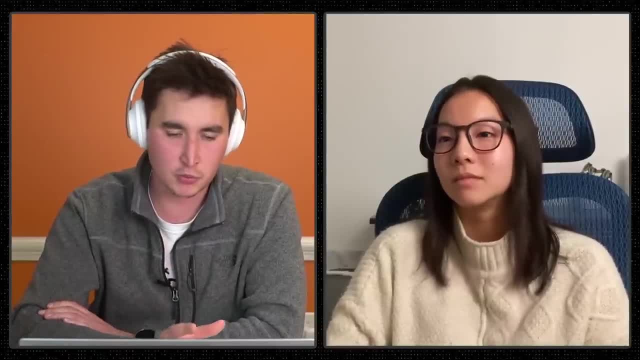 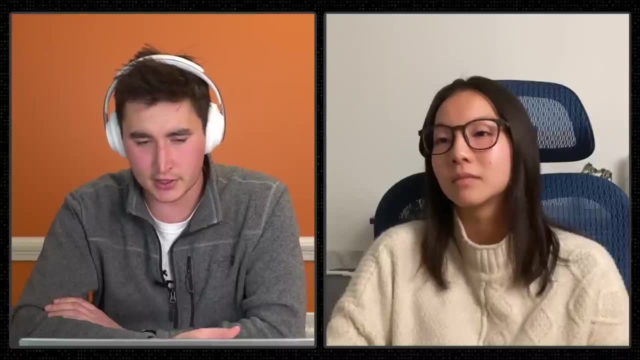 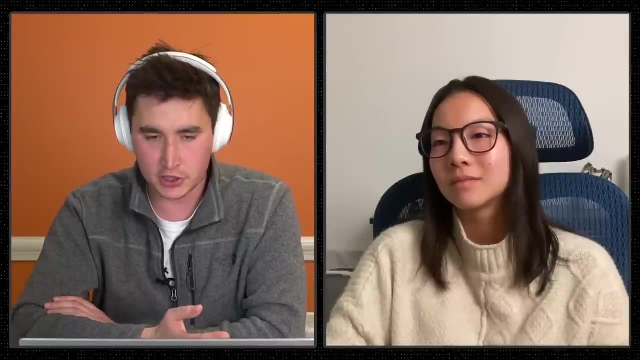 more of a managerial type role recently, whereas i very much was more of an individual contributor writing code, you know, on the front lines previously. so i like that too. on the flip side, i think least, uh, what i enjoy least, uh, you know this is, i guess, love-hate relationship, but you know work. 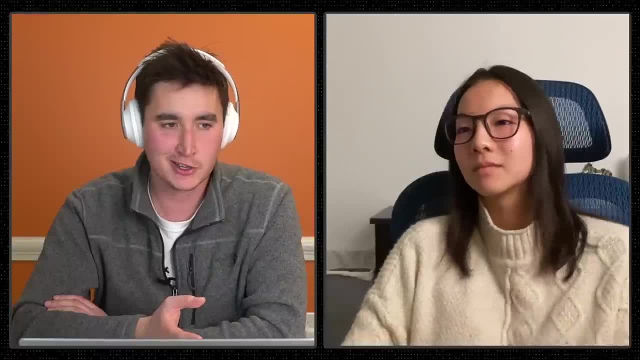 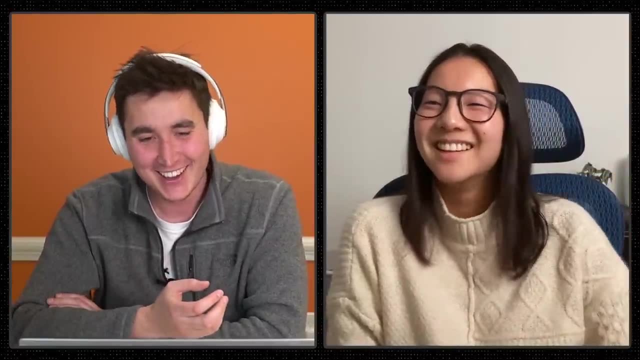 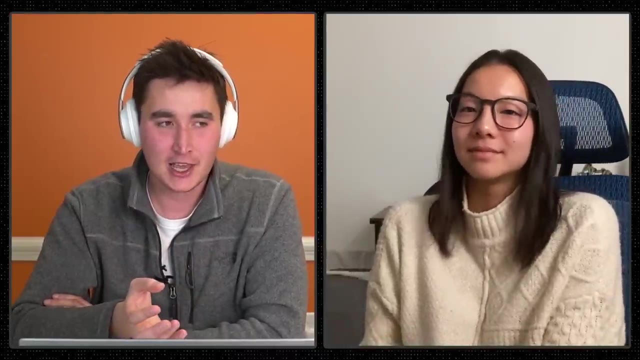 bit of a grind, like we work hard hours. we, you know it's uh. you know to be classic and cliche. you know, work hard, play hard. wait, sorry. yeah, work hard, play hard. that's the saying. um, so i mean it's uh. we put a lot of hours in there's, late nights sometimes. but i think with that you, you do get. 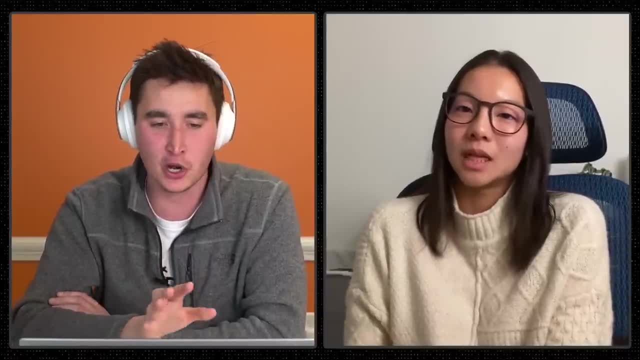 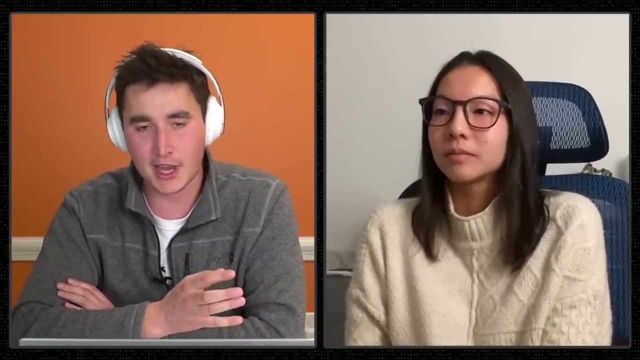 that learning, but it's just like sometimes it's a balance, it's like just making sure you know when to step back and reassess and just like not get too burnt out. so, uh, love hate relationship on that side, but i think that overall i would take that over. not being challenged, yeah, okay, awesome. 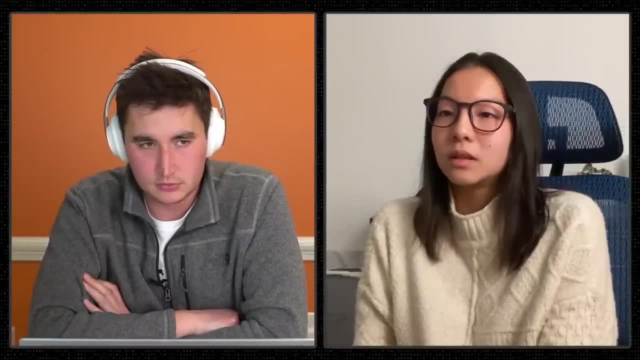 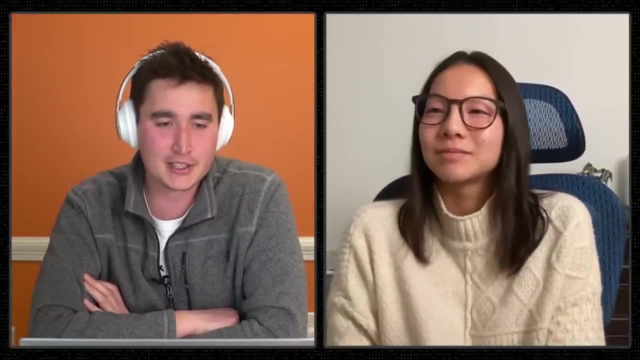 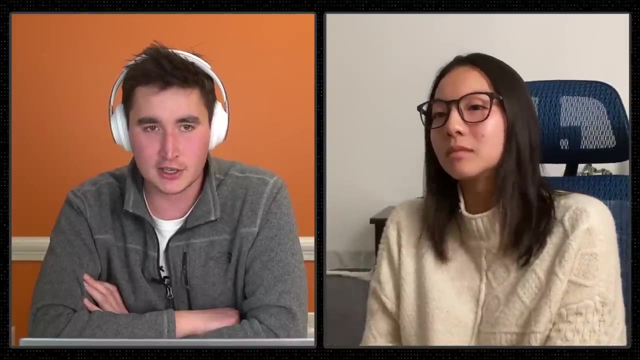 um, and how long have you been working there so far? uh, i think this is my fifth year, so you know it's been a little while. so you know i've- yeah, because i've had the ability to kind of switch around my role. i think i've stayed kind of engaged and, yeah, i've just had opportunities. 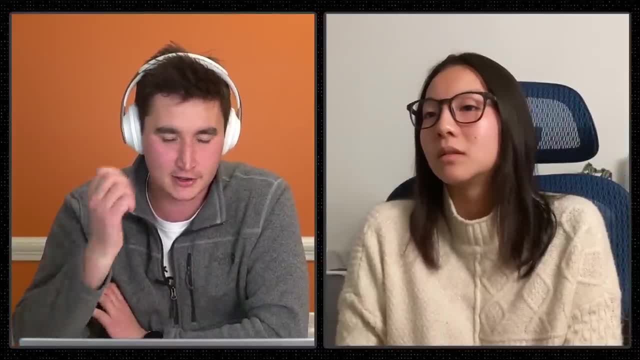 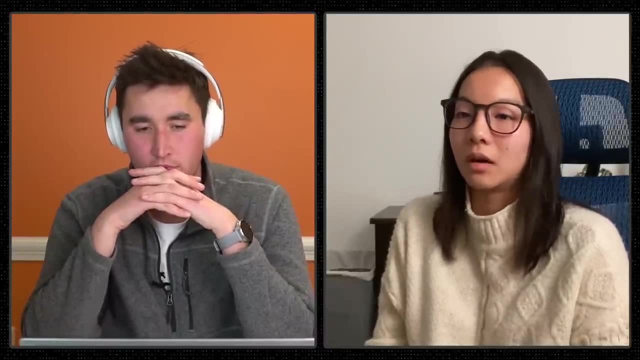 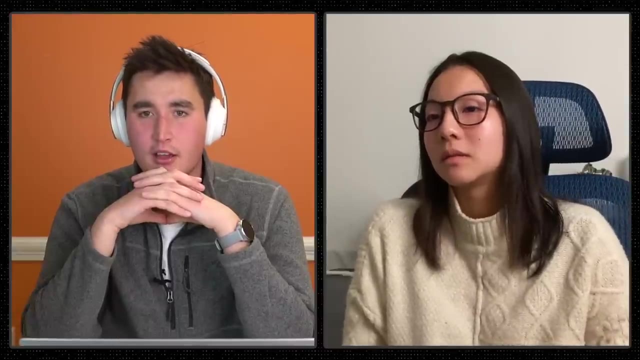 to learn different stuff, and i think that's kind of what has helped me stay this long right. yeah, yeah, yeah awesome, because my follow-up question was going to be like: what opportunities for growth are there like within the company and how, how does the company support that growth? yeah, yeah, um. 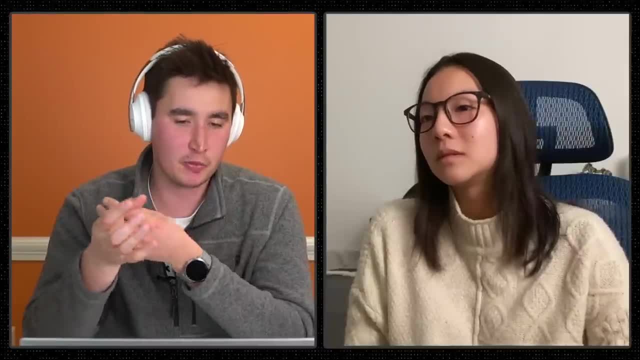 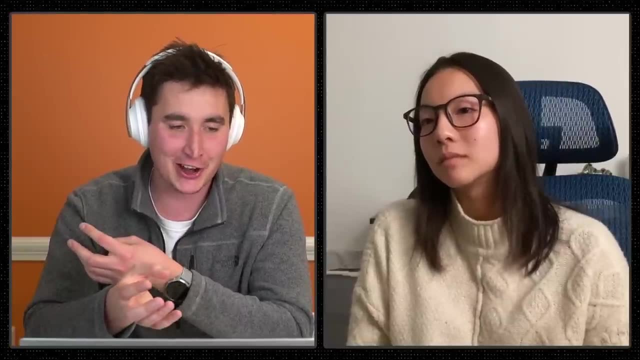 i mean there's a couple things i think just in general from from being in a team environment where there's a lot of just driven people that want to know the latest, you know the state of the art like. sometimes it just naturally kind of comes out during lunch discussions and whatnot. 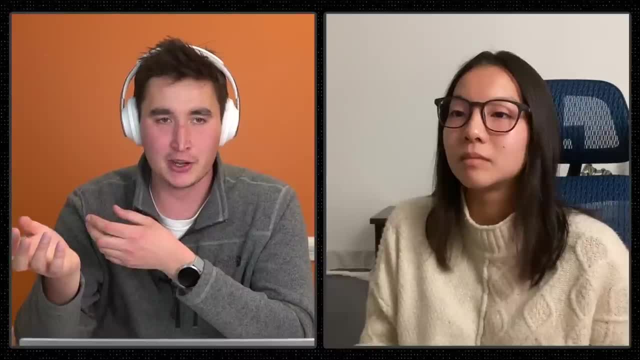 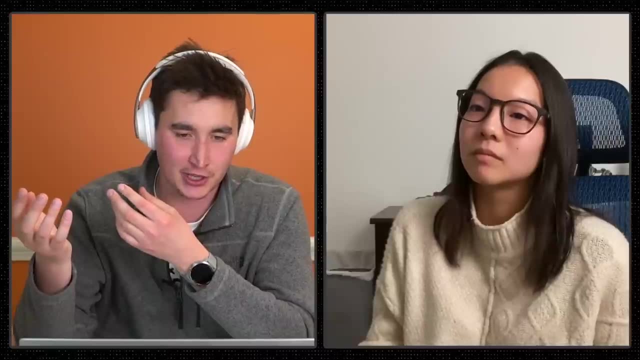 some people are working remotely somewhere at you know the office. but you know both channels. like you know, if i'm at the office we go out and you know some of this. just the discussions just happen, naturally, you know, at lunch. or we sometimes host remote kind of like you know zoom lunches where you all kind of just hang out and 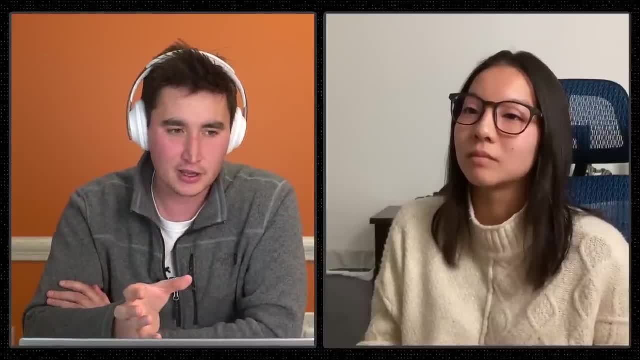 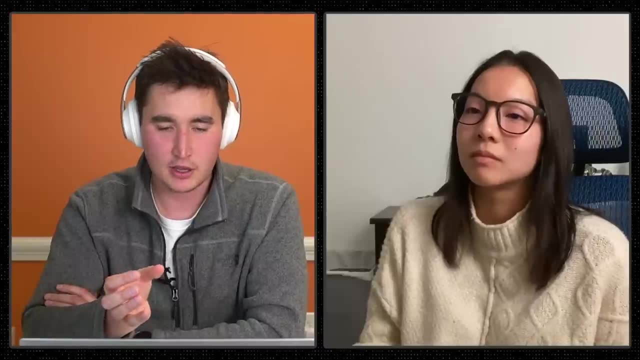 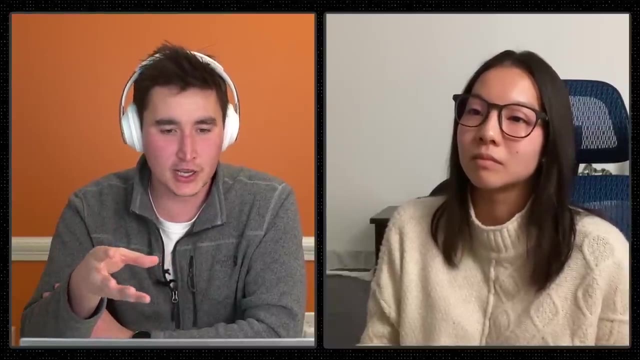 you know, chat about things. so that's like kind of an informal way from a formal perspective, like we try to, you know, make sure that everyone that's here is happy. uh, we, you know, have routine, um, you know, performance kind of check-ins, and perform like i don't. i don't say performance as 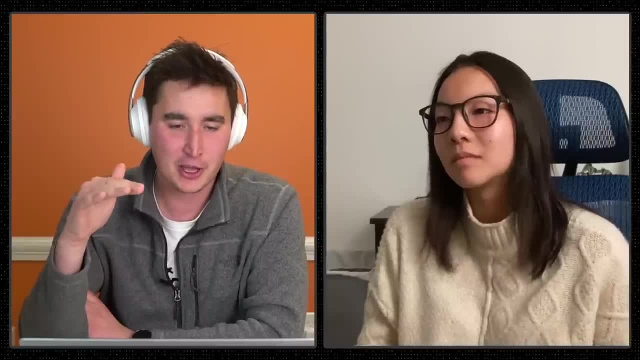 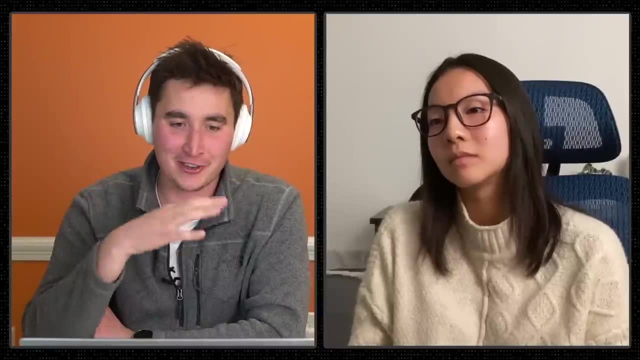 in, like you know, very strict, like if you don't meet certain bar you're out. but it's very much a constructive process where everyone on the team, no matter who you are, whether you're you know the ceo or if you're you know, a junior engineer, like everyone has performance reviews. someone on the 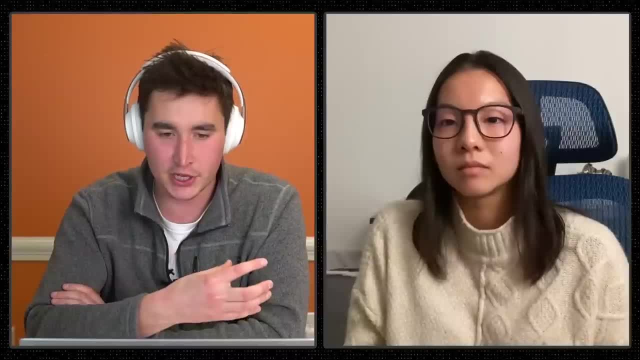 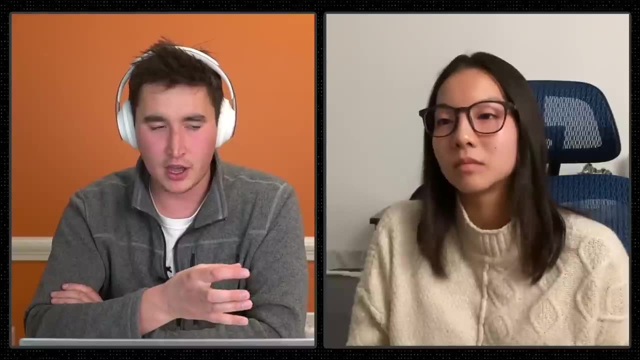 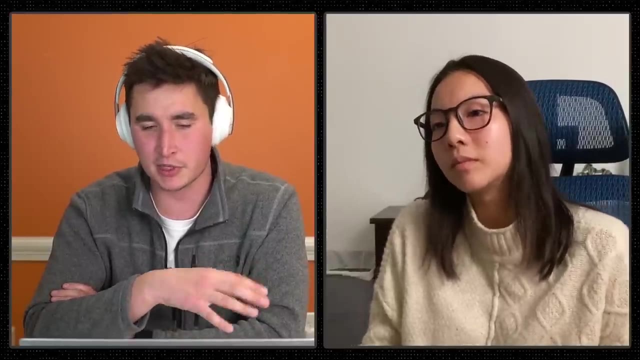 team is tasked with evaluating and having that conversation, what you're doing well, what could be improved. so there's like constructive feedback across the board and we try to do that um either every quarter or every other quarter. um, typically every quarter we try to have something. yeah, sometimes it's more formal, sometimes a little. 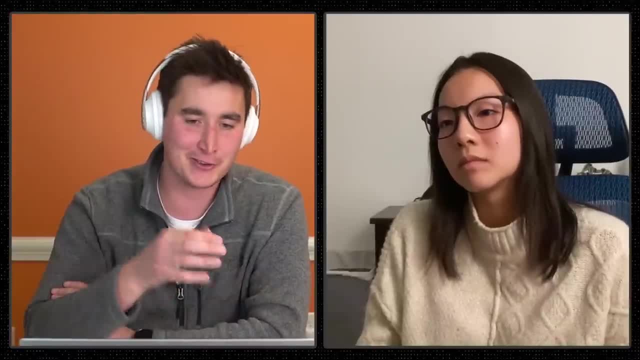 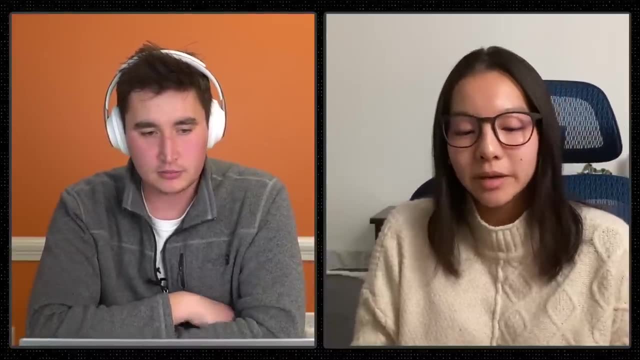 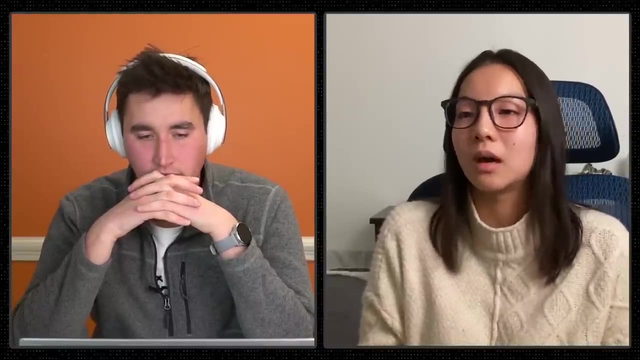 bit less formal, but everyone's critiquing everyone, no matter if you're the, you know ceo, uh, or you know you're more junior, awesome, um. and then for my final question: just how, like what? what would my first, maybe six months kind of look like? what would uh be some of the projects that i'm working? 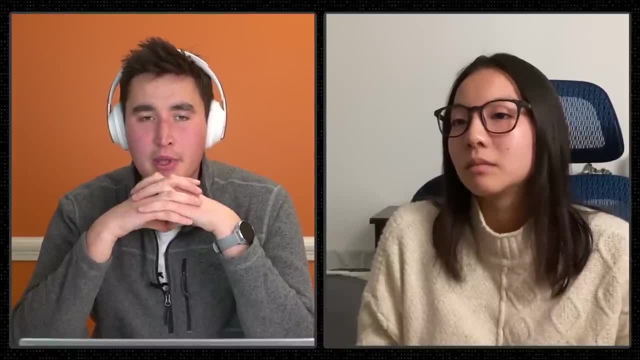 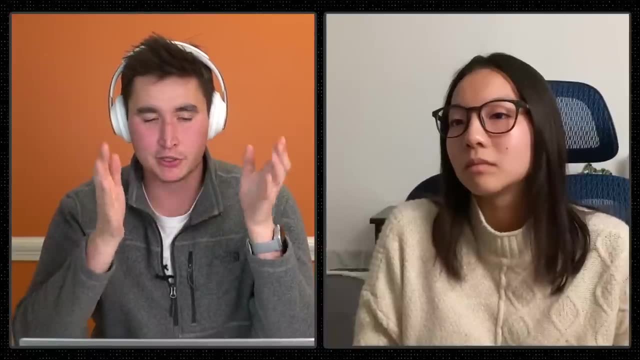 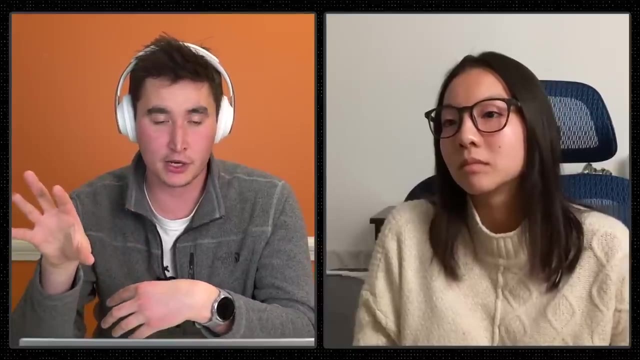 on look like yeah. so i mean, i think one of the most important things from my perspective for anyone joining the team is we don't want to have new team members be siloed. we want to make sure that they are exposed to what we have kind of out there on- not just my team, but you know. 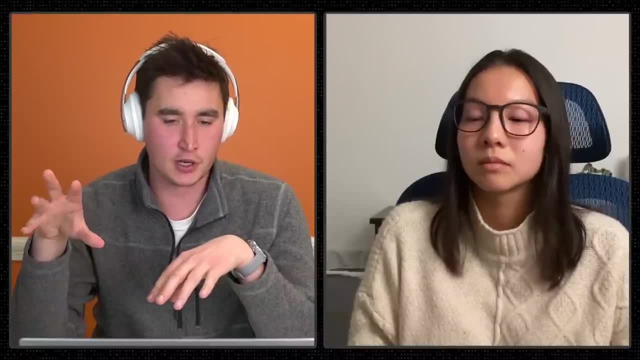 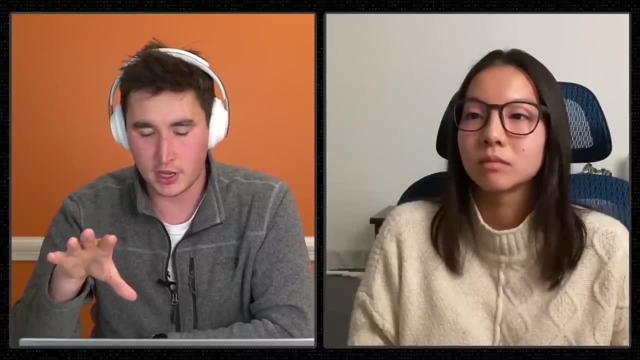 surrounding teams. so a couple of things that you'll be kind of doing is, first off, you'll be, you know, assigned immediately upon arriving a mentor that can kind of help guide you and, um, you know, you'll specifically like: this is a hot role for you know my team. so, like they would, 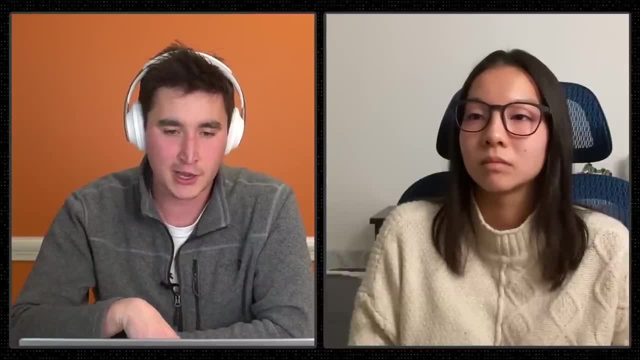 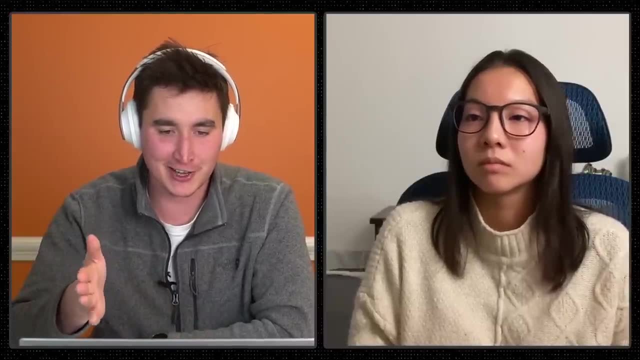 be kind of introducing you to our systems, walking you through the code base, you know, introducing you to the other people on the team. so one of the big things is like you have this mentor that's kind of there to guide you every way, every step. but another important point is like we try to 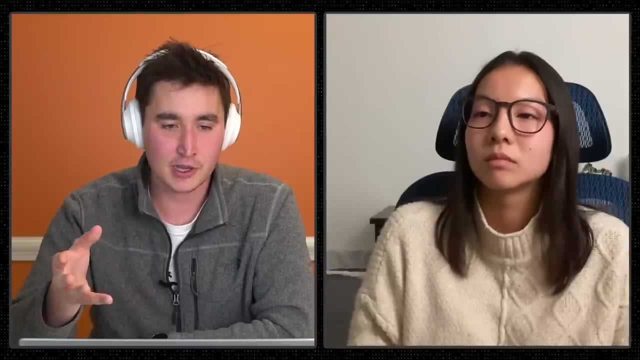 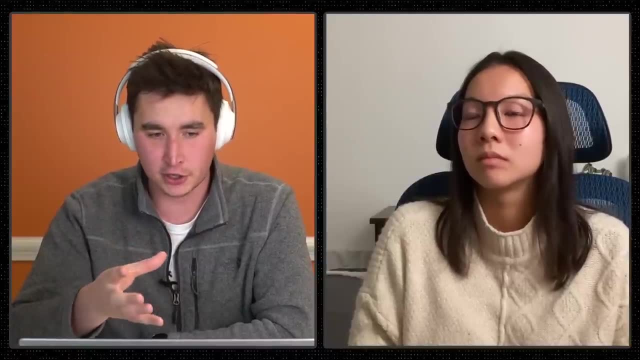 make sure you get one-on-ones with everyone on the team within the first month approximately, at least within our small team. so like you get to meet everyone on the team, you get to introduce the code base. so it's really just kind of getting warmed up, getting comfortable seeing things. 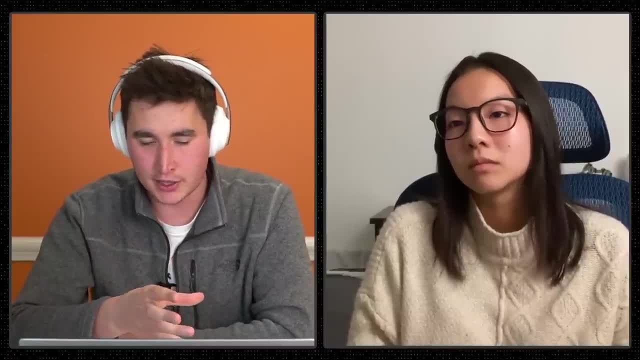 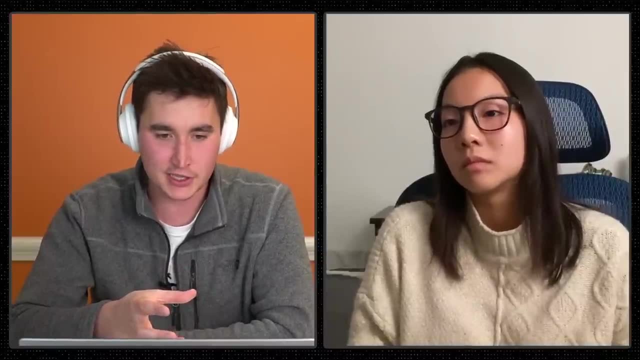 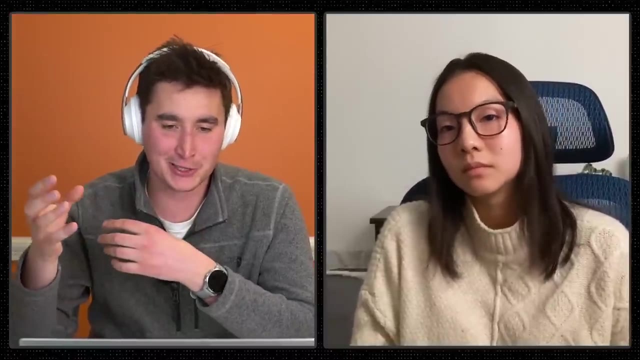 probably, you know, end of month one to, like you know, month three. a big part of it will be, you know, tackling some kind of more entry-level tickets on the systems really get your hands dirty. plug in and, and you know, they won't be the most complex, you won't be designing a system from scratch. 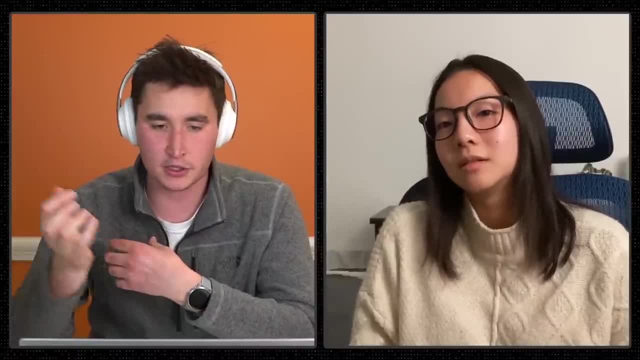 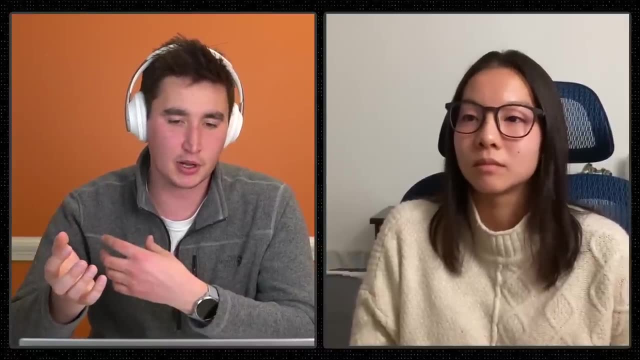 but taking our existing systems, you know, ironing out some bugs, all that get more comfortable. after that you'll be kind of more potentially leading- not leading, but like kind of help co-lead certain initiatives. yeah, and that has a little bit more flexibility. you can kind of get different ways. 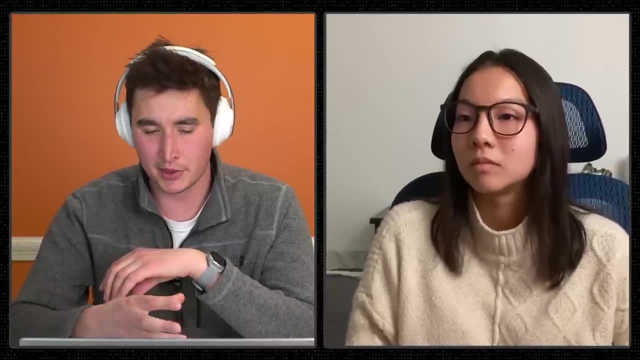 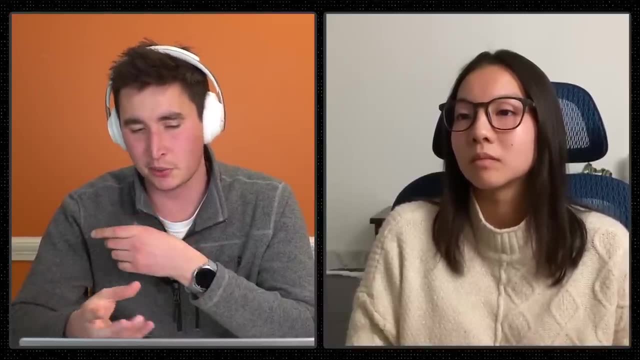 whether you want to be really the one grinding out the code or you want to be more thinking about the design and all that, and i think the only other thing is like, kind of throughout this process, we try to also introduce you to some of the teams that we work closely with, so you'll definitely 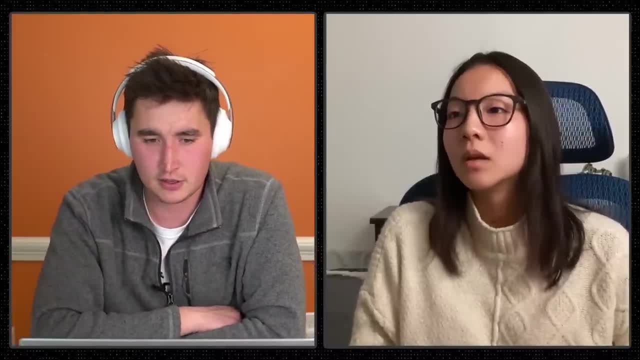 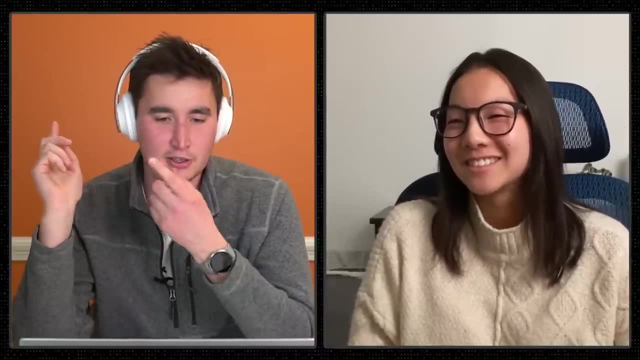 have some interaction with them. but that does that answer your question? yeah, for sure. yeah, awesome. well, thank you for your questions. awesome. so i think next steps from here is there's going to be a software engineering uh interview, so that will test more of your python skills, and then also 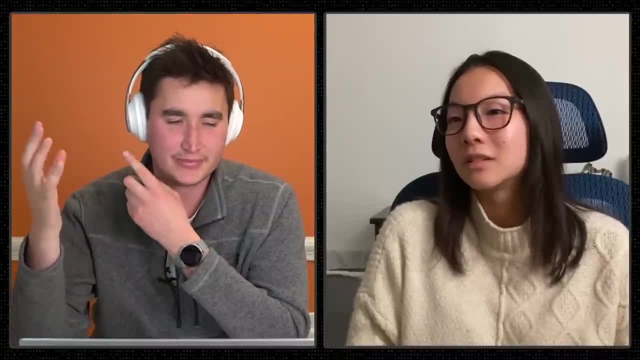 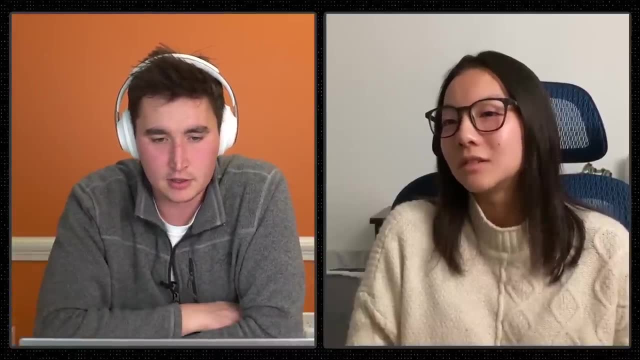 likely it will be like a behavioral interview as well, where just engage a little bit more of your career interest and all that. so next steps: you'll hear back with us in the next few days probably, and we'll go from there. okay, awesome. well, thank you so much for taking the time. 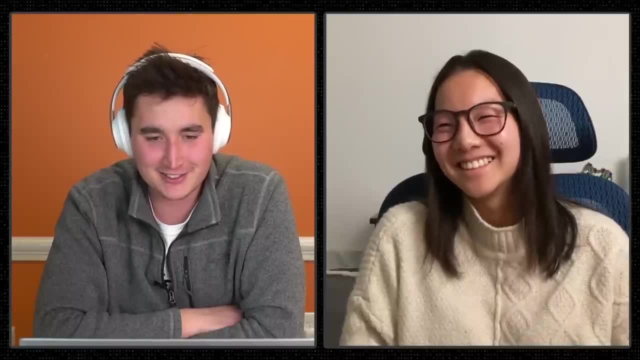 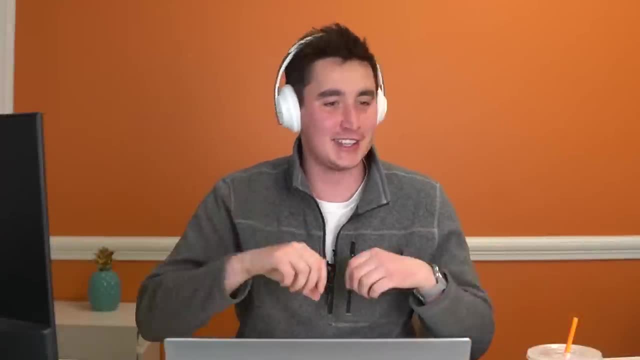 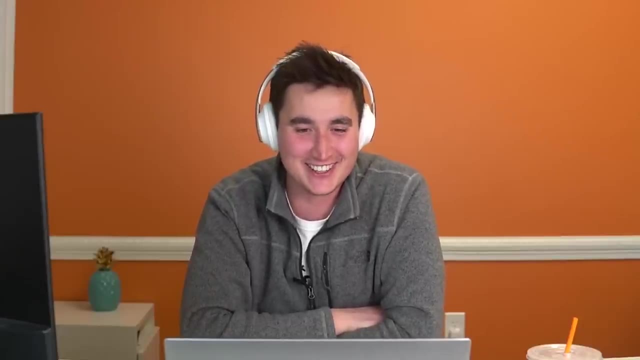 yeah, it was a pleasure and nice meeting you and the day. yeah, you too, thank you see ya, bye-bye, all right end interview. i'm not geith cali anymore, i'm keith galley. you put me on the spot answering, uh, some of those questions at the end. i had to. 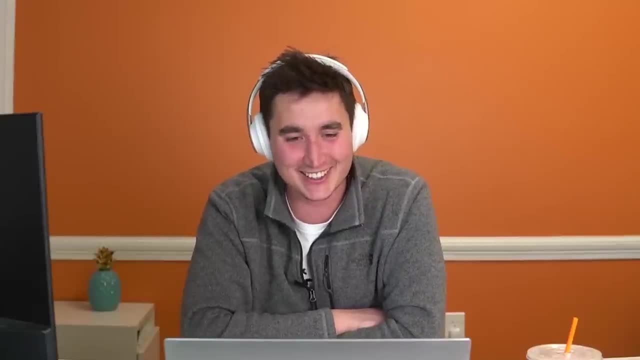 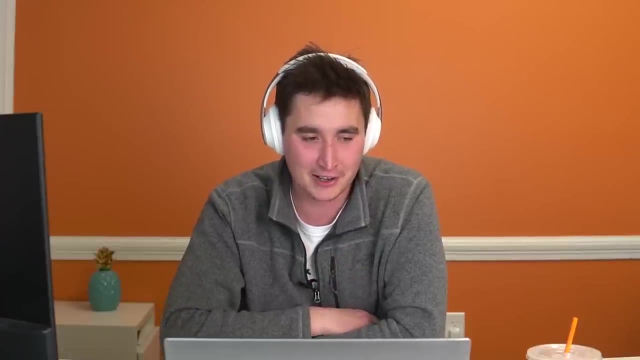 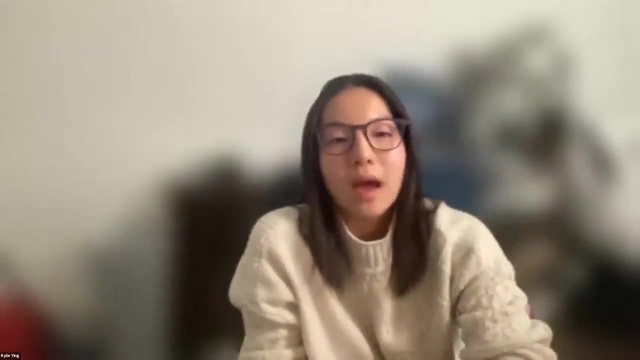 tap into my uh intro to acting skills, to like feel it. but i mean, honestly, i feel like i could answer it how i would answer it if i was in that situation and kind of from prior career experience. but yeah, because what were you saying? well, i feel like a critical part of interviews is asking questions, to look engaged. 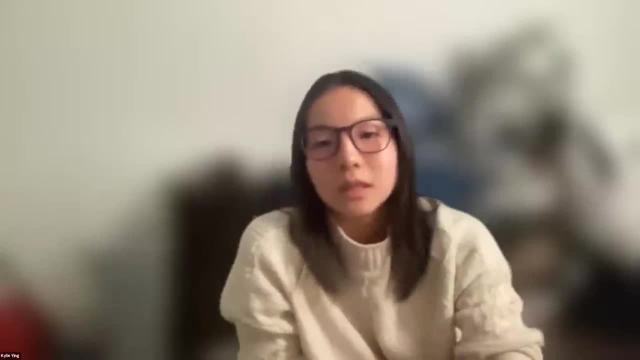 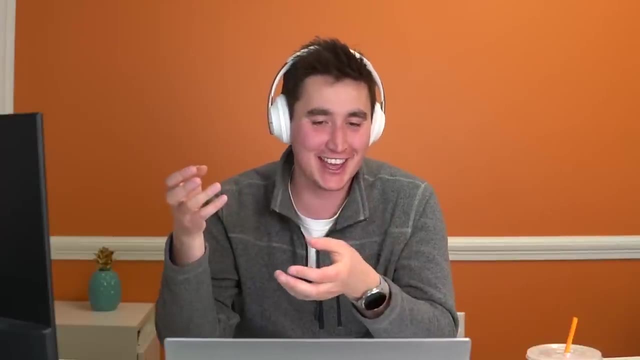 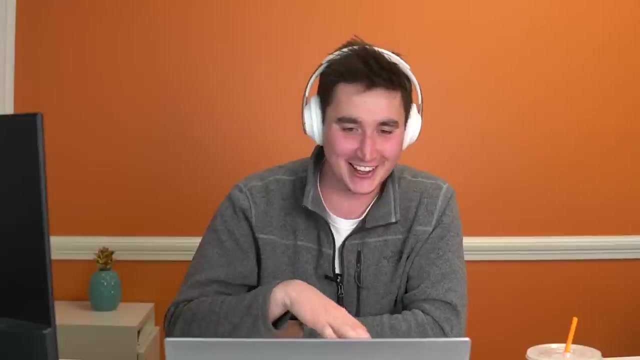 and uh and like genuinely interested in the role, right? so i didn't want to just be like yeah, yeah, yeah, that's fair, and the reason i asked that is because that is a important point. so i i just i wasn't, i guess, preparing to be on my toes and like getting ready to answer these, but i think it was. 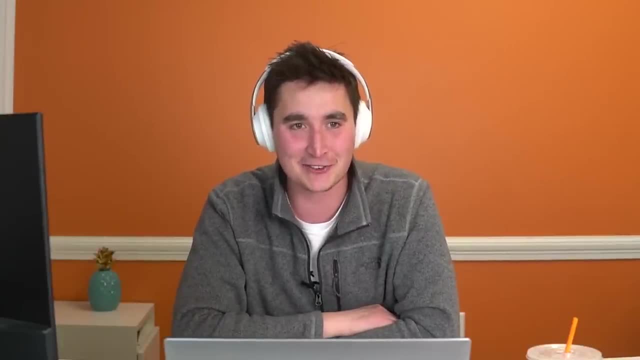 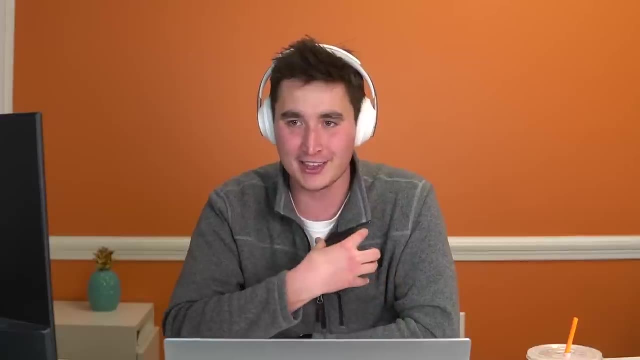 good that you did ask those questions, and i think one thing that might be interesting is for you to kind of evaluate kind of my breakdown, my responses and stuff and what you're looking for, because i think one thing that i think about in these interview settings and one thing i think is: 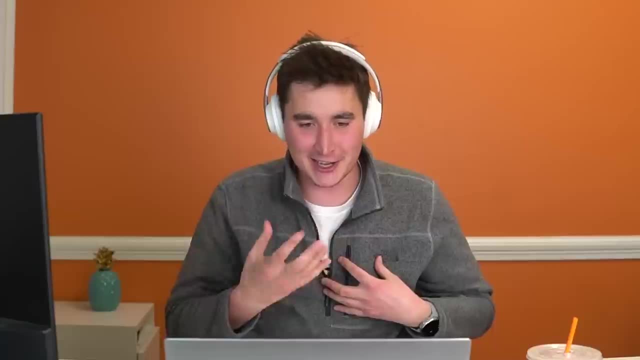 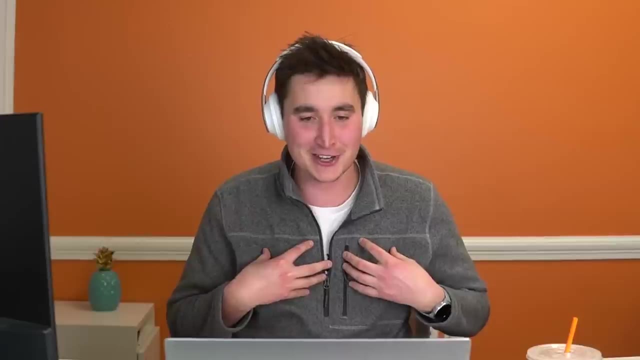 important to keep in mind is, like i very much it's an interview for you, but i'm very much also like you're interviewing me and like for me. when i was doing a lot of these interviews, like i definitely got stressed out when i was interviewing certain people that i knew were 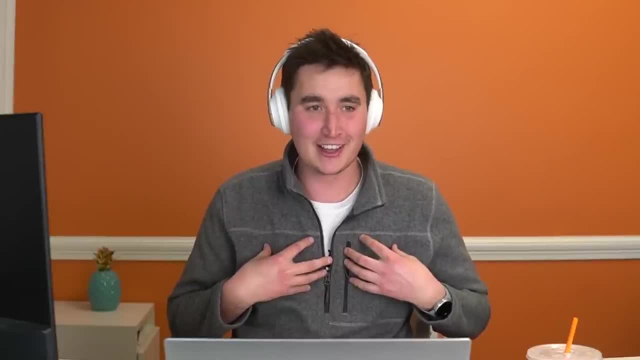 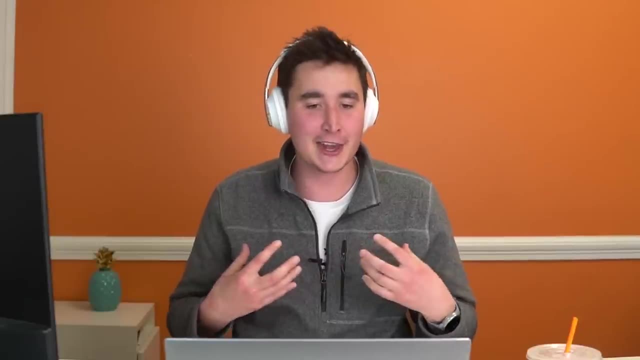 like high level. we really wanted to land this person. so i feel like, uh, like keeping that in mind as an interviewee, that, like you know, this is not a one directional thing like they're. like i had nerves, you know, going into this, even though this is a mock interview, because, like 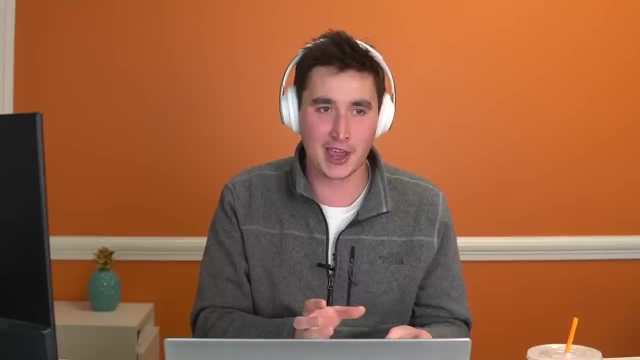 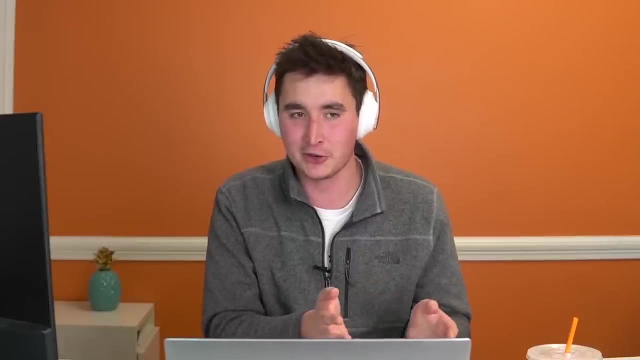 i wanted to ask the right questions, i wanted to get the conversations to do the right way and like that's definitely how i felt in real world situations as well, where it's like it's definitely both directions, especially if you really are looking to land a top candidate. 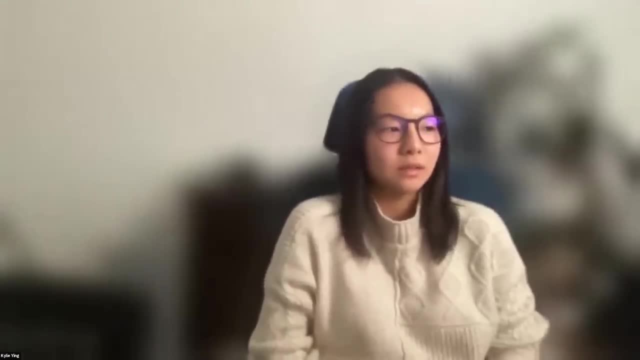 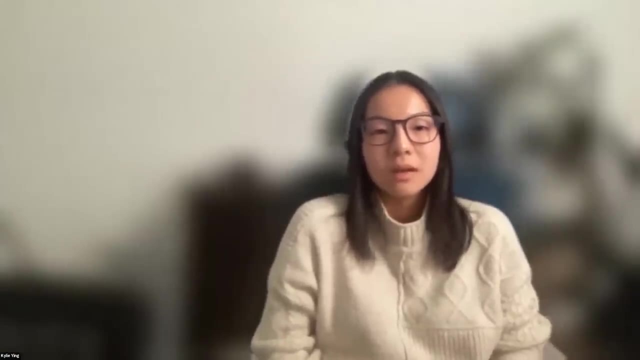 yeah, so i definitely think that, like overall, i mean i enjoyed the interview. i thought it was pretty like conceptual, which is good. i don't like when a lot of it is just memorization, and i think that in terms of the questions, well, okay, to be honest, i wasn't like 100. 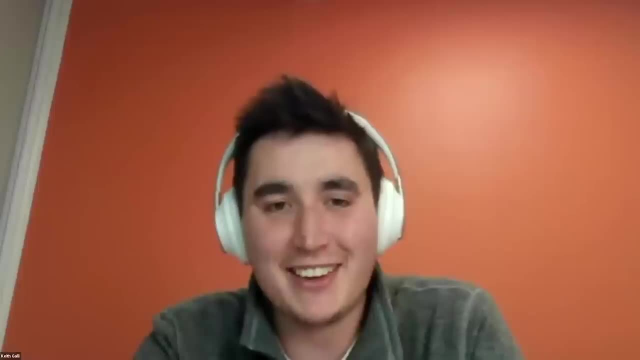 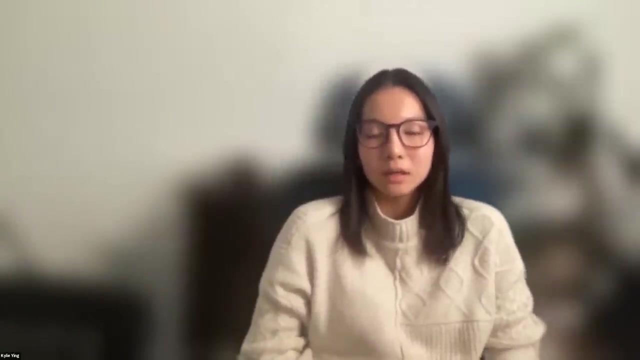 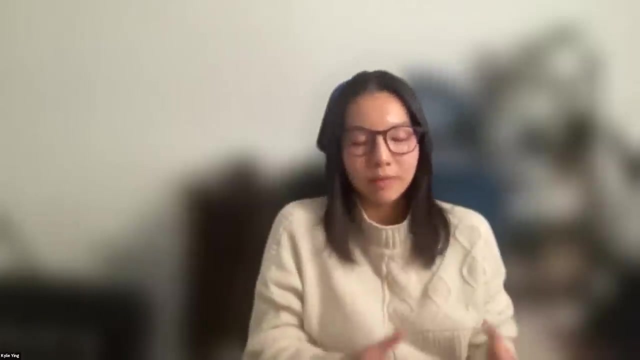 listening that much. it's not a real company. yeah, um, but i do think that i do think that being like concise in your answer is probably, uh, something good to practice. so i do feel like, um, you did talk about a lot of things where you could have just said: well, i think my favorite thing is this: 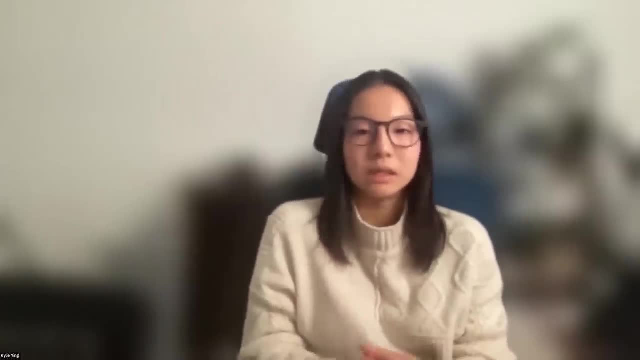 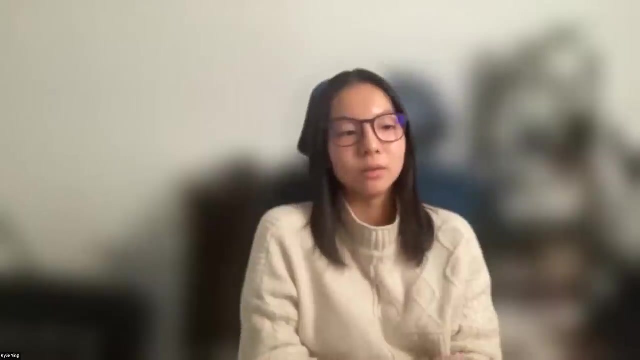 because i have a lot of flexibility and like i have a lot of growth opportunities and uh, that's kind of just like what i think is the best way to propel my career, whereas a negative is just that i feel like, you know, work is kind of a grind sometimes but like, but, we're all here because 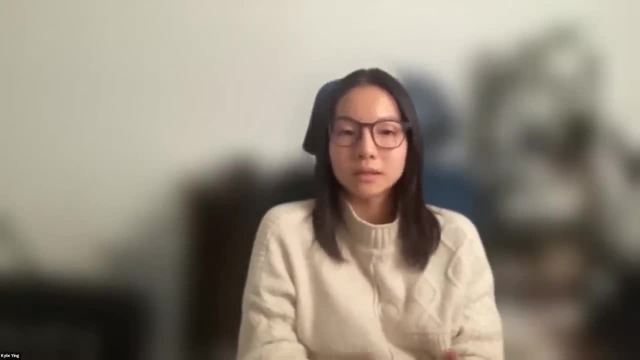 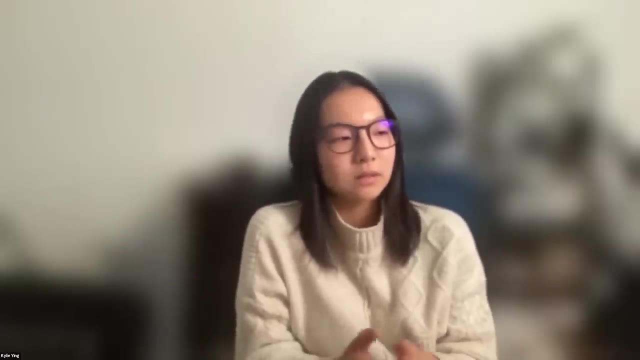 we're really passionate about the product and so like we're always like we want this to work and succeed and i want to be a part of that team, so like we work hard to make that happen. just like being more concise with those responses, um, and i feel like you know, i feel like when i ask: 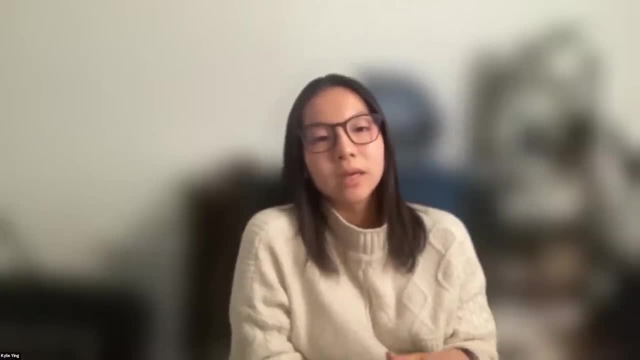 people what they want to do. it's kind of like evaluating whether or not it's somewhere i'd want to work right. so like if somebody does say like, oh, the work is a grind, then it might like that is probably one thing that i'm prioritizing. is that like, i want a work-life balance, or? 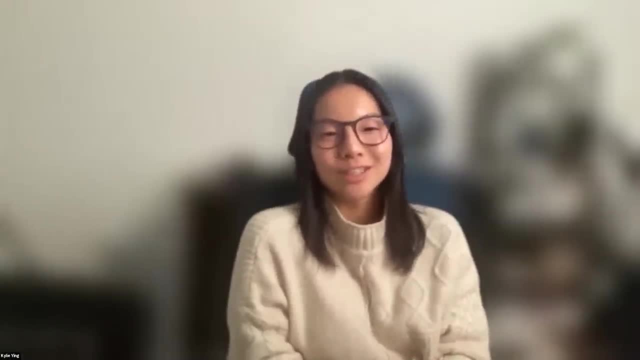 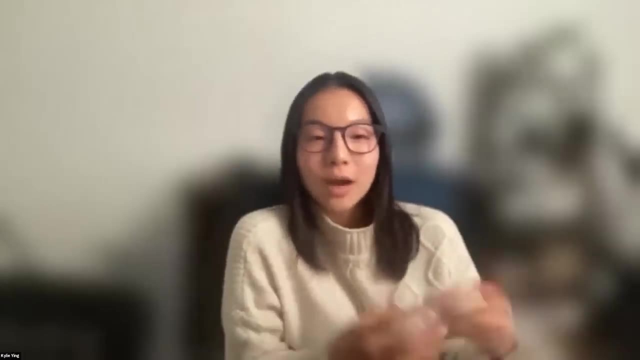 yeah, um. so i guess, like as an interview or something tricky that you could do is like, before asking, before being like, oh, do you have any questions? to kind of get a feel for what they're looking for, and then, yeah, your response to that. but also, at the same time, i feel like 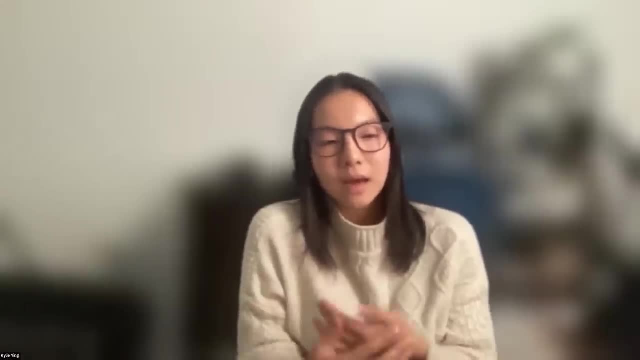 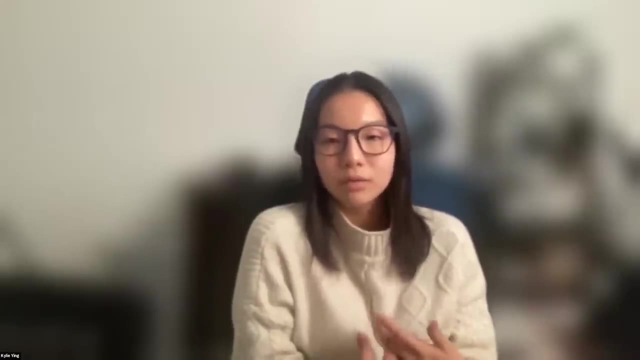 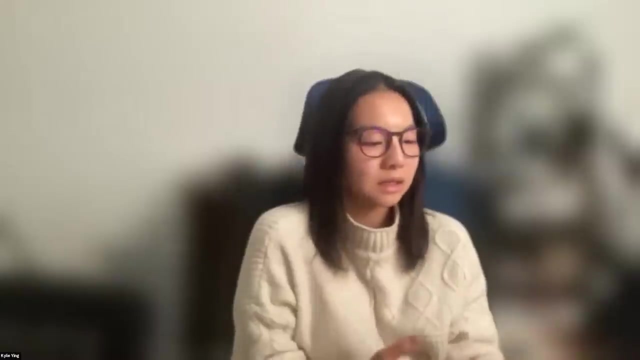 then it's not very like as an interviewee. i want people to be honest and genuine with their answers, right, like i want to be able to evaluate for myself, like like, oh, i i'm gonna expect to work nine to six every day and then have the rest of my time i'm gonna expect, maybe once every once in a. 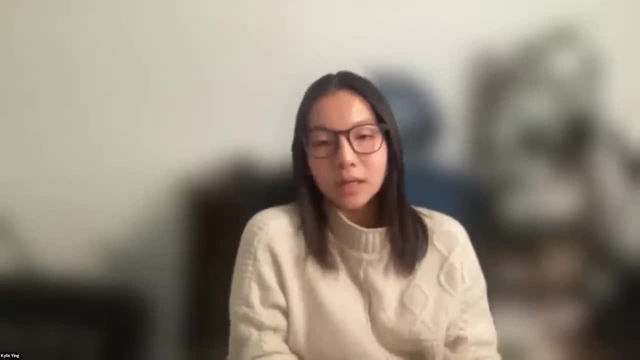 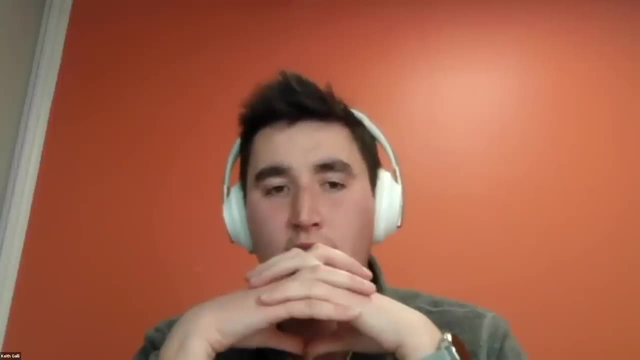 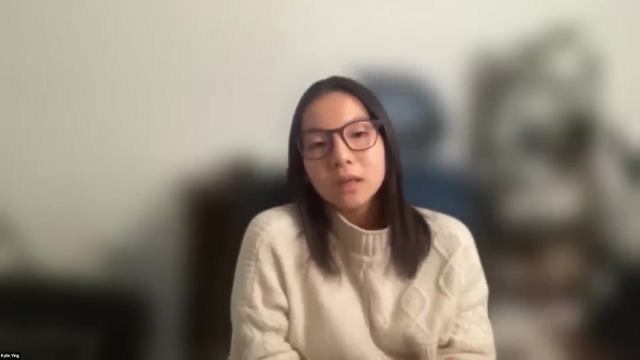 while to have to be on call, but not every night, and if, then, the reality is different from that, then i would be very disappointed, right, yeah, um, and i would want to leave, and so i think that those are things to think about, but i do think, like honesty is the best policy. yeah, um, this is. 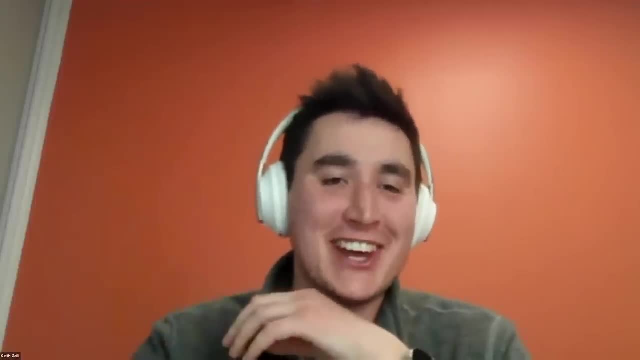 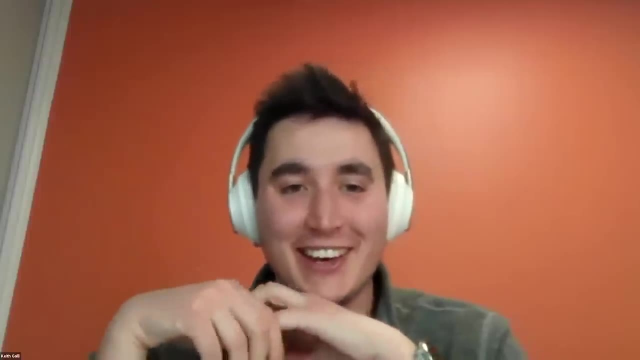 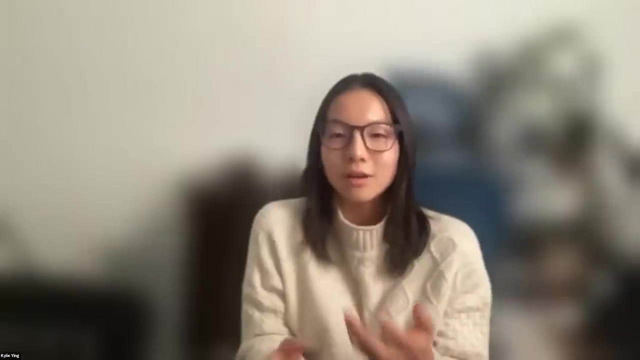 interesting because in all the interviews i did, i never really got the chance to ask that type of question of, like you know, evaluate my own responses in trying to impress a candidate. yeah, well, i definitely think. uh, one thing is like: even when you're interviewing, i do think you like add a lot of fluff in things. so i think that, for example, when you ask me, 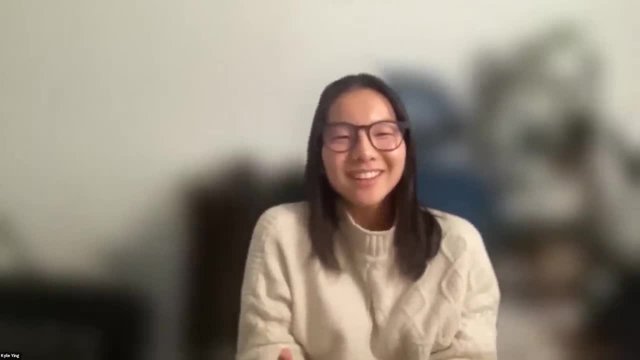 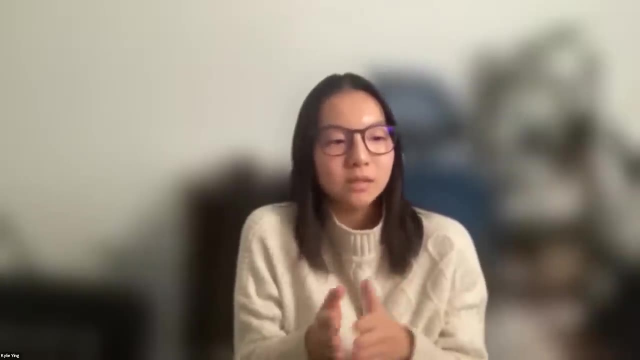 things like: oh, did you get the question? like you didn't even ask a question. yeah, at that point, when you were like detailing the problem and i think maybe just adding more breaks in between kind of your monologue, in a way like just being like: oh, does that make sense? 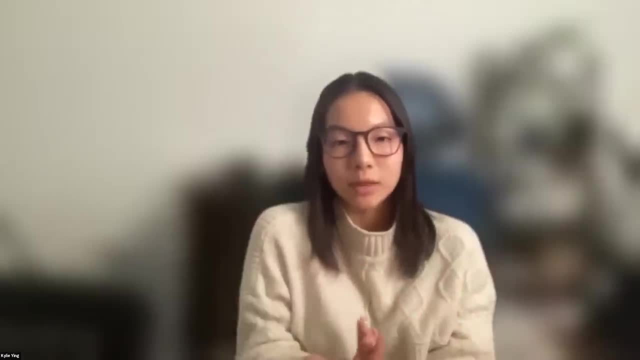 to give the interviewer, you know, some more engagement. also, a chance to ask questions is probably good, and i don't think you have to rephrase something multiple times, like when you ask what are some features that we should investigate regarding the bot issue. just ask that and then, if they have any questions, they'll like. 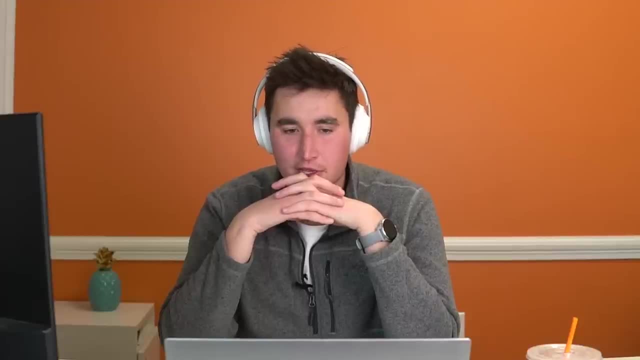 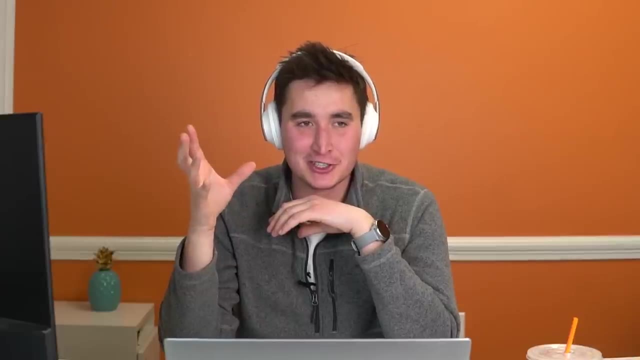 ask specifics, right? yeah, that makes sense and i feel like i goofed there. i definitely even in my notes. i kind of wanted to pause and just like see if you understood the like overall, i guess, like foundation of the the. it wasn't a question, that was the issue. i specifically didn't write question. 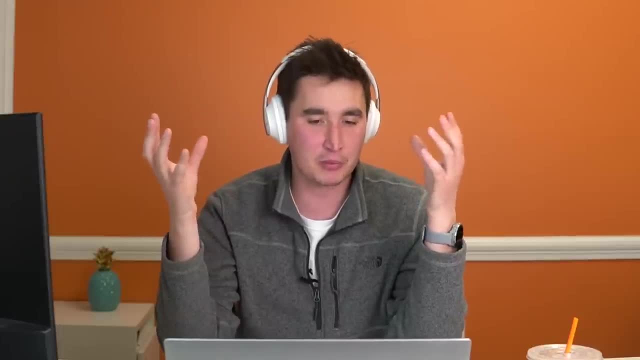 there like the premise of, like the context of the- uh, the problem context, i guess the that was it. there was no like question yet but i, even though i wrote in my notes and i fixed, i removed question, it just did like problem context. i think i said it out loud again, so it's like good. 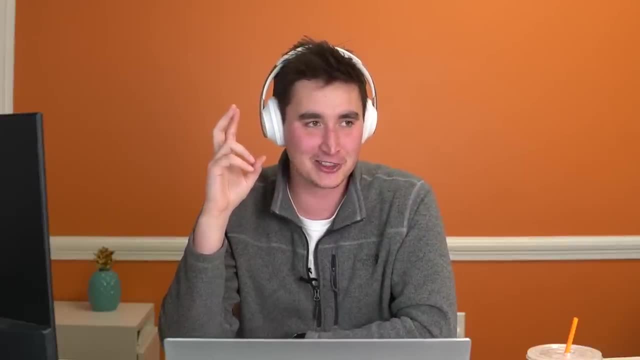 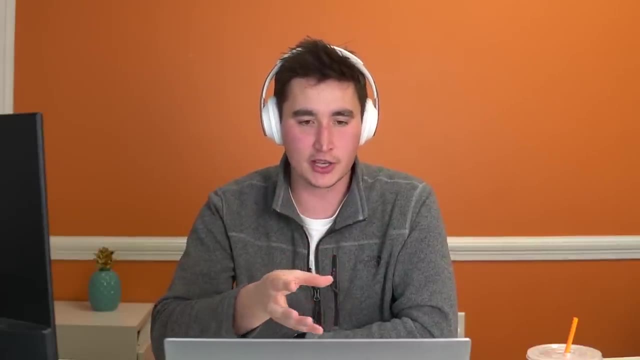 to know. i think it's good to know to not be too fluffy. i think i like doing that, um, so this is good insights from my perspective. i do want to just like as part of the uh video, also like give you some feedback, i guess. last question before i do that is like i guess any other feedback on i 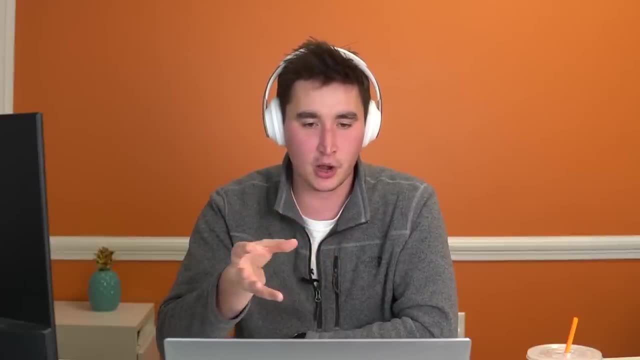 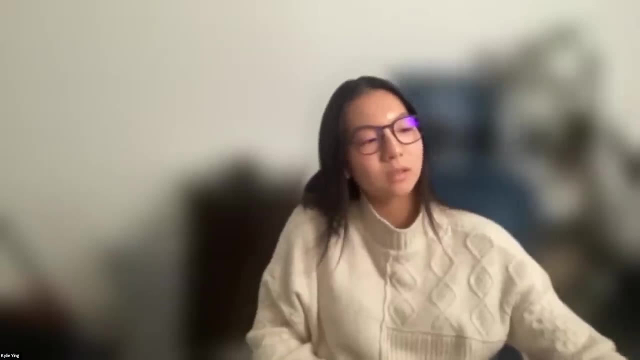 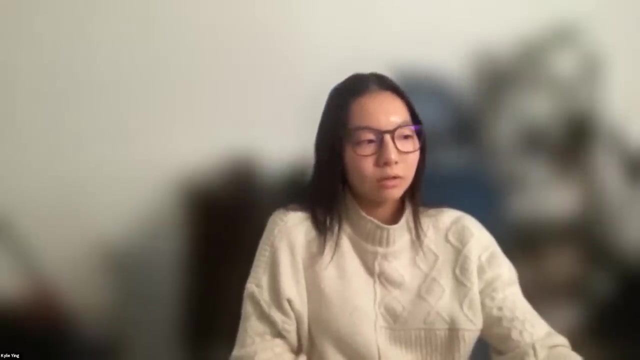 guess the premise of the question and like just the flow of that type of interview. um no, i do think this was a very interesting interview because it's not straightforward, right? it's not like i can just mention the various features that i would put into a model, like i do think. 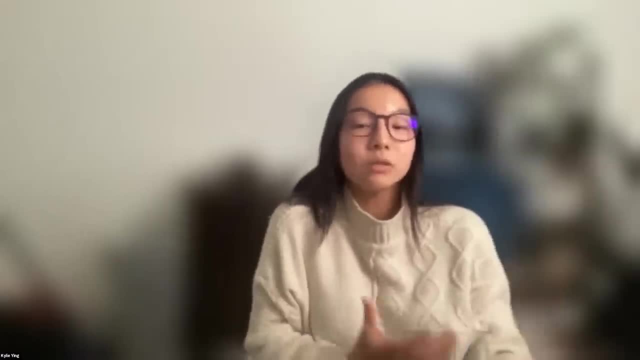 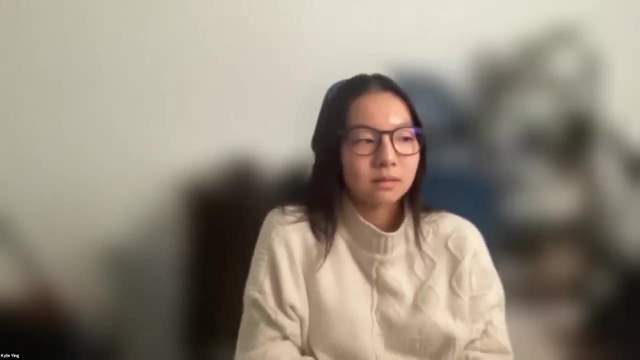 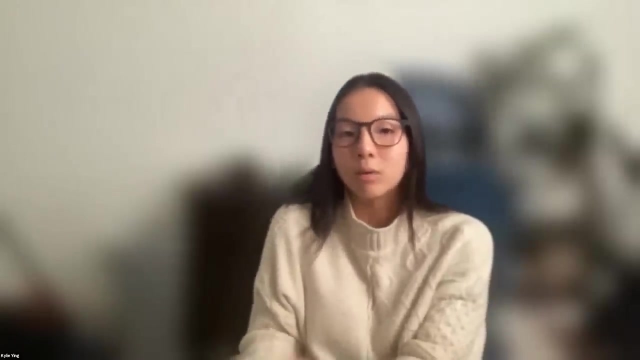 that it required some time to think about um. i do think it was very open-ended and i think that's good in some ways, because it forces me, as the interviewee, to ask for specifics and um, and you can. you would tell a lot about a candidate by the questions that they do ask. 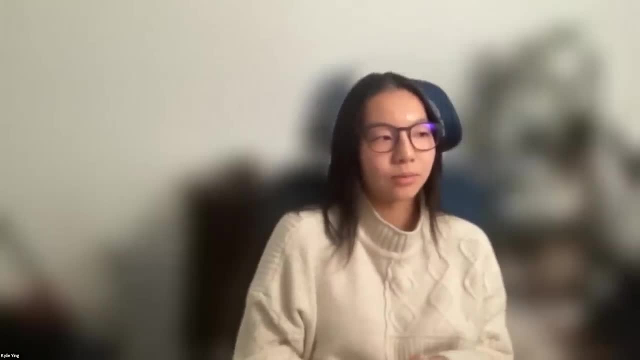 and i also think that, for example, when i was trying to go through, you know what would this data set look like, or how would you approach collecting that data like. i do think that, um, the one tricky part that i kind of faced was after i did this like naive labeling system, you're like 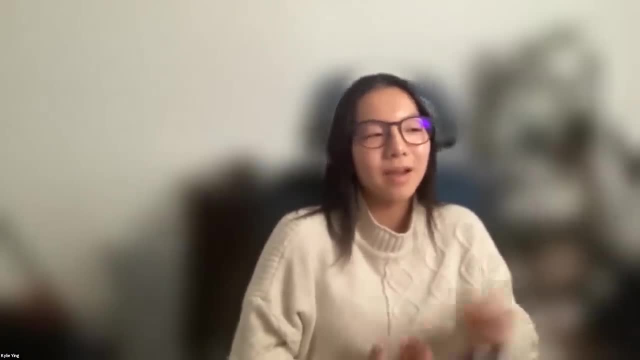 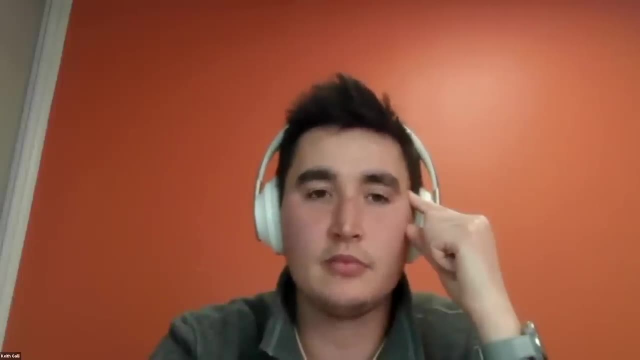 well, what is what is wrong with that? and in my head i'm like: well, obviously you can do something more complex, but like i think as a candidate, you can do something more complex, but i think as a baseline, like there's nothing wrong with, like what i said, right, because it just depends. 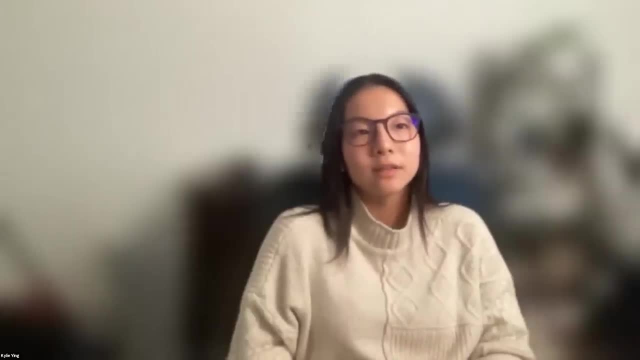 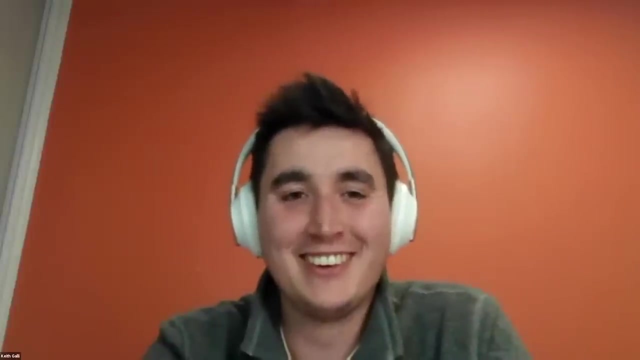 on where you set that threshold. so i would actually- unless an interview interviewee is like blatantly wrong, i think from the perspective of an interviewee like i don't, like i'm also under stress right, like i don't want to, just i don't want to hear like, oh, that's wrong, yeah, um. 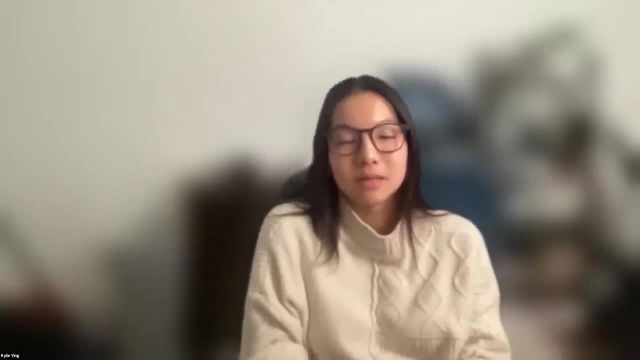 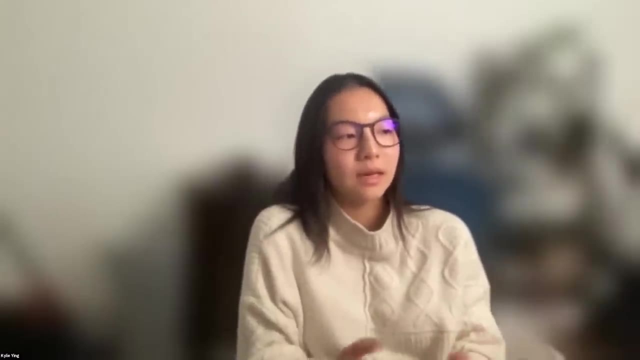 you didn't say it was like wrong, but you just said: oh, there might be some flaws with that, like, like, can you think of anything? and so i tried my best to think of some things, but i do think that, like, maybe if you had said: well, this, you know, user feedback is really great, but can you think of? 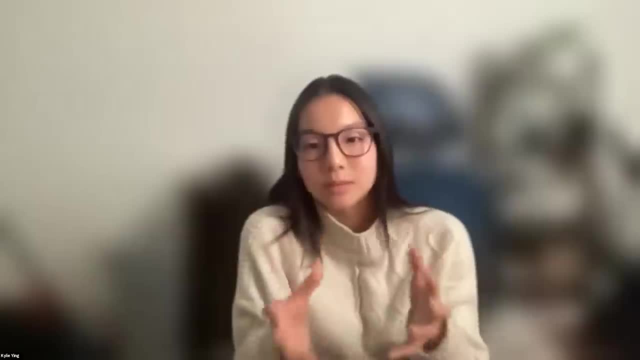 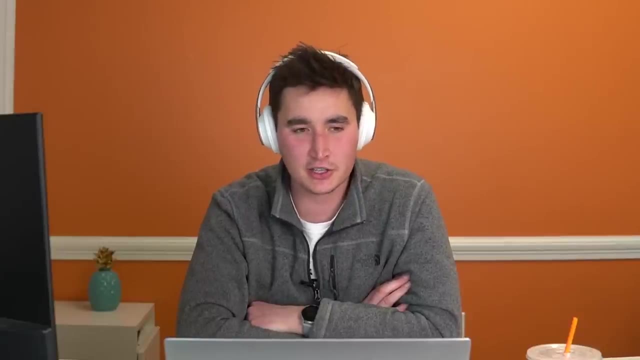 anything specifically with, like, this specific part of that, that things might go wrong, or something like that. yeah, i think the issue, the challenge, is a balancing act. it's like, on the one hand, i don't want to be leading, i don't want to like be like, hey, you could think about this specific. 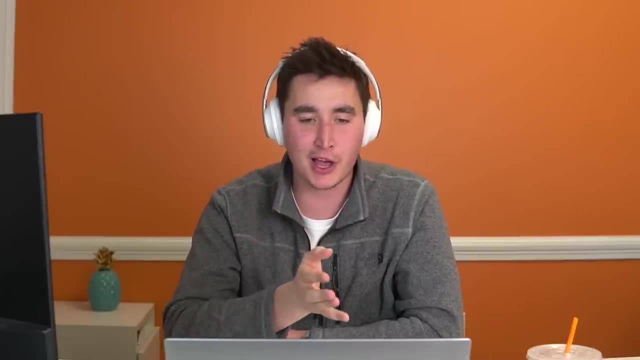 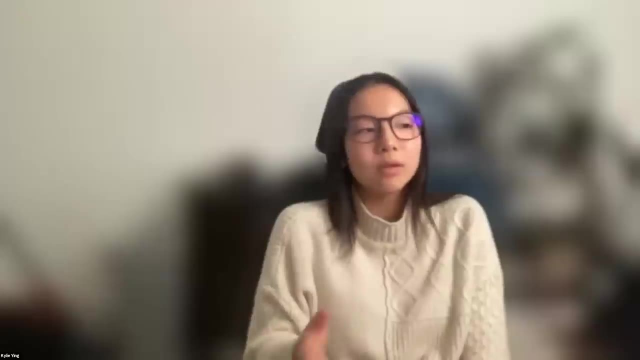 thing. so i try to like: i think maybe i could be more positive. uh, instead of saying what's wrong, you know, just saying how can you improve this and just leaving it at that. i think that would also be good, because i think when you said like like there are some flaws here, it made me think like, oh, this system is just 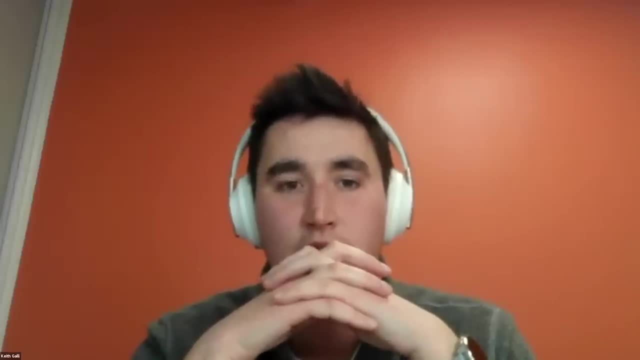 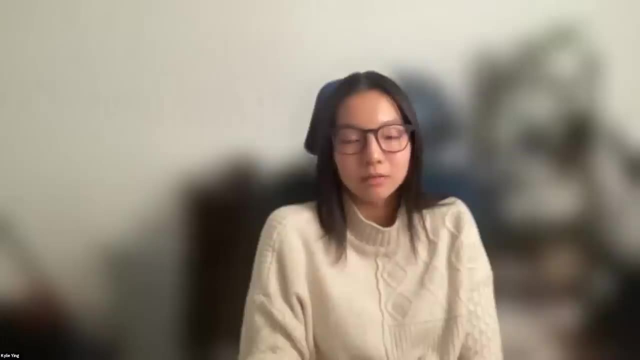 like yeah, like i should just not be using um like reports of spam, but like i think that you genuinely should be using reports of spam if you're trying to label your data right. so i think, like i think that's a way to improve upon this system, that would make me think, okay, i'm on the right track. 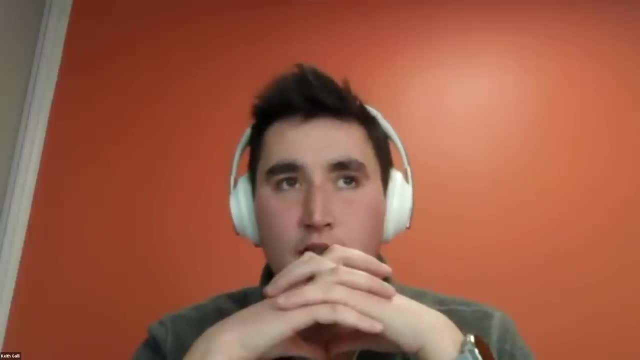 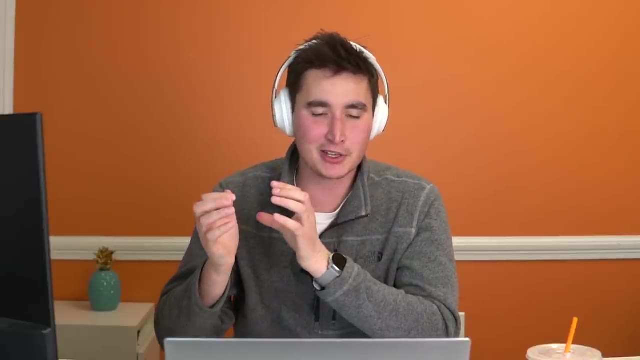 but, yeah, what are some flaws that i can think about there? yeah, i definitely agree with that, i think. just one note to add too: i think that from an interview perspective, i think that that's the best approach that you, what you mentioned from your perspective, one thing that you could. 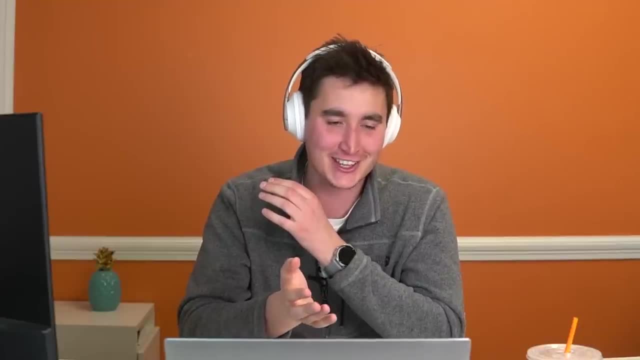 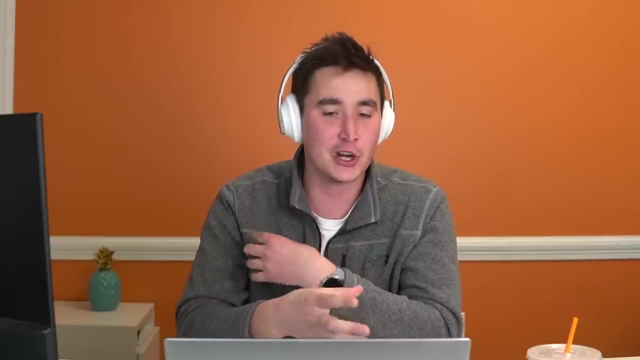 potentially employ and whether or not you want to do this, it's kind of up to you. i've seen this before in real interviews. that i've done is like you're welcome to push back at the. if you do it in like a, you know, a- i don't friendly is maybe not the way, but like in a professional. 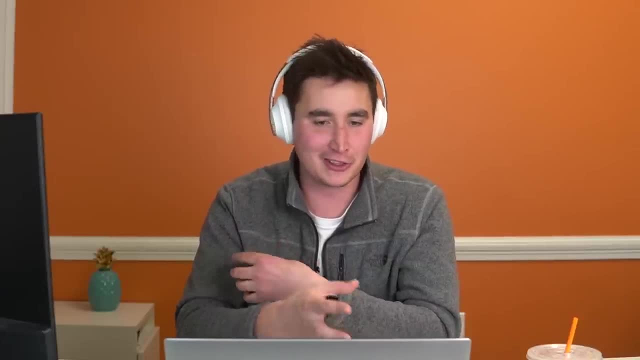 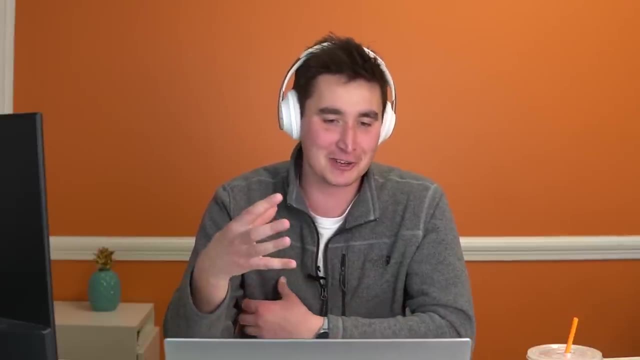 way and say actually i think that this is a fine, like i don't think there's anything inherently wrong with this. i think this is a good baseline approach. we can improve it, like you can kind of spin it that way too. obviously with nerves and stuff it's tough to do that, but like i've been 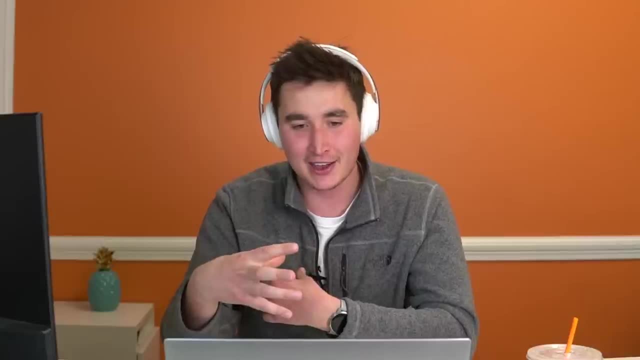 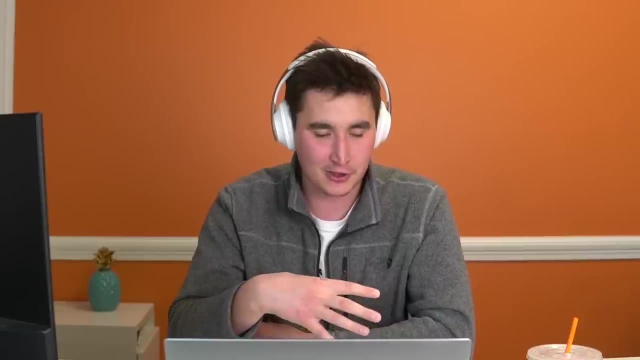 at an interview where we, like we kind of got into a debate, but in that i learned a lot about how they think that they're willing to stand up for what they believe in. and, like they weren't ever aggressive but they were able to, like, stand their ground, argue their points, but being willing to 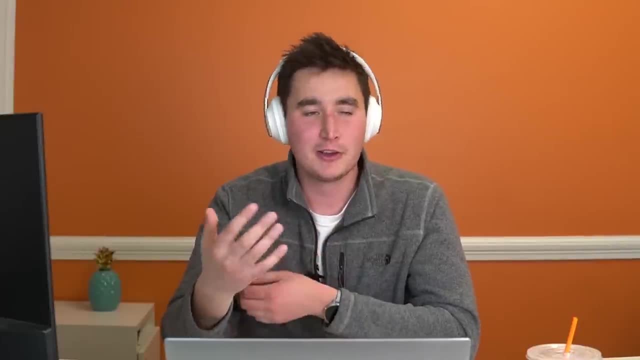 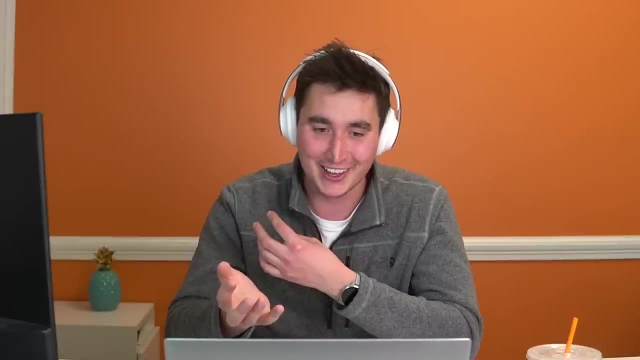 listen to my side and like kind of we could come to an agreement. so whether or not you want to play into that, you know, is up to you. sometimes interviewers might be cruel. they might purposely get your nerves and be like, make you think you're doing something wrong, even though you're not. but 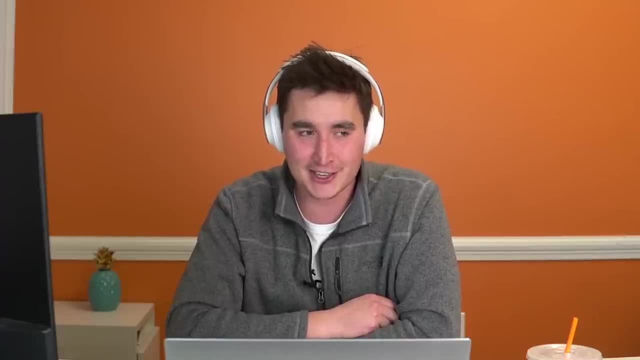 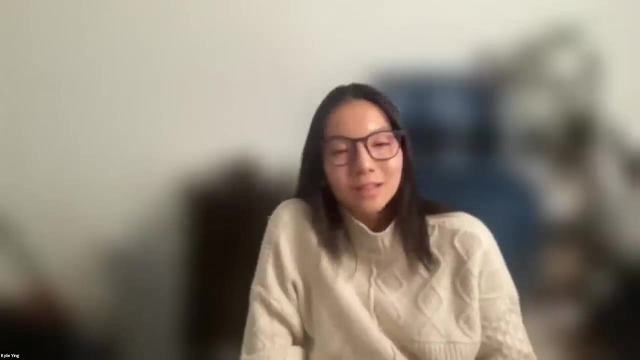 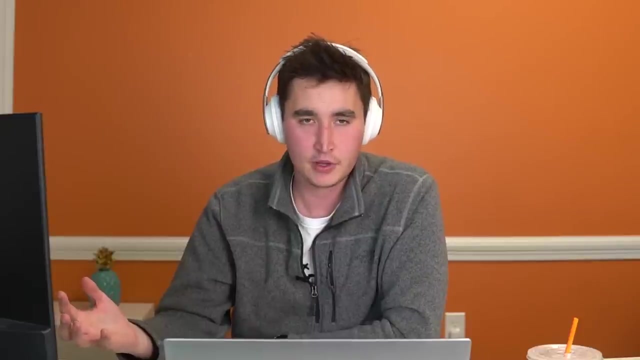 uh, yeah, it's an interesting, i think, from both sides- the right, you know it's a chess match a bit there. um, yeah, no, i agree. okay, i don't have anything else. yeah, so from my perspective, just to add some details, i guess i mean overall, like i mean some high level things, like the reason that i would approach an interview. 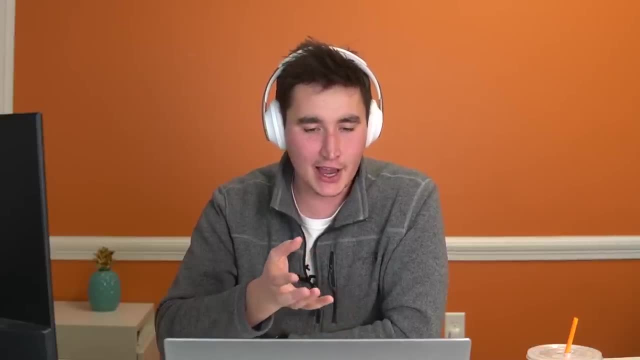 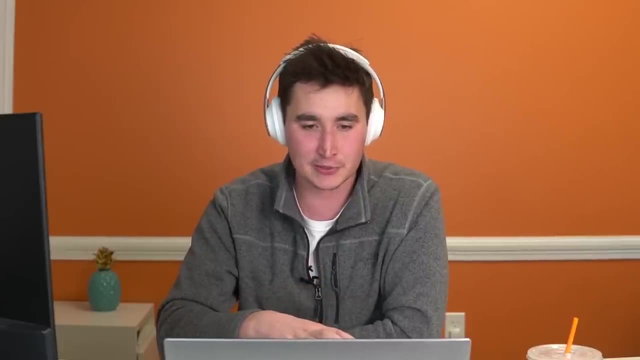 like this is because, if this is like a high level position, i assume you know how to code. i assume that you know, like the fundamentals that you can program, that i'm not worried about that as much. i'm worried about how you are as a thinker, and not even like how you are as a thinker, but also 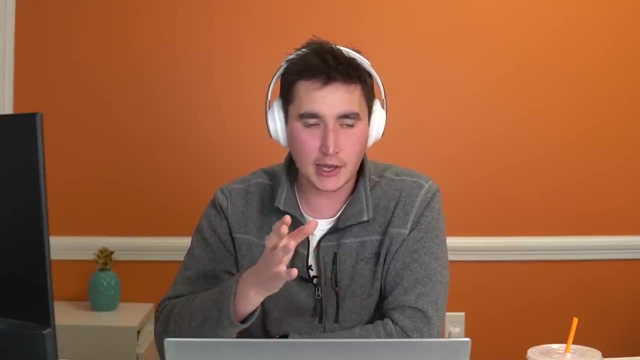 how organized are you as a thinker? because i could potentially interview someone that's very brilliant. but they might just kind of ramble on in a way that i can't follow and i just like, even though i understand they know that they're talking about, i just i need to think about it in the context of a bigger team and if they're not being 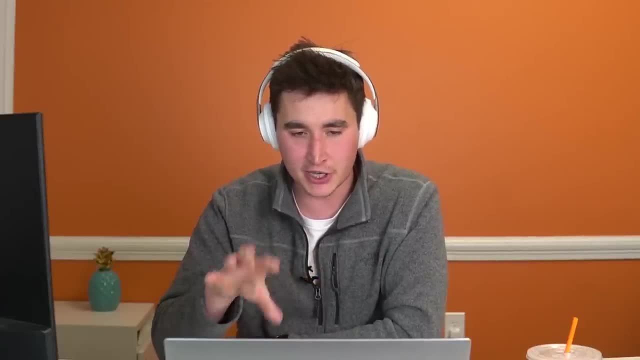 straight to the point and like being able to flesh out in a way that's easy to follow their points, then that's not probably someone i want to work with, even if they're brilliant. so i think you know some of my first comments is that i think you did a great job at like not only 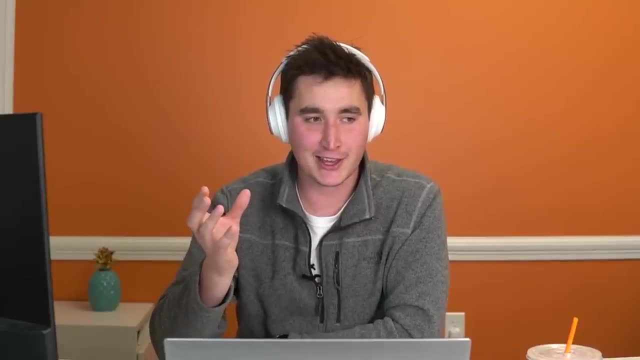 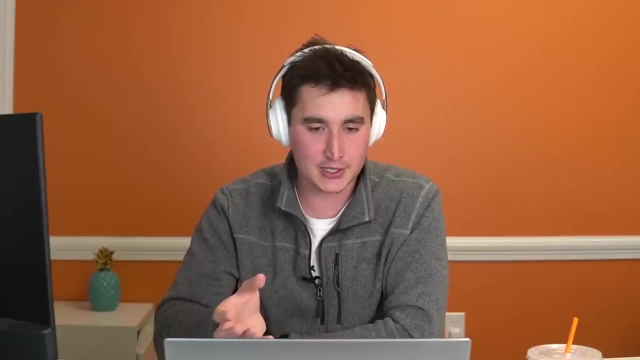 explaining your points, but also like being able to explain your points concisely, i think, once you started having to write down the google doc. one thing i really appreciated- and i don't always see- is like you are very cautious to format it nicely, which is a big thing for me as a reviewer. it's 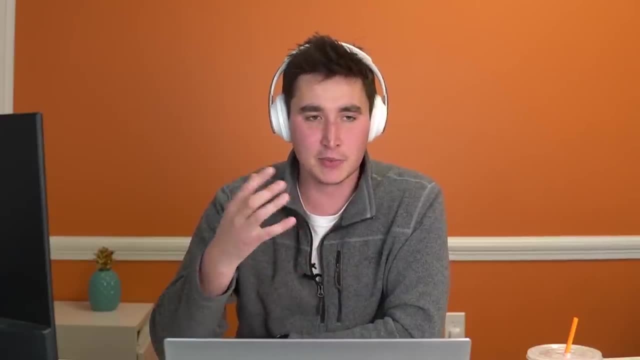 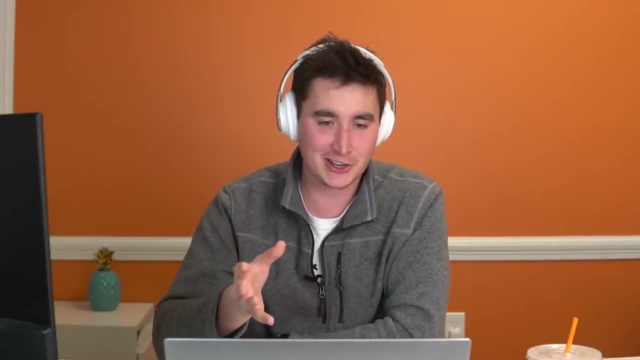 like a small detail, but i think it goes a long way where it's like it makes me. it makes it easier for me to understand things. it makes it easier for me to under like follow up on certain points. so like structure there is good, solid, like formatting and all of that, so like 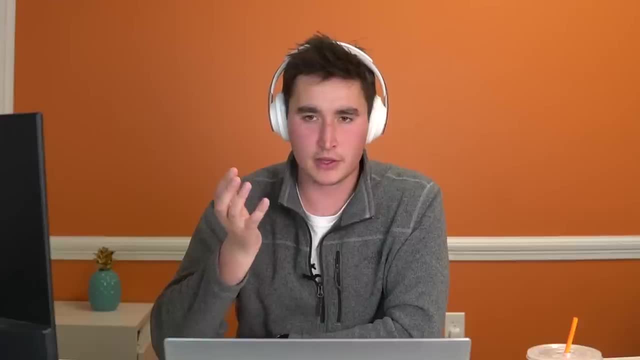 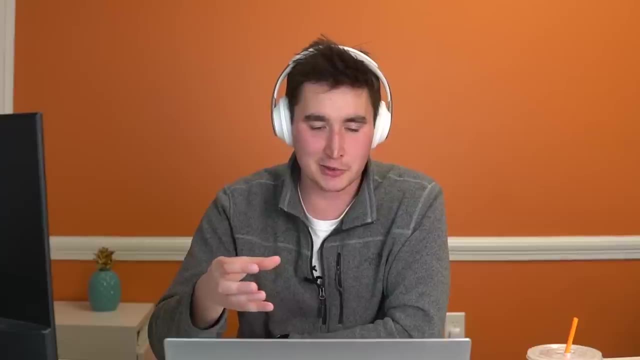 yeah, all solid there. i think overall, like, i think, a lot of just good discussion. i think you got to a lot of points without me even having to prod to that. it's like you kind of got to some of the like crux of like, oh, these are the features. i want to do a, you know, build a feature vector of. 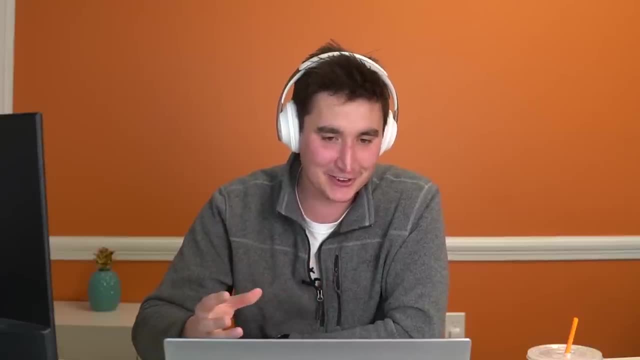 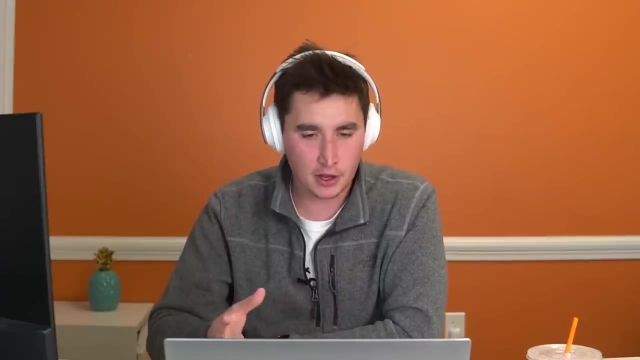 all this stuff and like i had specific questions, hoping that you would get to feature vector and stuff, but you kind of just brought it up on your own, which was solid. i think it was a good use of like thinking out loud, like making sure that you're going through your thought process and 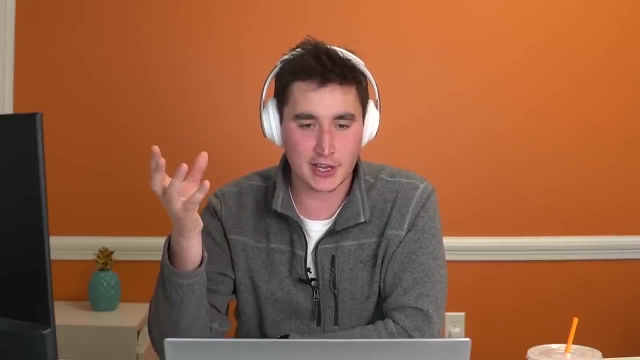 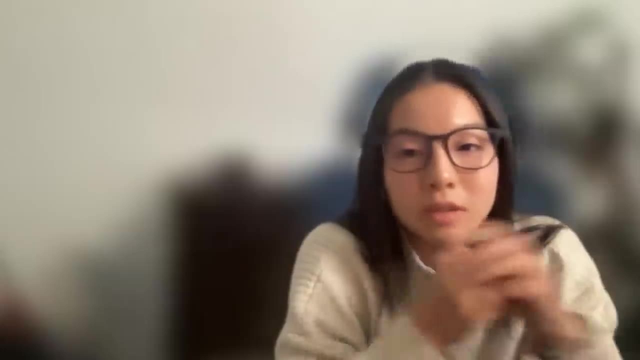 like you know saying what you're thinking as you're, you know writing it out as you're saying it, like just it allowed for more discussion, allowed me to see how you think. well, i definitely think that, like so, because this is being put on youtube. i definitely think that. one thing to mention that 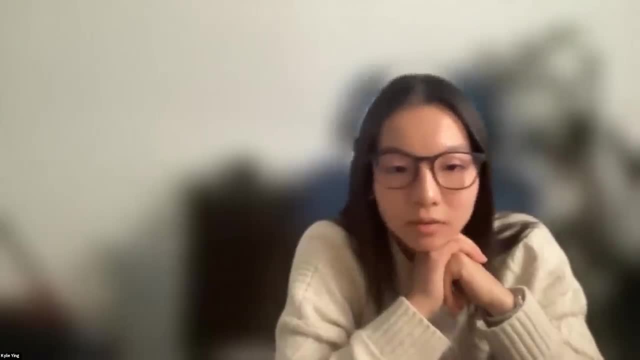 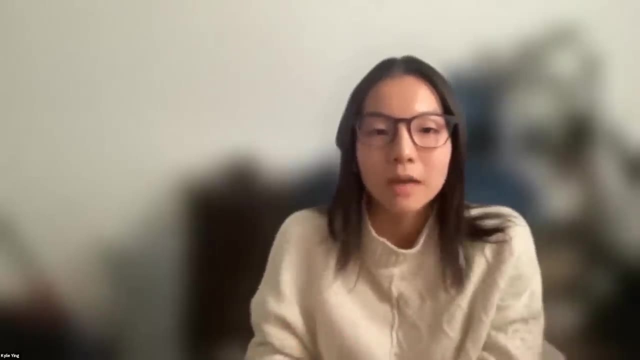 like people who are kind of newer to peck interviewing and stuff like that, like i. i don't think it's common knowledge, if you're new to this space, to talk out loud during these interviews, like i. i don't think i think a lot of people just think, oh, they asked me. 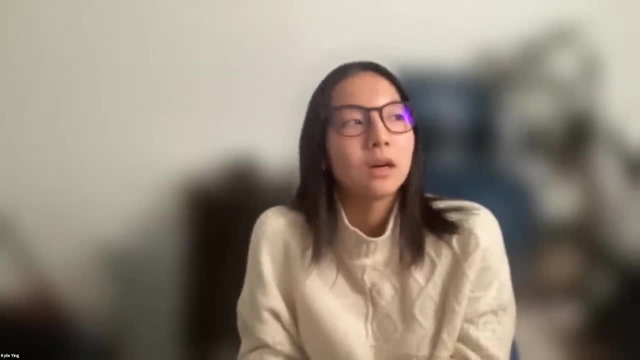 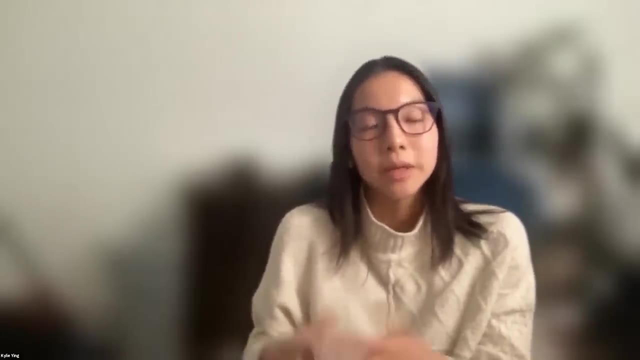 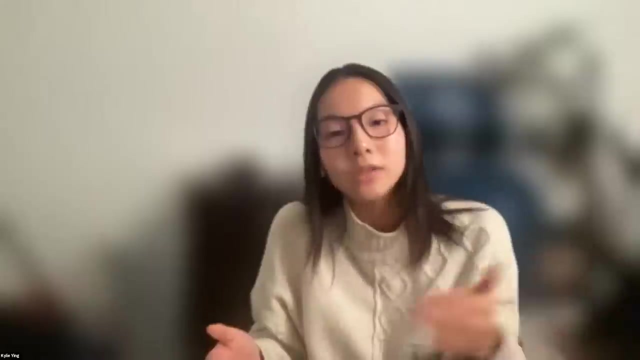 this question. i just need to get the answer. no, like you need to. um, like, what they really want to know is how you think right, not whether or not you'll get to the right answer, because what an interview should, what an interviewer hopefully should- be doing is, if you're going on a completely wrong path, kind of guide you. 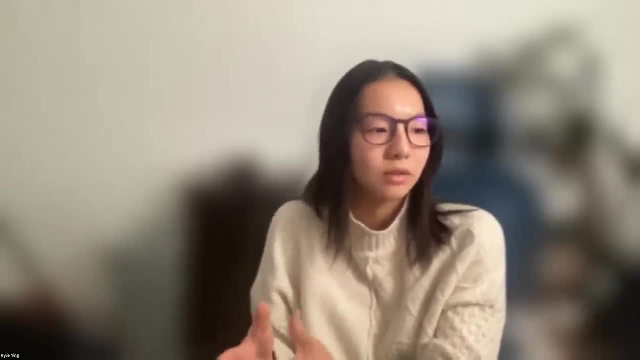 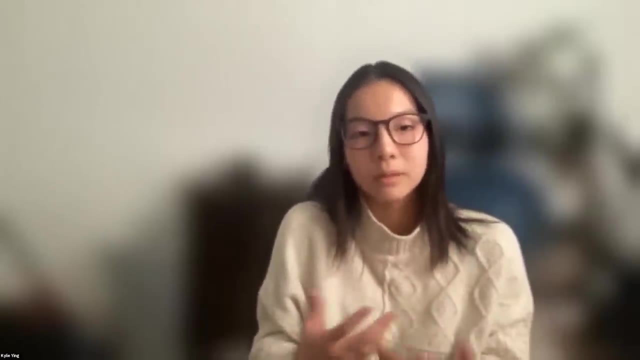 to the like right answer, right. and i really enjoy interviews where it's more like a conversation, where i'm not just talking to myself, where i can bounce ideas back and forth, because that also with me, like this, is what it would be like to work with this person on a team, um, so you really want? 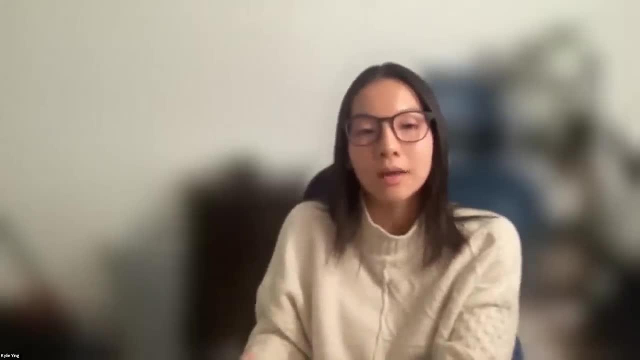 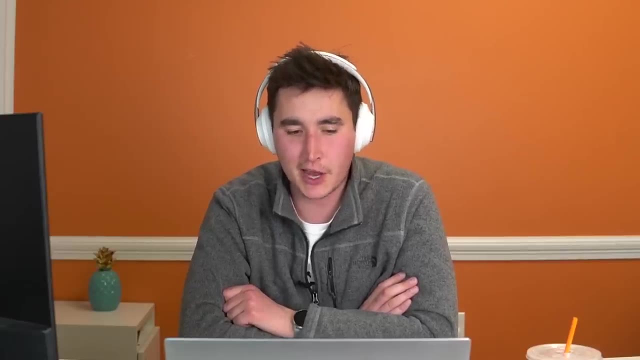 to be able to display how you think and how you arrive at the answer, rather than just saying an answer and then justifying it. yeah, definitely, yeah, i think that's great to pull, you know to bring up. i think that it is kind of weird. it's kind of different and new same thing with like. 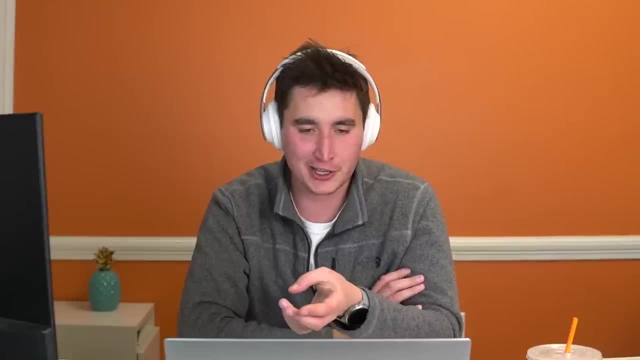 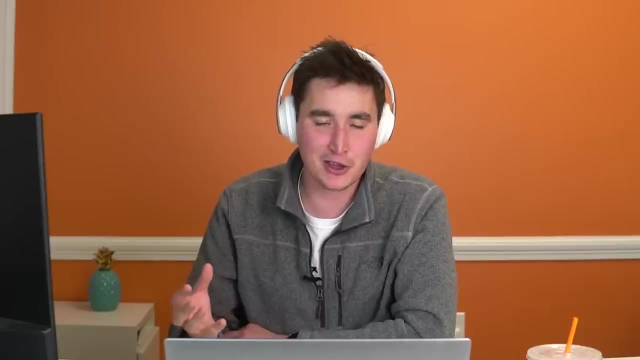 writing things down during an interview, like we use google docs here, but like traditionally, if this was in person, like it'd be a whiteboard or something, i'm like- i think some people aren't prepared for that too- so like knowing that this might be what you have to do, but i think yeah. 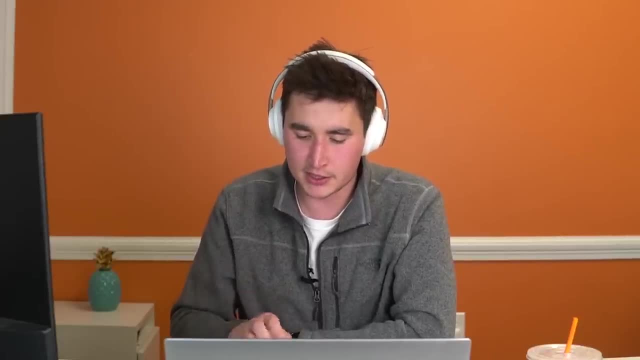 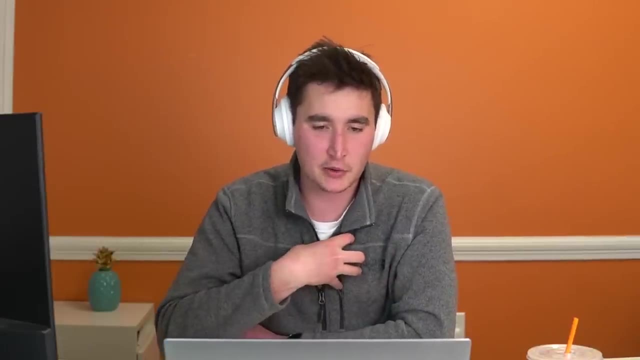 speaking out loud is super important. um, let's see what other notes do i have here. so some like small details, like overall, like from my perspective as an interviewer, like i thought you had a solid performance, like a a like good performance, like i'd be excited as an interviewer. 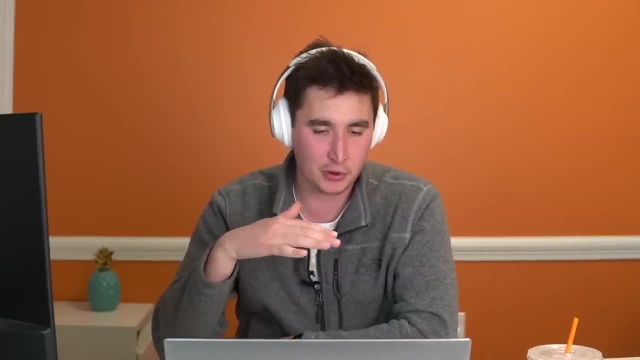 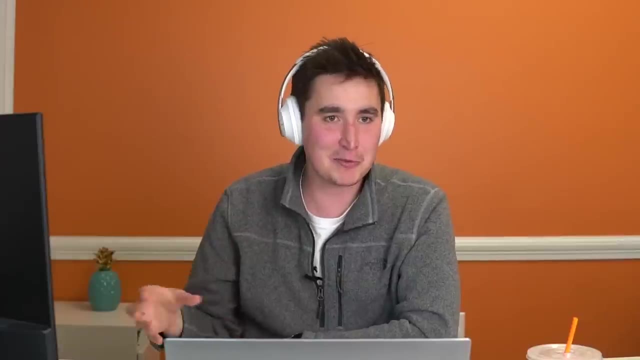 to come out of that interview like, like this person hit the main bullet points that i had. so, like you know, it would really come down to what do the other candidates look like? But like, definitely, you know, like sometimes you come out of interview you just immediately know like 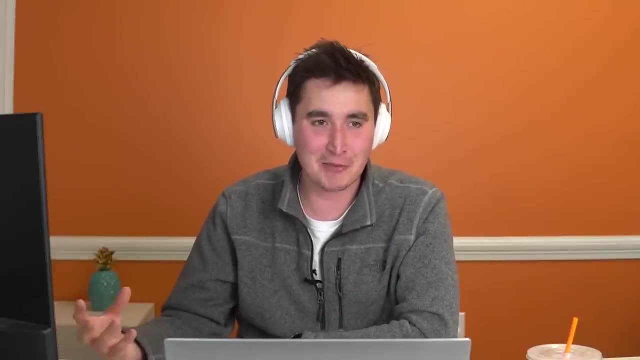 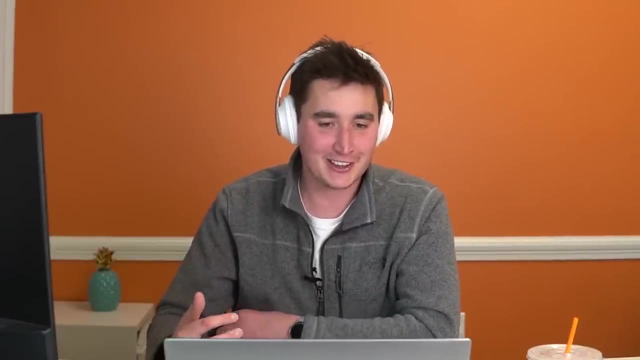 this candidate was not right. Sometimes you come out of it and you're like you know, maybe, like I definitely came out of this interview and I was like yeah, that was a solid performance. Like this person knows what they're talking about, They think clearly, So like good from there. 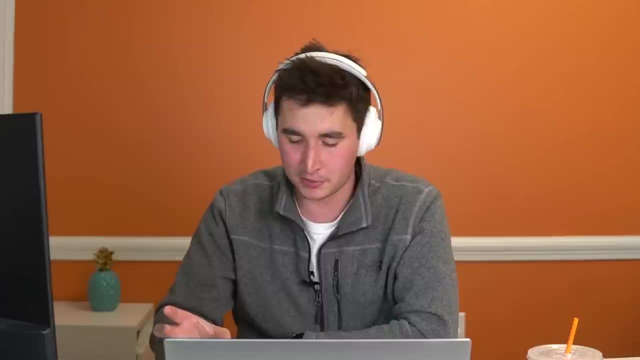 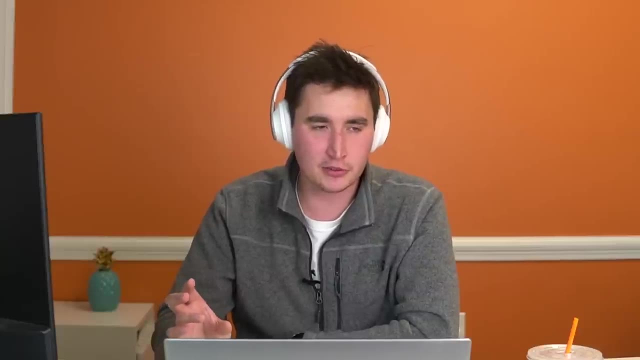 So like I'll be nitpicky on things because, like, overall good performance. One thing that you kind of did- and it ultimately was my next question, but like I would have liked to think a little bit more discussion. when I brought up the data set, you kind of skipped to the model implementation. 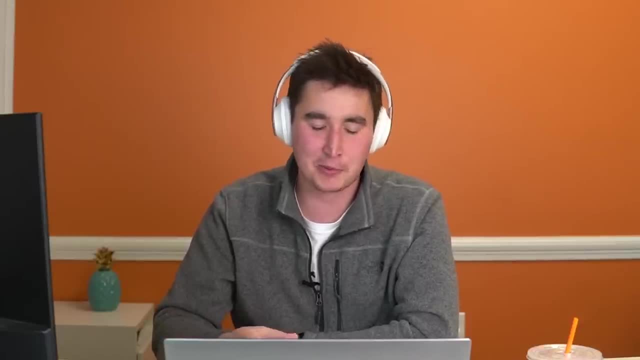 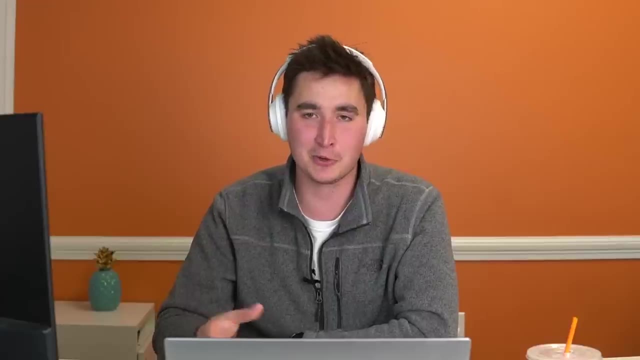 And so, like I didn't stop you, I didn't pause it and bring you back because that was the next question, But just kind of keeping in mind what the question was at hand, whereas you ended up focusing on implementation, which was important, was the next question. But I think, like I would, 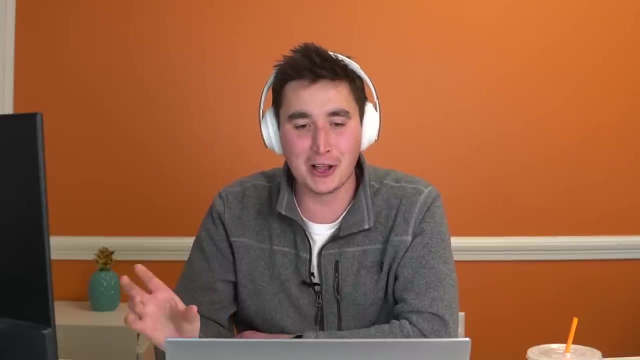 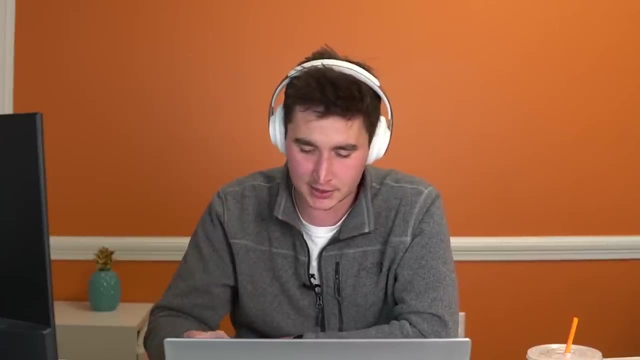 have liked to walk through that, I guess, in a specific manner. So small nuanced detail, like kind of a Annoying me being annoying, but like just something to consider, just to keep in mind. are you answering the question that was asked? Another detail: this is kind of at the end. 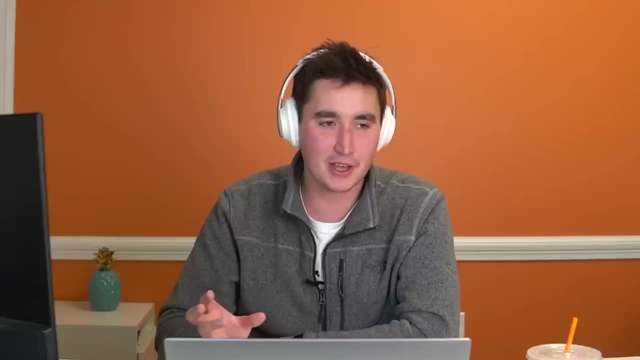 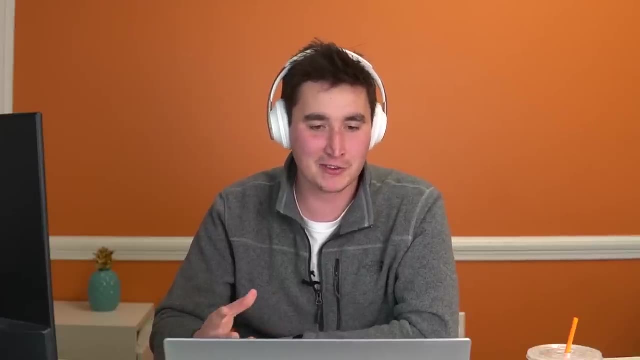 and there is like little things that I'm like bringing up. It's not like a ton of, I think, things. One thing at the end: I think it was good that you mentioned like hey, I don't have that much knowledge in the system side of things, Like you shouldn't try to lie to your interviewer. Like 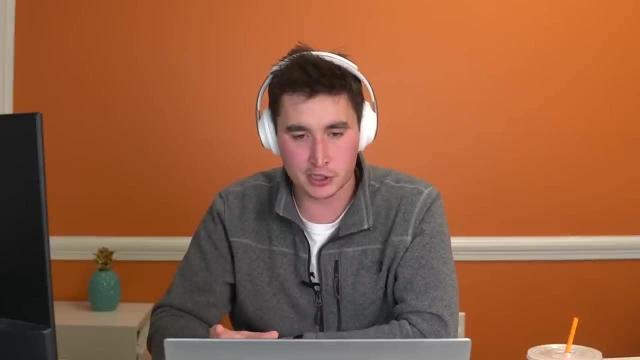 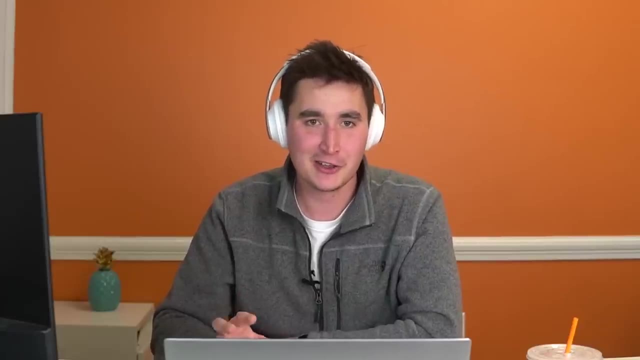 I think it's really impressive when someone knows when to say: hey, I don't know that much about that And I think that's a really good thing to do, And I think that's a really good thing to do, So I think it was good by like stating that explicitly and not trying to like you know. 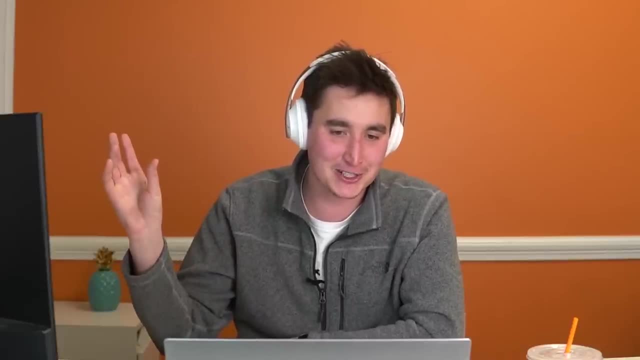 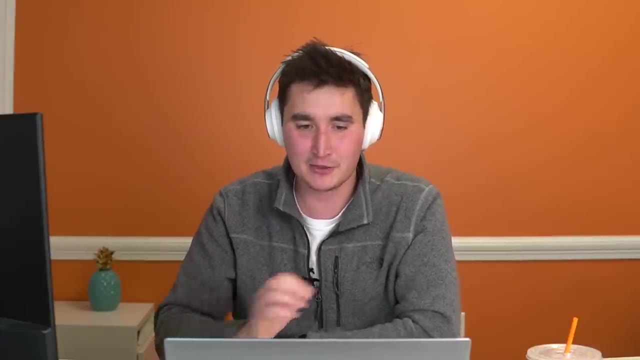 spin off some information on random cloud services that you actually don't know much about, Because I might ask you details about those and then you might be like I have nothing, So it could catch you in a weird situation. I do think that when, So the reason why I brought it up there. 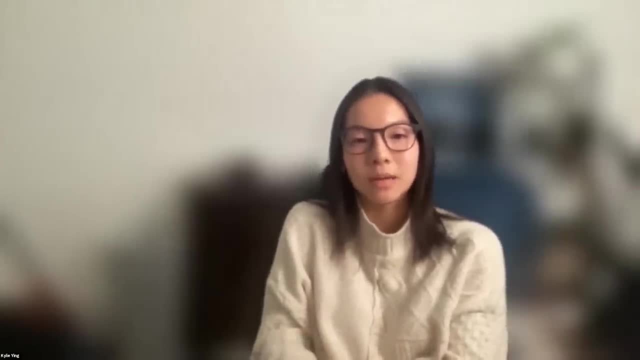 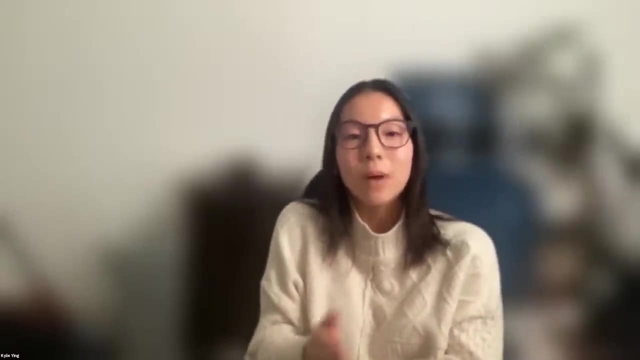 was because you asked a specific question about the deployment of this right. Like I would never have said it myself, Like I don't know that much about this, But it was literally just because I asked a specific question that I do not know the answer to, that I brought this up And like: 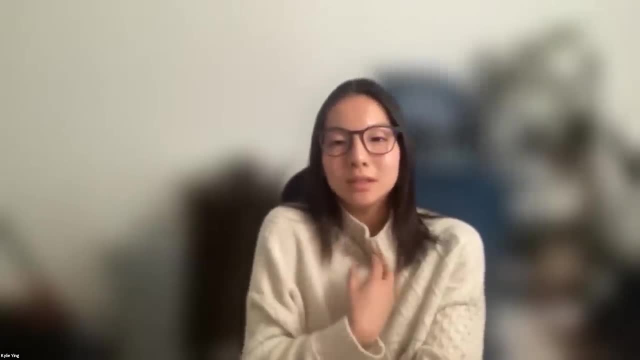 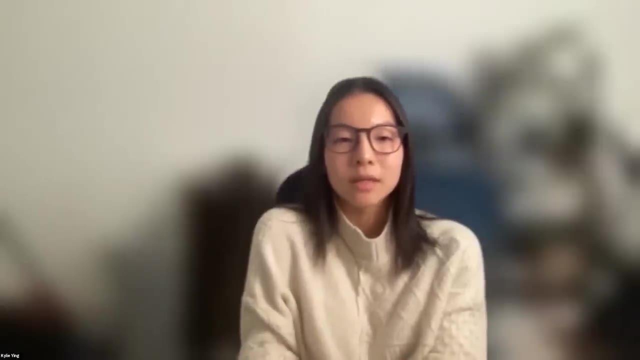 I don't think like I think that, at least to me when I used to interview people, like to me it's, it's okay if somebody doesn't know something, right, Like what I want to see is that. 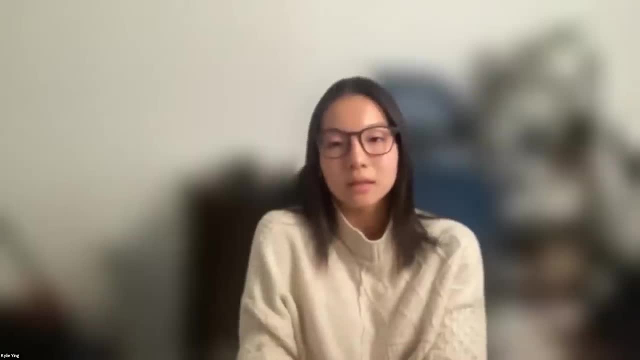 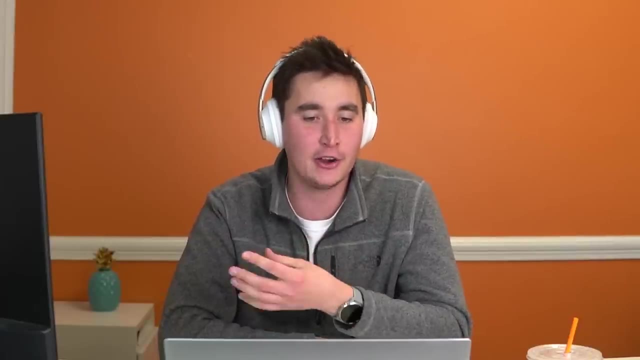 they're teachable and that they can learn and that they can think. So yeah, and I think you bring up a good point though, because you're kind of point is. I asked you about it And you said: I don't know much, You don't want to call attention to things. 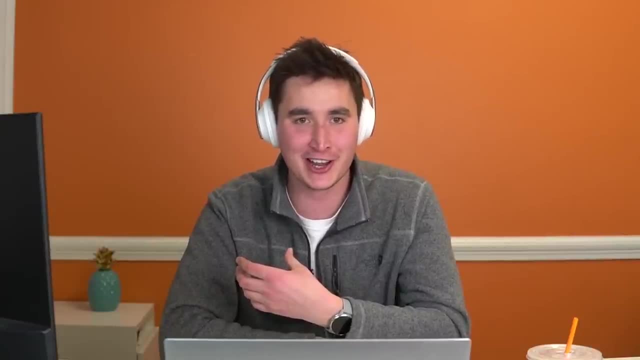 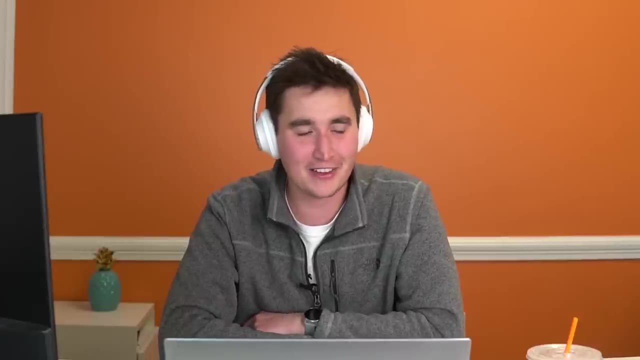 that weren't brought up. you don't be like, Oh, I'm actually like a junior engineer, Like I don't actually like know that much coding, like don't bring up things. Yeah, I definitely see that sometimes in like interviews that I do bringing up things that they should. 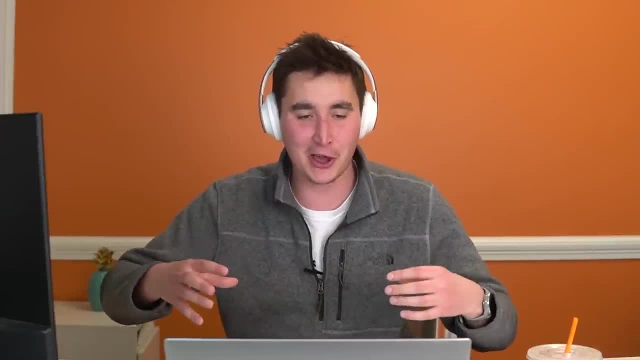 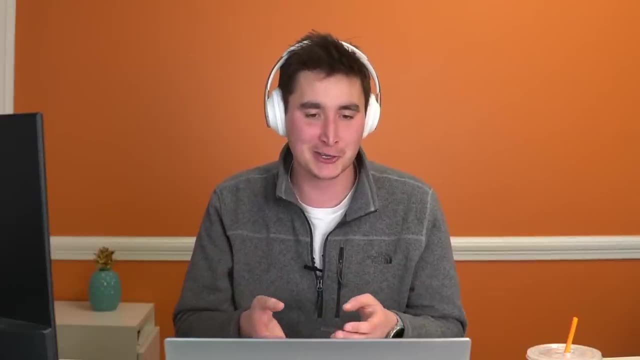 bring up: like be very confident, professional, like know your stuff, fake it till you make it And, if they like, bring up something specific that you know you can't talk that much about, be honest, but don't throw that out on your own. like, let them bring it up. 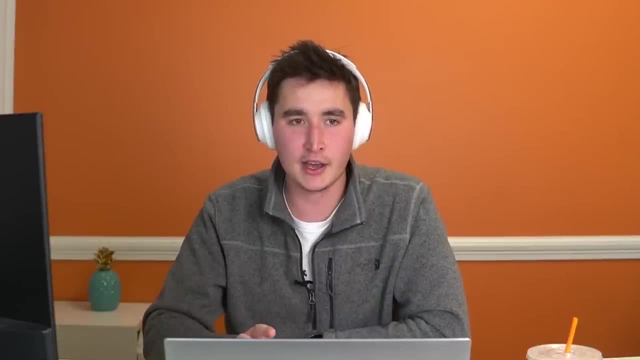 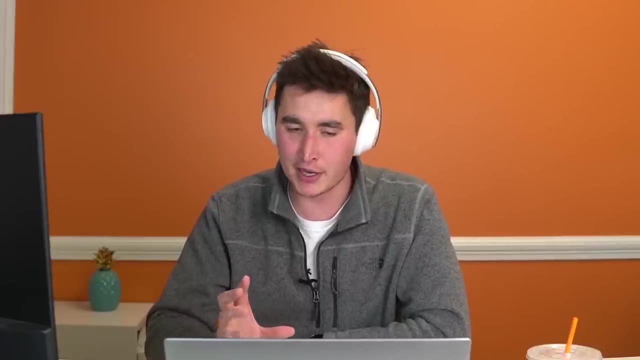 So some things that could improve on that idea I think that it was good mentioning of. like you know, obviously we're gonna probably use a GPU, probably going on like paralyzed things. I think one thing that might have been interesting to say upon that type of answer to dive into some. 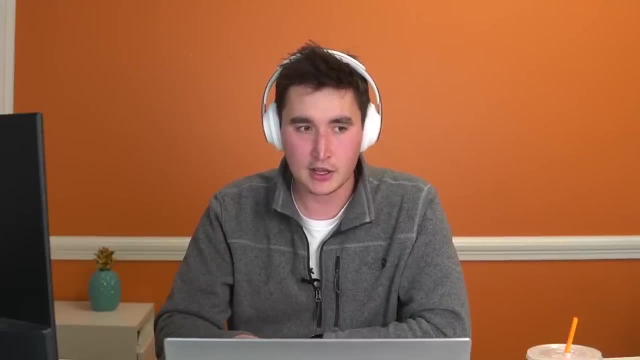 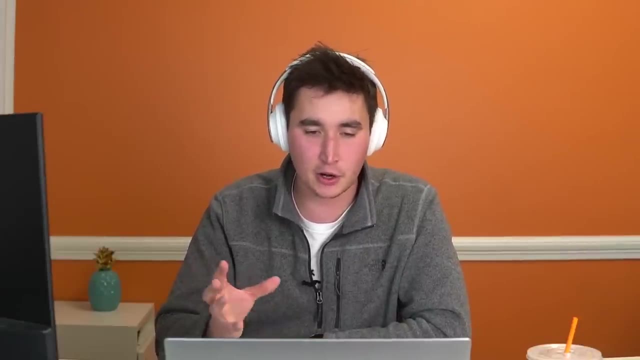 of the more technical details is, I think, that we would maybe just explicitly kind of mentioning, like tokenizing maybe, some of these tweets and whatnot or whatever you want to pass into the system, But also, I think, a big thing that you could have you know, you could have you know. 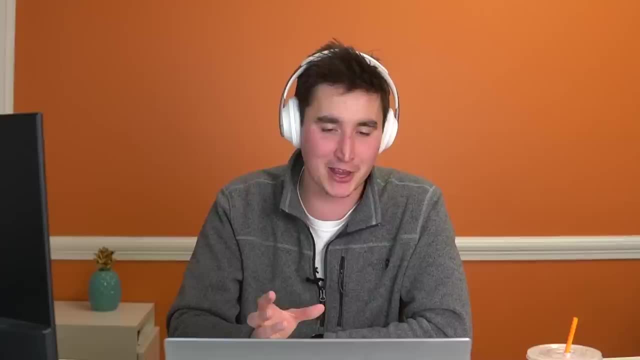 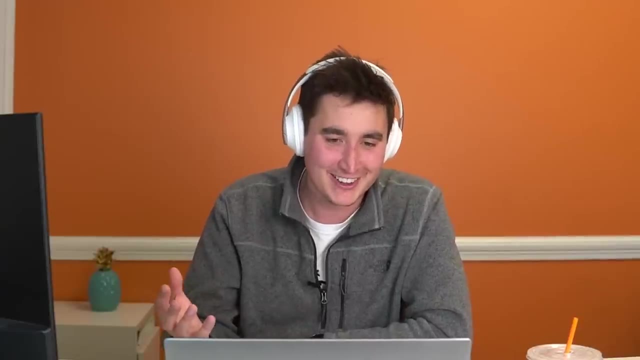 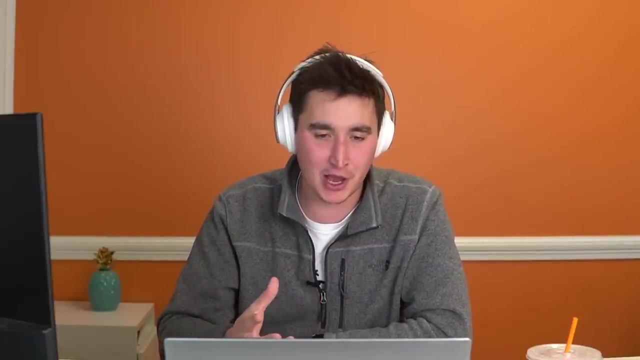 brought up was like batching And just explicitly mentioned like. you probably don't want to take one tweet at a time because that's gonna like, like. if we think about all of glitter as a parallel to Twitter, obviously there's so many tweets happening, there's so many potential bot. 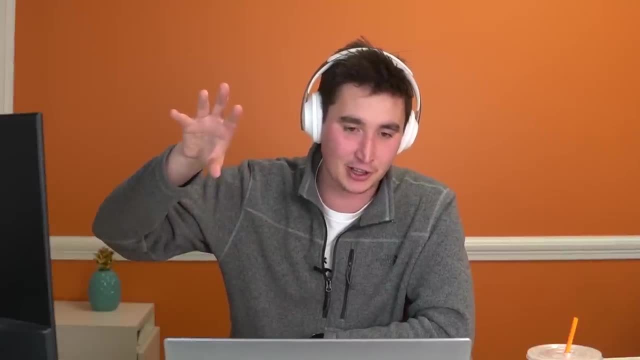 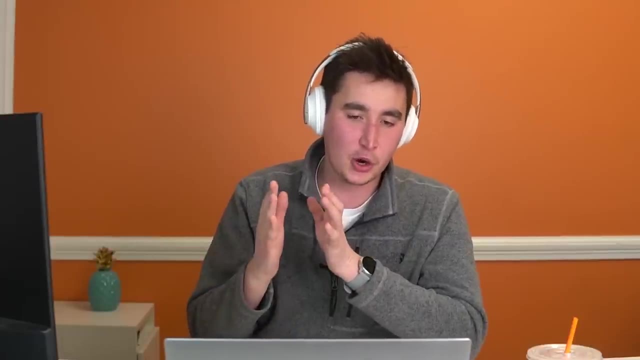 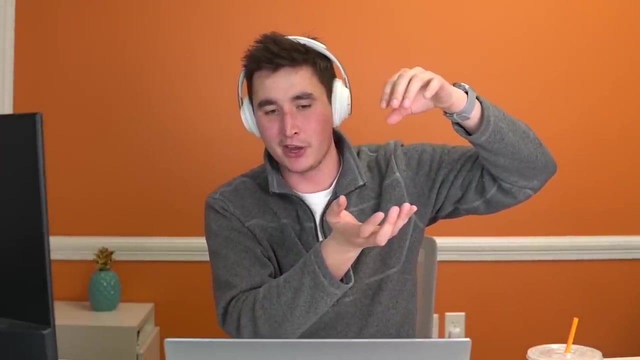 accounts that if we were trying to handle these on an individual level like it would just be in crazy, like intense processing. So we would need to, like you know, maybe we have a window open for five seconds or something that like collects a big batch of these, and we have our model set up in such a way where it can process. 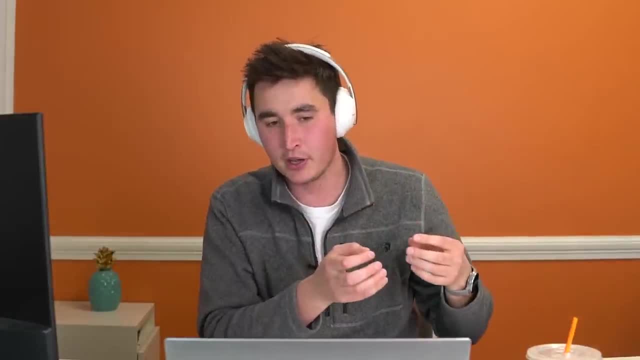 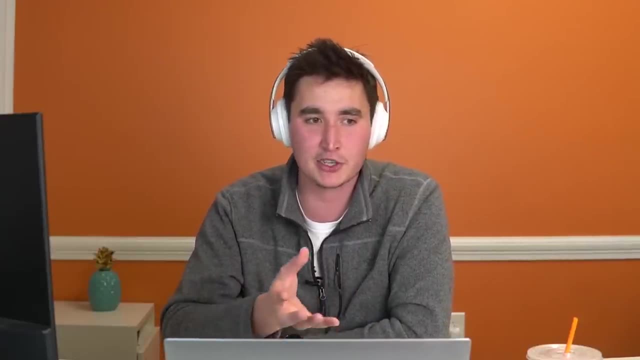 that full batch and spit out that output, and then we have to parse that output. So that would be like, I think, one way to improve that- but I think it is on the deployment side of that is. you know, maybe not your expertise, but I think the batching could have been something interesting to bring up. 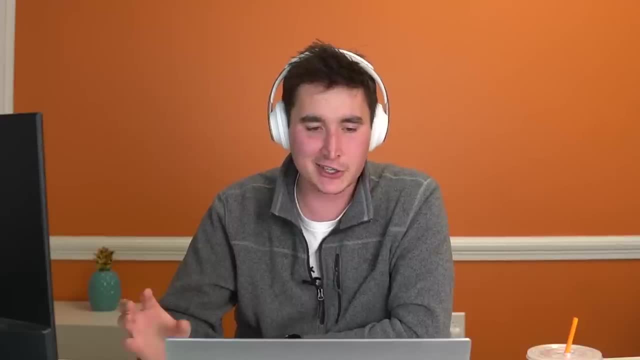 I'm trying to think of other specific components. I think the challenges I like when I'm in an interview with two people, where one person's writing the notes and one person's really leading the interview, Because I think one thing that's challenging sometimes is 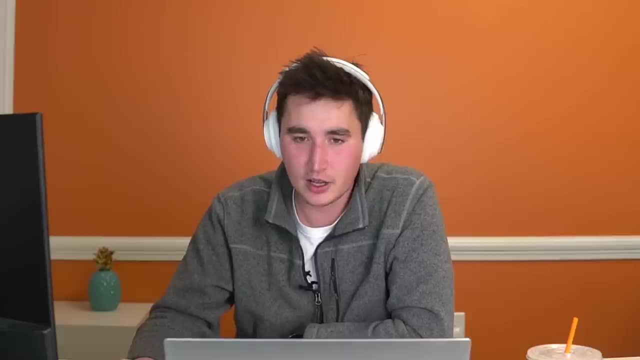 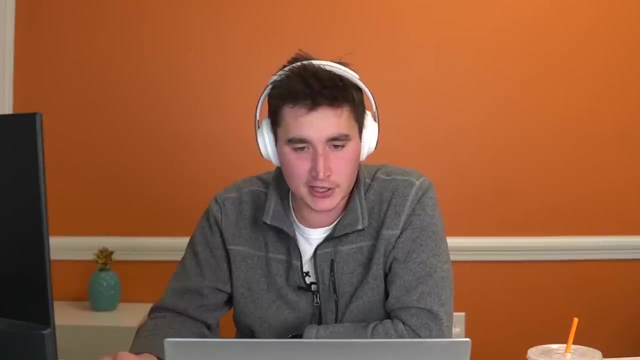 writing those notes down as you're trying to listen And let me see I don't have too much like, I guess, specific like criticism that I wrote down. I might like review afterwards and provide additional things other like positive notes, you know, for people listening and whatnot. 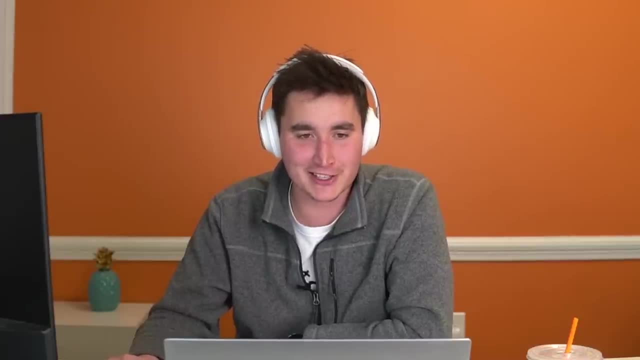 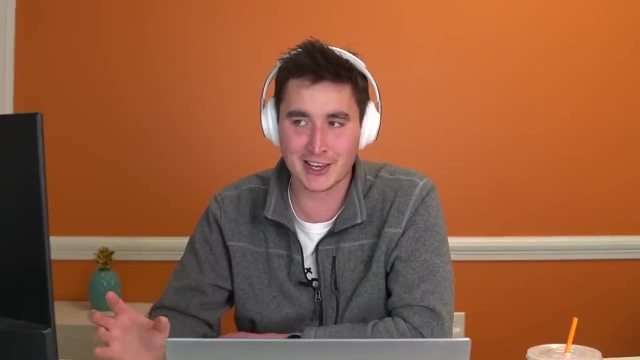 Like I appreciated when we talked about, like you know, anything that is exciting to you. I appreciate it that you kind of like didn't just go chat GPT. you kind of like mentioned chat GPT because I feel like that's. 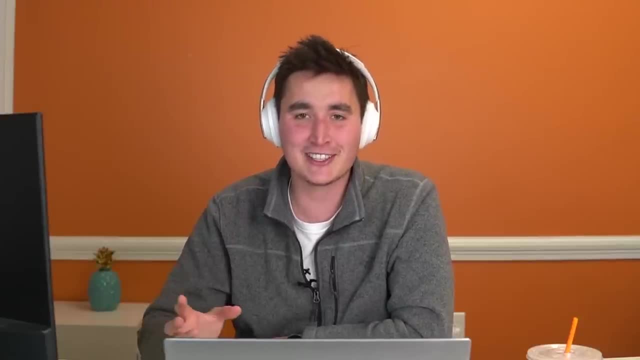 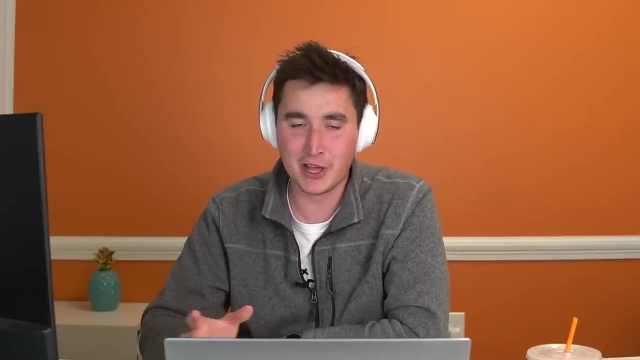 right now what I expect everyone to say. So it was nice to see some interest. that was aside from that. that was unique and different. So, like you know, you don't want to blend in with every other candidate, Even if you want to say something like chat, GPT offer something unique and different. 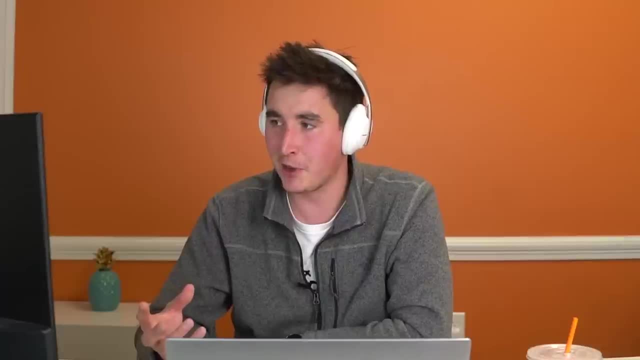 that someone's going to remember you by, And I think that, talking about reinforcement learning, talking about, you know, superhuman chess, AI poker, AI spins around a lot, but I think it's spins up a more unique conversation. 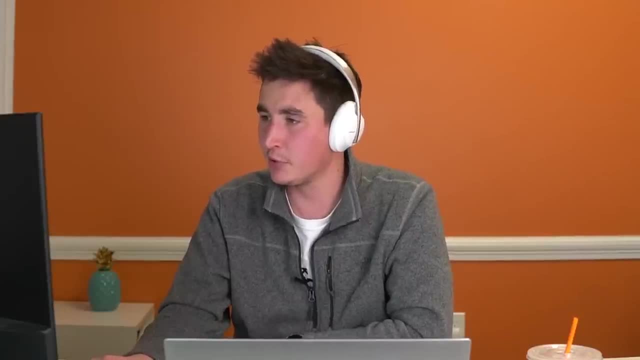 Other, I guess potential thing that could have maybe improved things a bit- And maybe this was lack on my part of like I call this a question- was it wasn't a question So it wasn't super clear. But I think there's some other- I think problems with bots that you maybe could have. 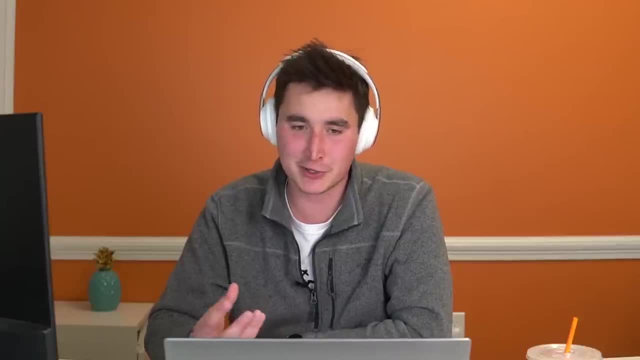 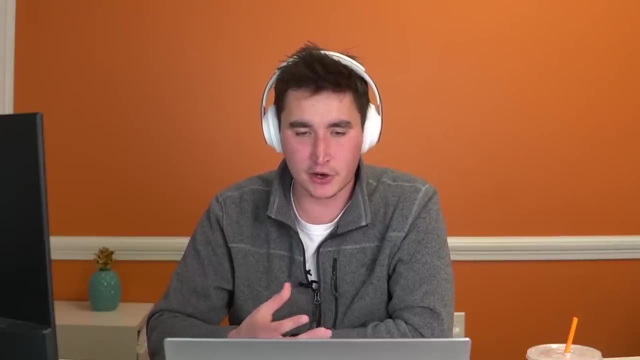 brought up. I think you didn't add that much new details And this wasn't a data science question. But from my perspective as an interviewer, I'm going to challenge your domain knowledge. Like if you're at a company, I expect you to. 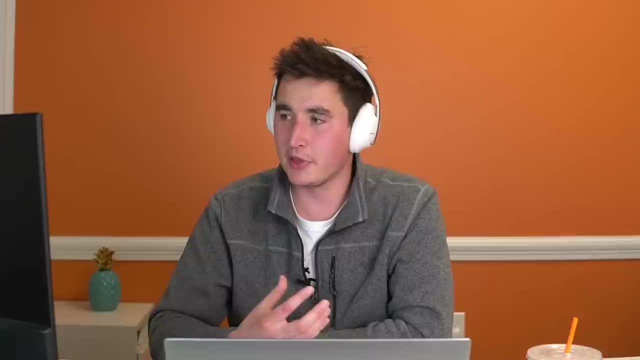 know a bit about the company, right. So, like some of the things, I think that potentially I think there could have been other, I guess problems with bots that could have been brought up that were kind of specifically unique and different from things that I brought. 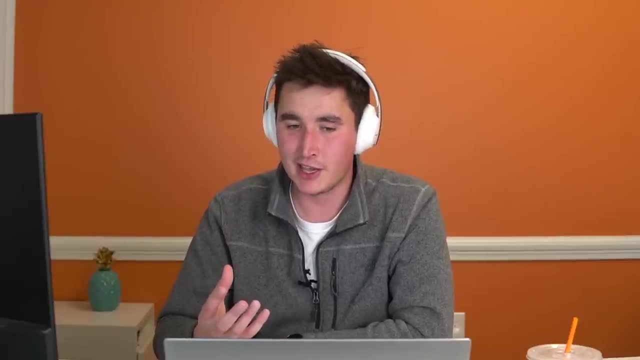 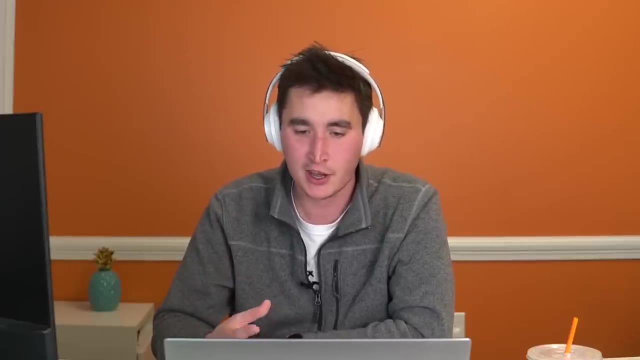 up Like. one thing you could have even mentioned is like it might hurt our metrics. we might, you know, if we have all these bots like it's hard for us to report accurate metrics to people like advertisers that you know might need these accurate metrics to you know, be able to, you know. 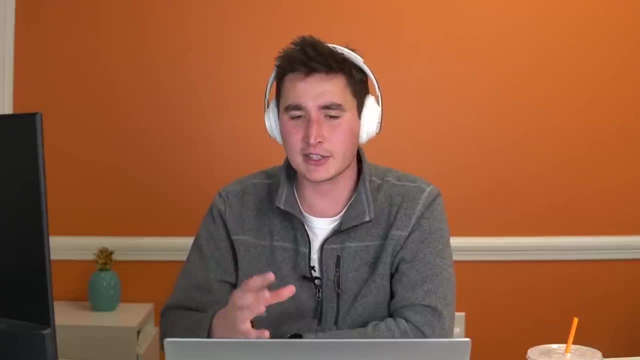 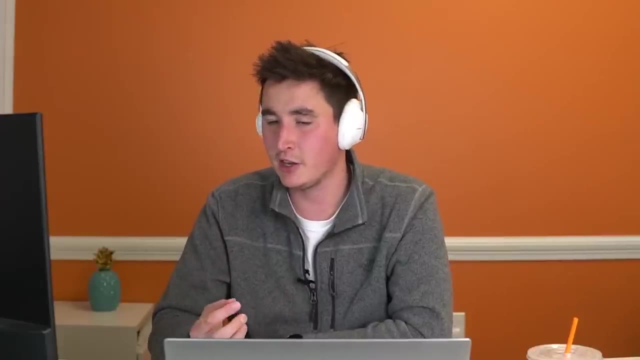 be able to budget properly, So that could cause us problems down the road. It's outside the box, it's different, but it might have been something interesting to bring up just to show you're really thinking about this. Other things, like you know, bots and this kind of came up with the following: 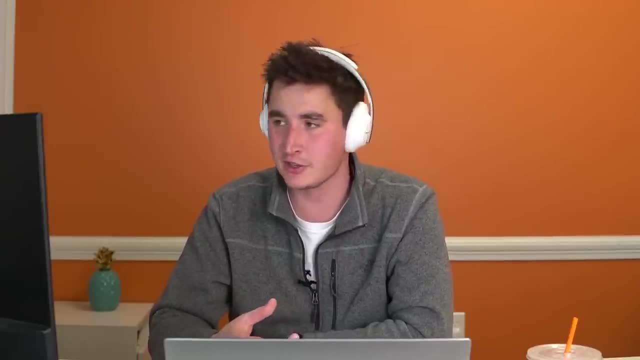 followers and who people follow. So it was kind of indirectly answered this. but like, if bots are liking people's stuff really quickly on, like, let's say, there's a reply and maybe a bot didn't reply to it, maybe a human replied, but that human account had a bot that was. 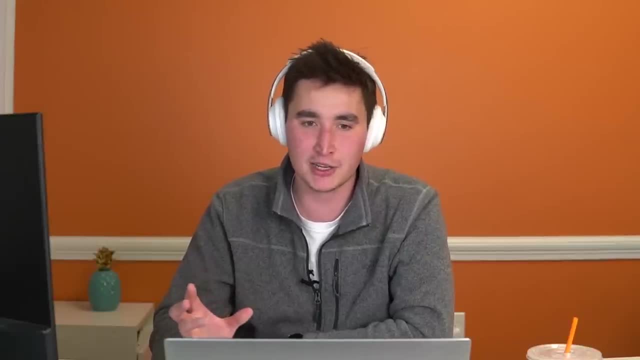 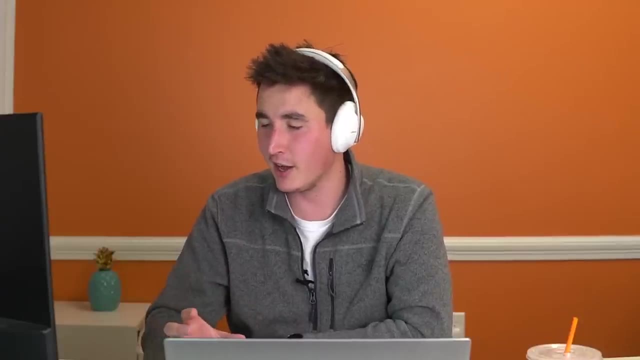 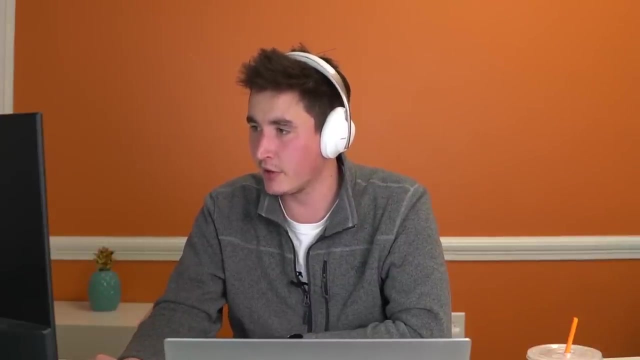 a bunch of bots that immediately liked it. it might give undeserved prominence to that reply, tweet or whatnot as a bot issue. So you know, these are small things I'm poking at, But just interesting things, I guess, to improve further. Yeah, I don't think I have anything else. 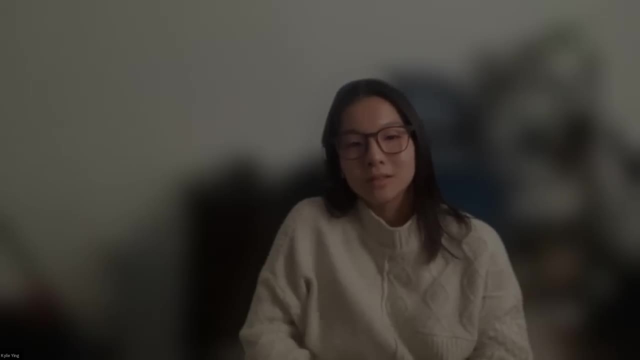 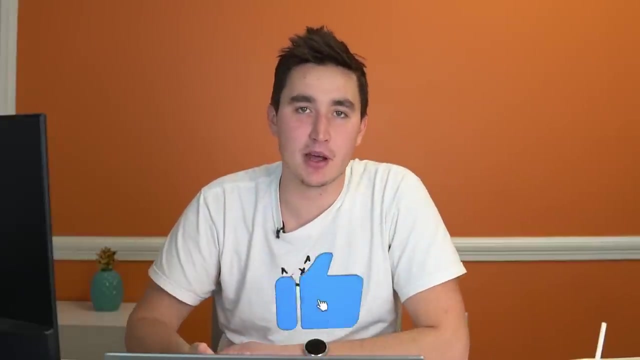 Yeah, I don't have anything either. All right, that's all we're going to cover in this video. If you enjoyed, make sure to throw this video a big thumbs up and also subscribe to not miss any future videos. If you have questions about the job interview process or have feedback on this video, 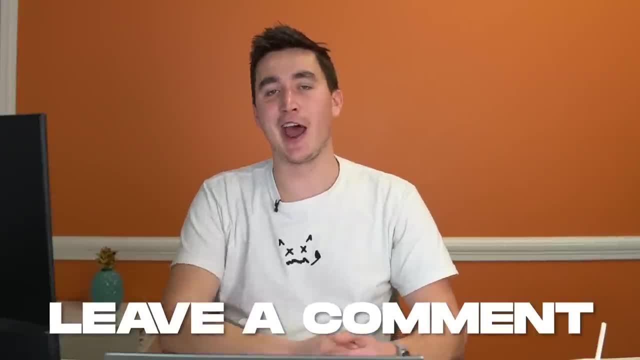 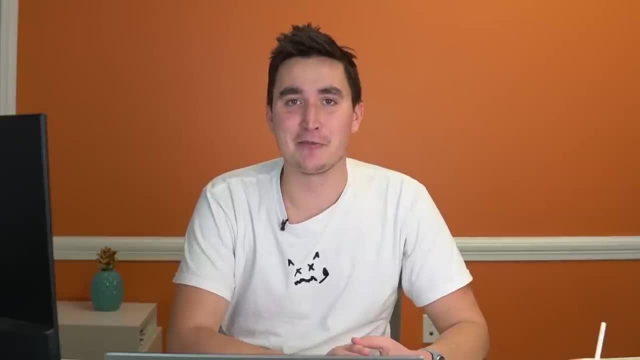 make sure to leave a comment down below. Huge shout out to Kylie for joining and making this video possible. That's all I have for this video. As always, thank you for supporting the channel And until next time.